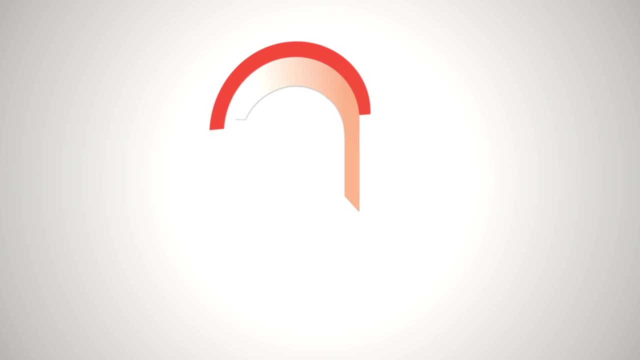 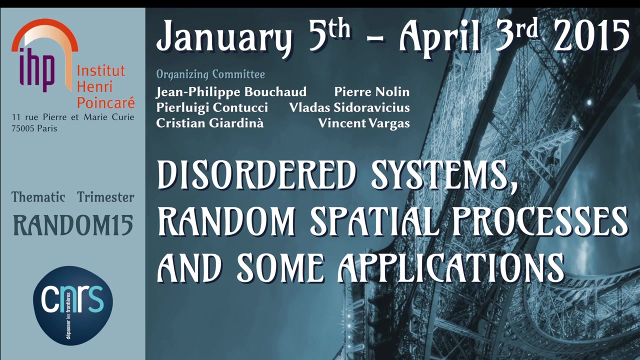 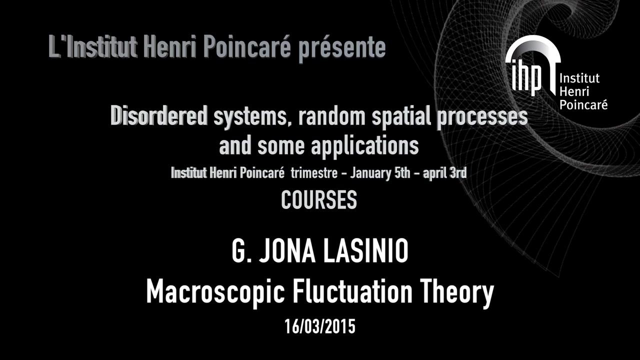 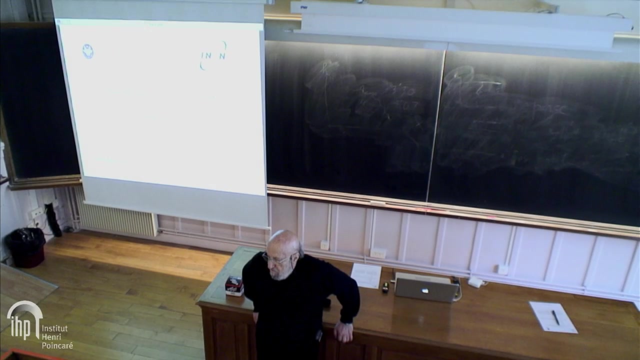 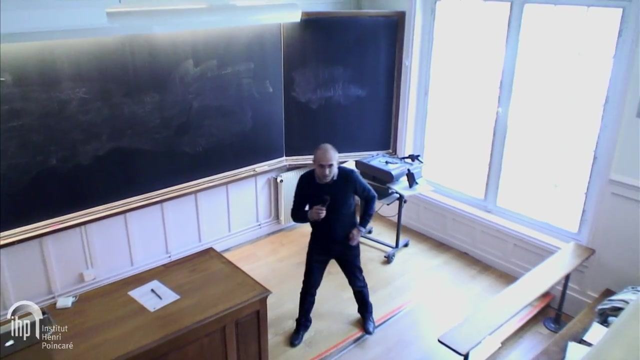 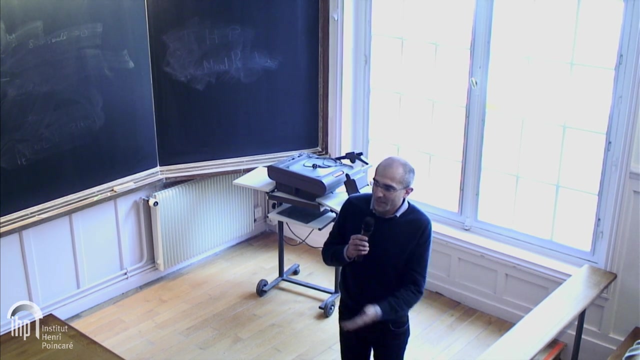 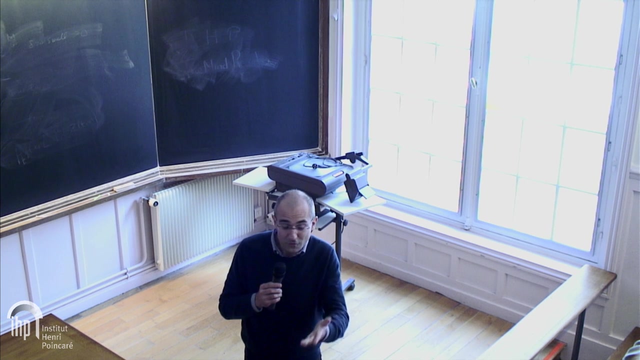 Thank you, Thank you, Okay. so good afternoon everybody. Welcome to this series of lecture by Gianni Ionalasinio. We are extremely happy that, for those of you that were here the past week at the conference, you could already have a glimpse about macroscopic fluctuation theory. 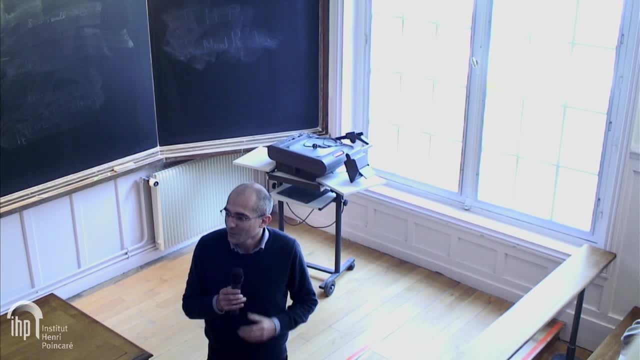 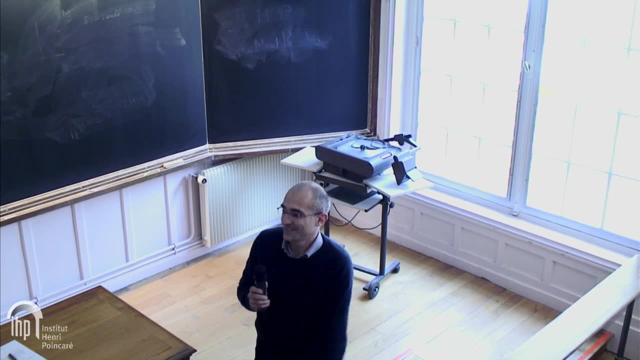 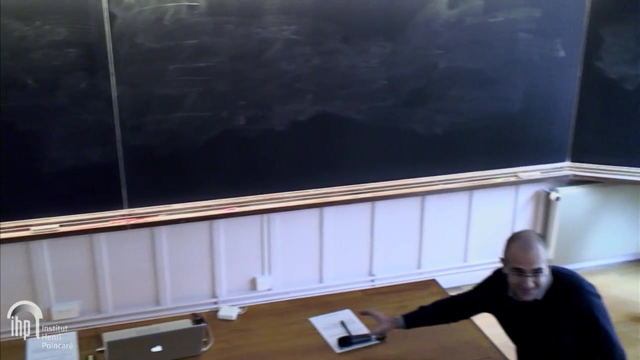 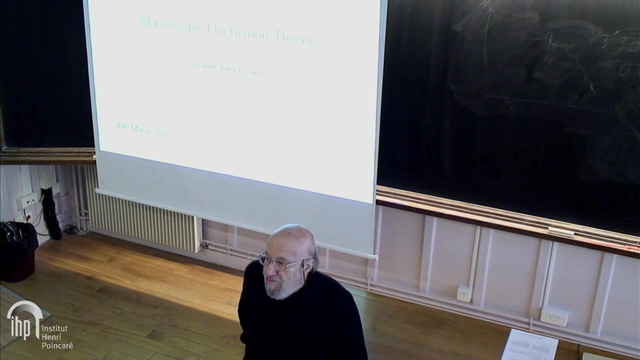 And we are happy that this week we can have an extended presentation. So we thank Gianni for accepting this. Well, thank you. How many of you have you heard my talk last week? Well, it's a majority, So. but 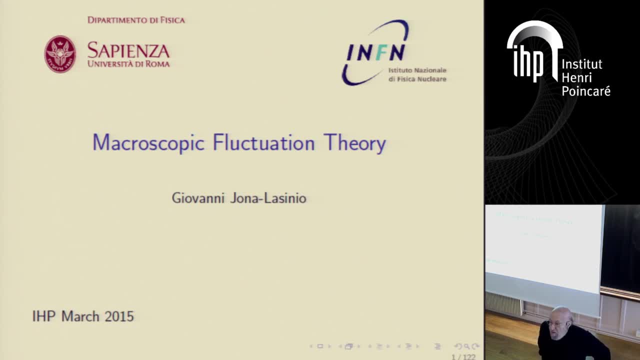 I don't remember, They don't remember. I'm sure you don't remember anything, So you know repetita you want So well, the subject is, if you want is an extended version, But with many more things that I could. 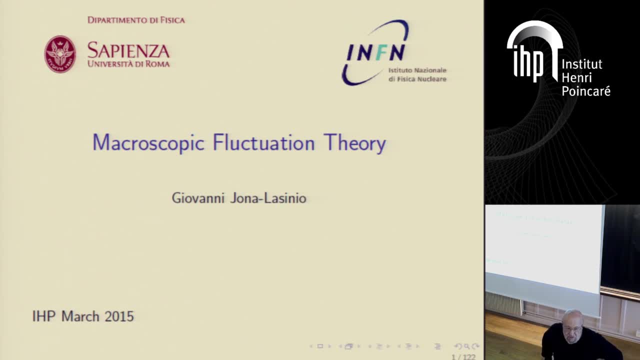 More things that I could not discuss the other day, So, but I think I will start with something historical, Because it's, I mean, to me the history of physics has always been helpful in understanding many why certain ideas came up. 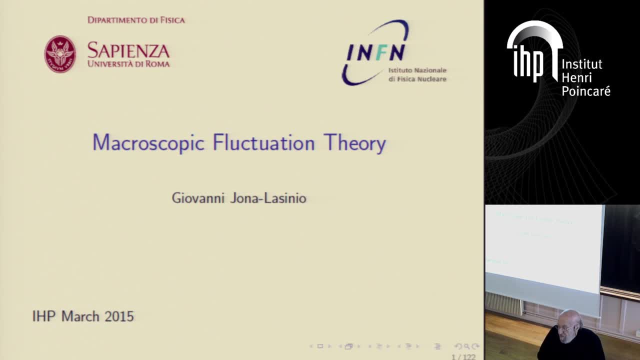 And the story, The story, The story that I'm going to tell, which is the story of large deviations in physics, in statistics and mechanics. well, starts with the work. you can guess by whom? from Einstein. It's a 1910 paper, which is partly correct and partly wrong. 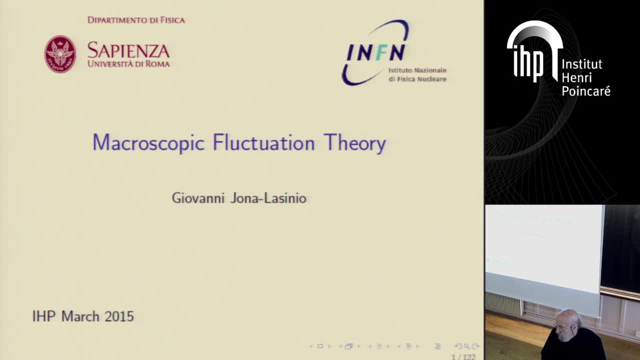 But the path, The path that he wrote, which is of interest to us, is absolutely correct. And what he discusses, fluctuations, macroscopic fluctuations in equilibrium. So let's, I will present you some quotations. Doesn't work? No, It's not. 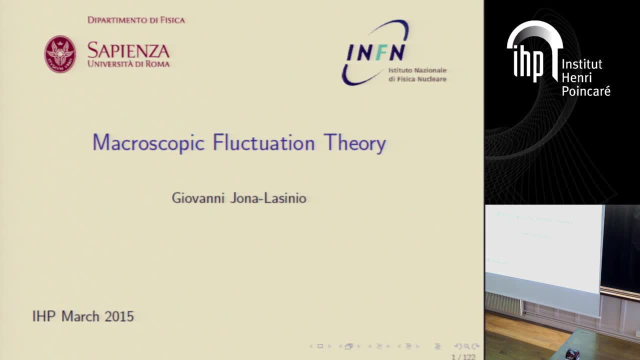 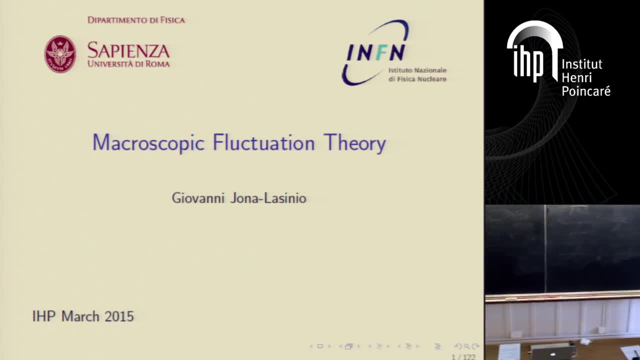 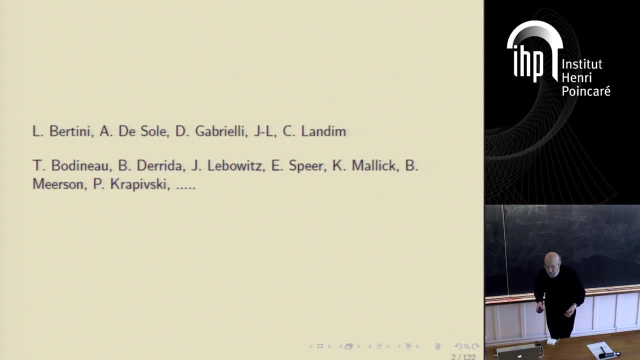 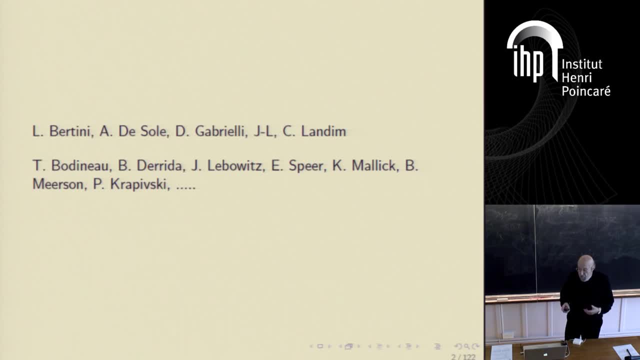 It doesn't matter, I used So, as I said the other day, I'll give you only one. I will give you later a reference, which is a review, and here are some of the people who have contributed to this theory, but the list is much longer, in fact. 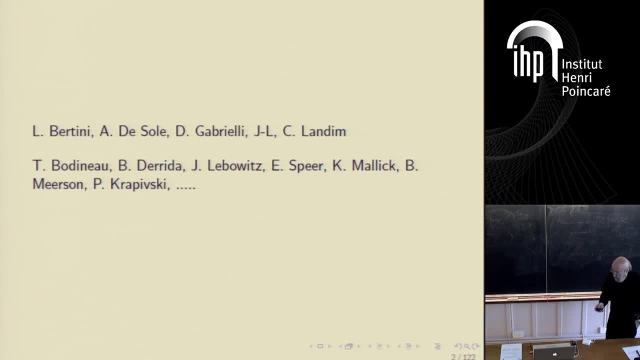 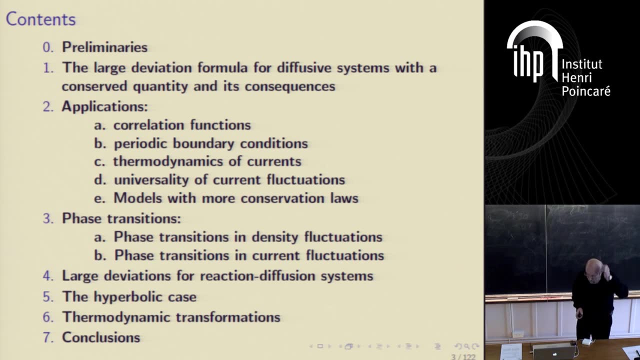 Let me so the what I'm going to discuss. well, here is a kind of summary. you know, during these three lectures, with respect to the other day, there will be several applications that will be treated. so this is, this is a list, and all these things peculiar to non-equilibrium and 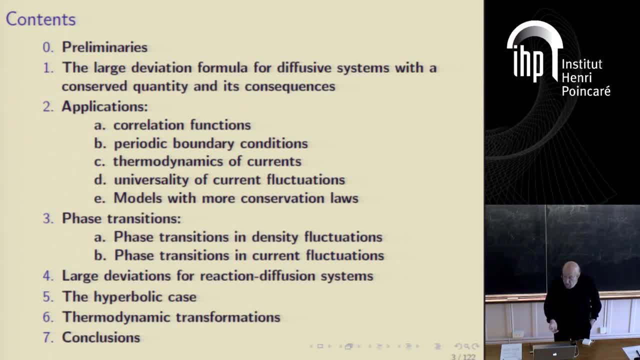 there will be a very interesting topic is the thermodynamics of currents, which the other day I did not discuss at all. then I will discuss phase transitions out of equilibrium, because out of equilibrium some phase transitions which are forbidden at any in equilibrium are possible. and then I 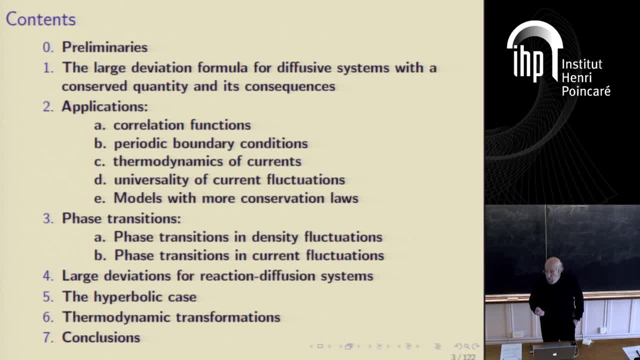 will discuss phase transitions in current fluctuations, that which are peculiar to this new thermodynamic variable, which is the current, and which have a dynamical, current dynamical character in this transition, at these phase transitions, and in some kind is the beginning of a novel chapter. then I will discuss briefly the hyperbolic case and then some more. 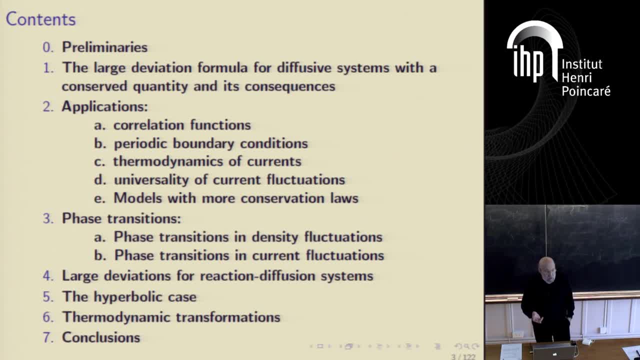 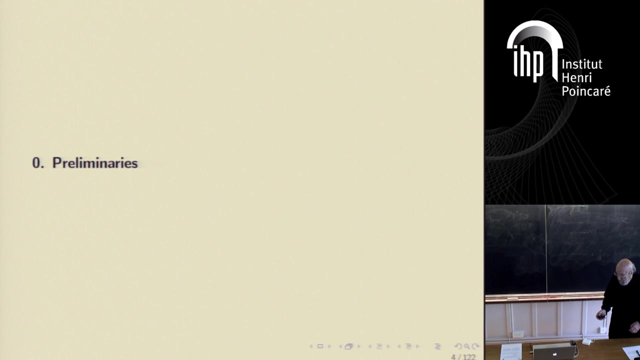 details on thermodynamic transformations with respect to what I discussed the other day and then what some conclusions. usually I don't draw conclusions because it's we are on the way, you don't. you don't know what it works now, thank you. so I don't have to stress that non-equilibrium is. 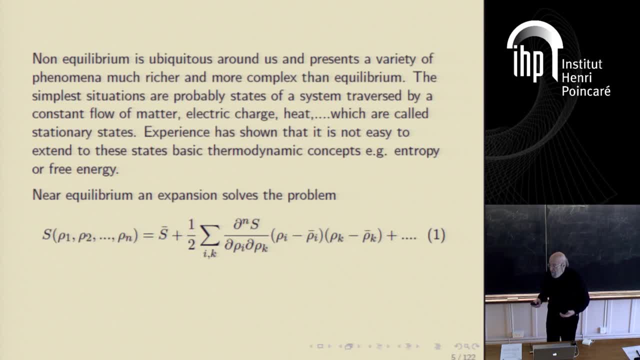 ubiquitous, and especially I mean in all situations in which you have some flow of energy, then are typically non-equilibrium situations and in fact there was a report of the American Commission of Energy some years ago- not so many years ago- that indicated that just the relation with this problem of flows of energies in the mentioned non 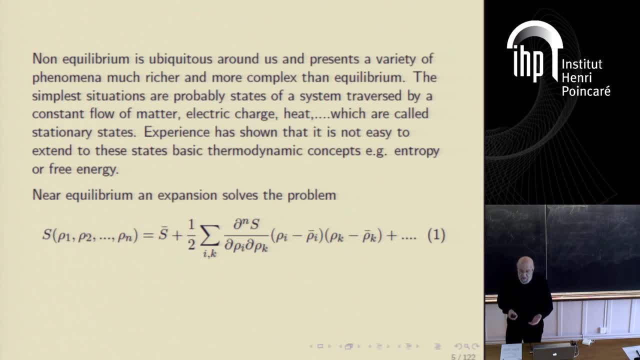 equilibrium physics as the really the important subject for the future. so we, So you see up to the first theory of non-equilibrium. I usually start from Sager, I mean macroscopic theory of non-equilibrium, and his idea was that his theory was near equilibrium. so he, 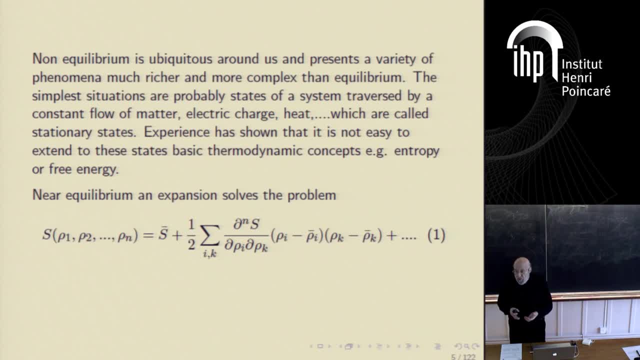 started making power series, development of the entropy in terms of the thermodynamic variables and of course you get the first time. you get is the second term, because the entropy is always a maximum, and then that was his way, so in that case you could reduce. 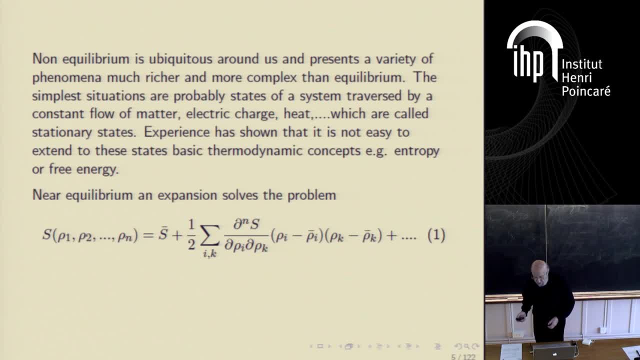 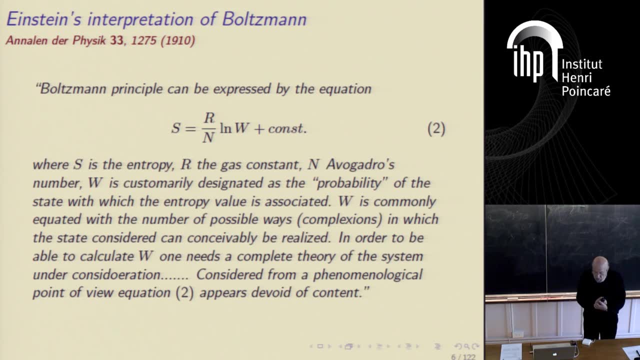 the non-equilibrium to equilibrium, just by this expression. But let me start from the Einstein interpretation of Boltzmann. You see, this is what he calls the Boltzmann principle. This is just quoted from his paper, which is translated in the book. there are several. 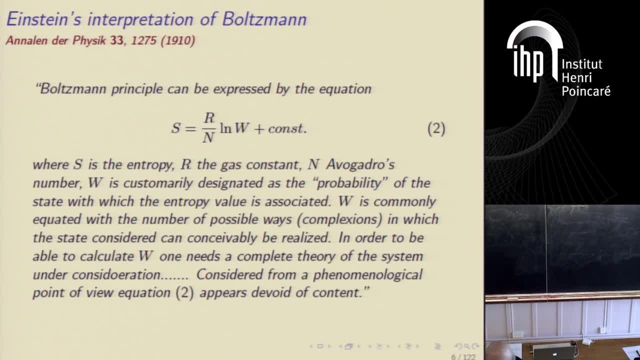 books with Einstein papers translated, So it's an official translation, if you want. So this is the famous relationship of Boltzmann which connects the entropy of an equilibrium state to the logarithmic. well, this is not the probability which is normalized to one. 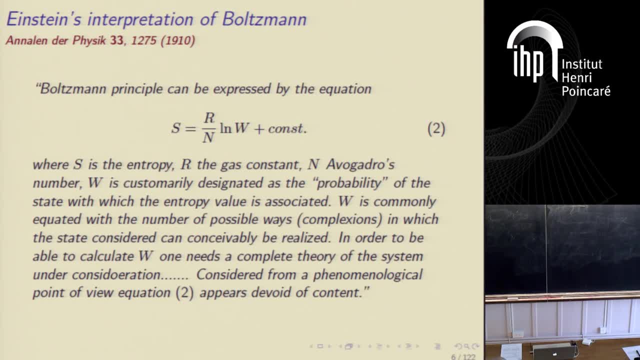 but is the number of states which are compatible with a certain choice of thermodynamic variables. So So yeah, in this formula you have a large number, which is Avogadro's number. This is called usually thermodynamic probability, but it's not a normalized one. 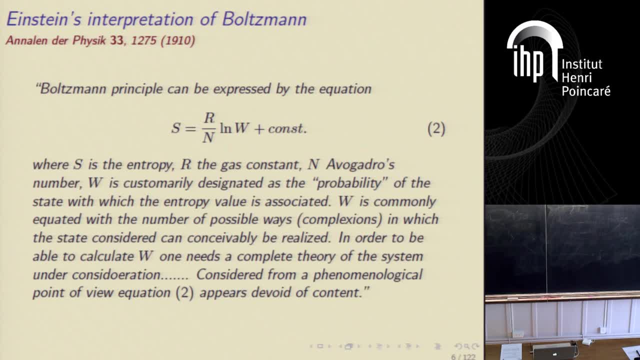 They were. they had the possible ways, the possible microscopic configurations which were compatible with the choice of thermodynamic variables, were called complexions. So And so these are the ways in which certain microscopic states can be realized microscopically. But what he objected? that this formula to calculate the number of states of the system. 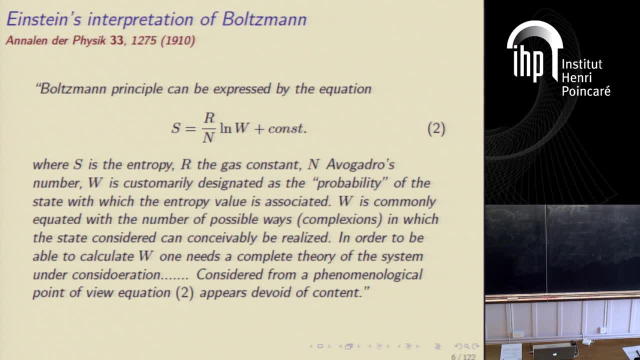 compatible with a certain choice of thermodynamic variable. you require the detailed microscopic theory, which was different for every system. So this formula for him, I mean, Einstein was very, always very, gave much importance to the fact that things that must be measurable. 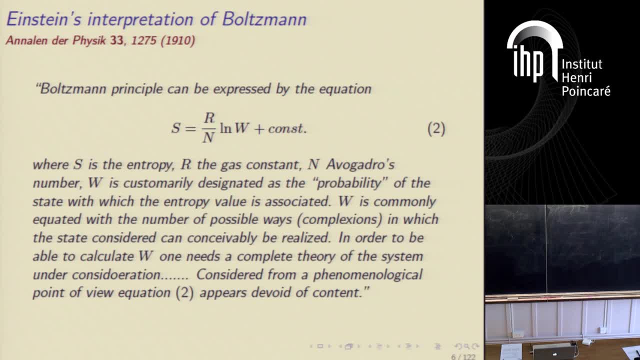 And he said so this he didn't like at all this thing. In fact he says: consider it from a nomological point of view. equation two appears devoid of content. So it went quite. his opinion was quite wrong. So he said: consider it from a nomological point of view, equation two appears devoid. 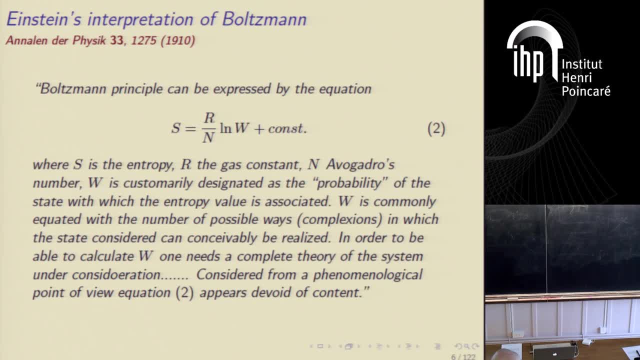 of content. So it went quite. his opinion was quite wrong. So he said: consider it from a nomological point of view. equation two appears devoid of content. So he says: consider it from a nomological point of view. equation two appears devoid. 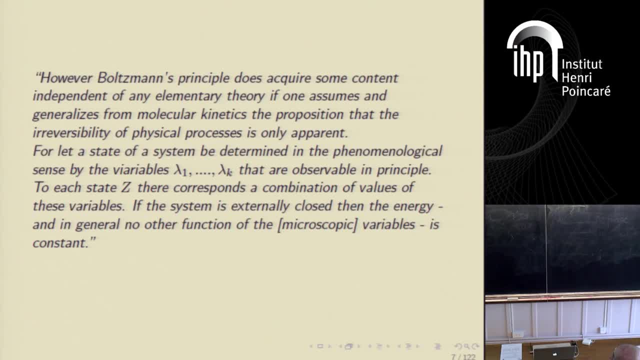 of content. So he says: consider it from a nomological point of view. equation two appears devoid of content. So it went quite. his opinion was quite. this situation seems quite, quite sharp. And now this still quote from Einstein: 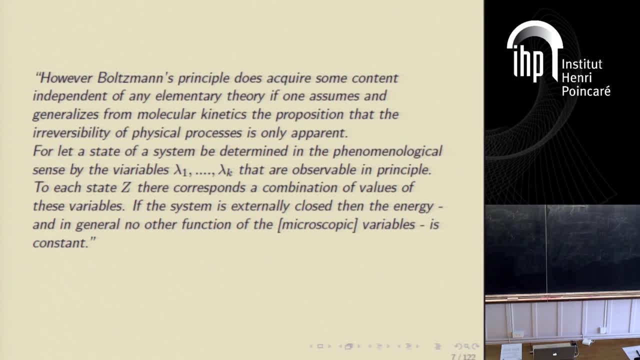 However he saysolan principle quite some content If one assume generalize from molecular kinetics the proposition that the irreversibility of physical process is hump in. So what in 19 is God's theory. So experiment, He said, we will replace it with. here you write here, you put it here that it's the 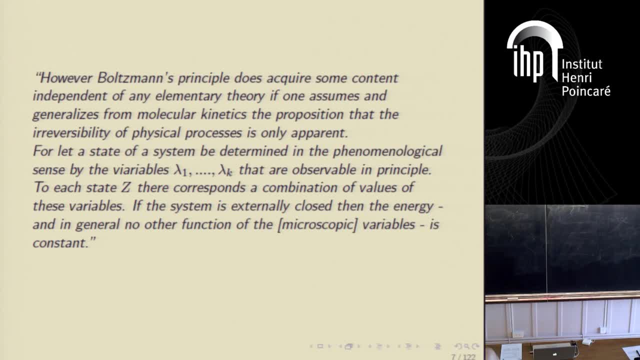 maybe thewydd is like saying There's no way that you can use all the words you find in the Jacquard model. So, and the way he thinks he can give meaning, phenomenological meaning, to a macroscopic state is, in principle, because there's always 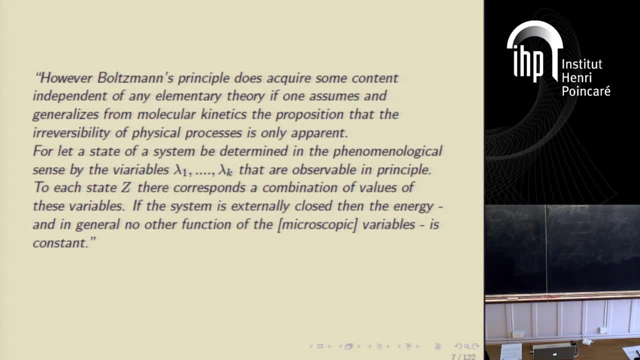 a question of principle is to measure how much time the system spends in a given macroscopic state, And this is something that, in principle, can be measured, Even if these times are so small that practically. but anyway, there is a connection with the phenomenology. 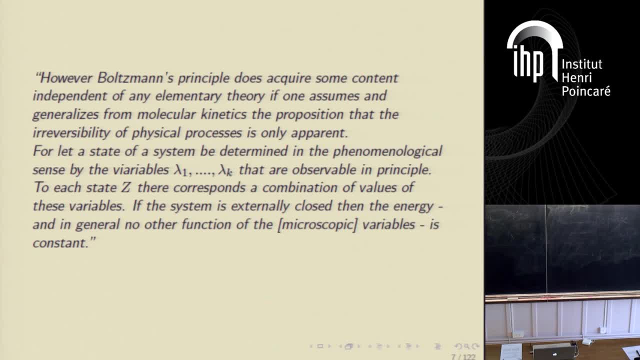 So and then so he considered a system, he considers a system where, which is in a state that characterizes this lambda one, lambda k, are macroscopic variables, So to each state the corresponding value of this variable if the system is externally closed. 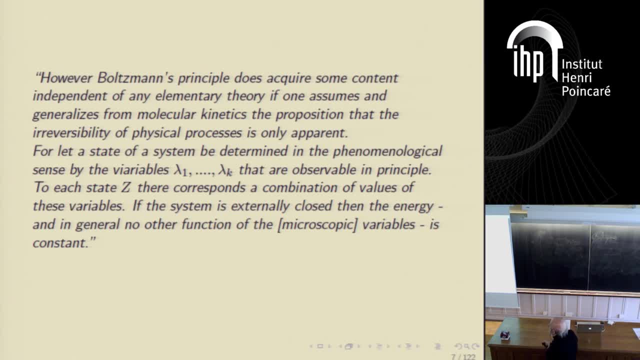 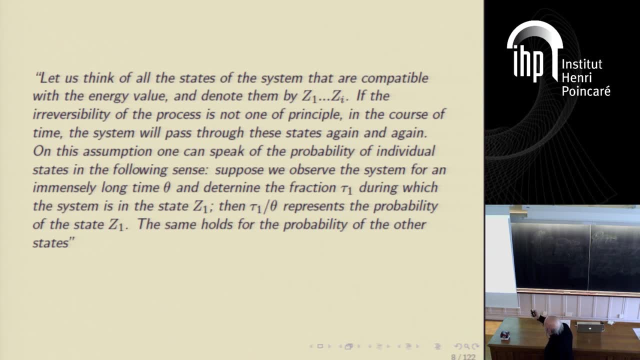 so it's an isolated system. the energy is the only constant. Now, that is the way he gives meaning to the probabilities. He considered different states. So he says: if irreversibility is only apparent, the system will go through all these states. 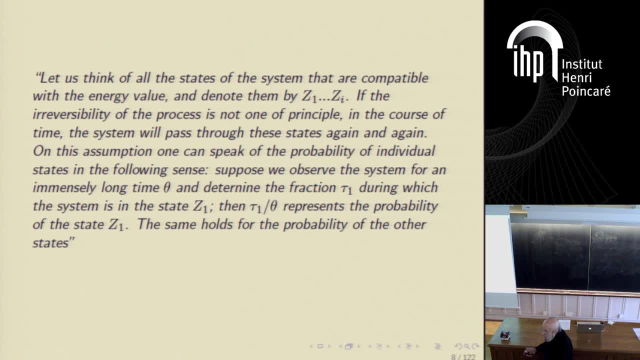 during its evolution. This is the ergodic hypothesis And in the way it was formulated at that time, I mean. And then the idea is to take this: the probabilities, you see you get the, so this tau over represent the probability. 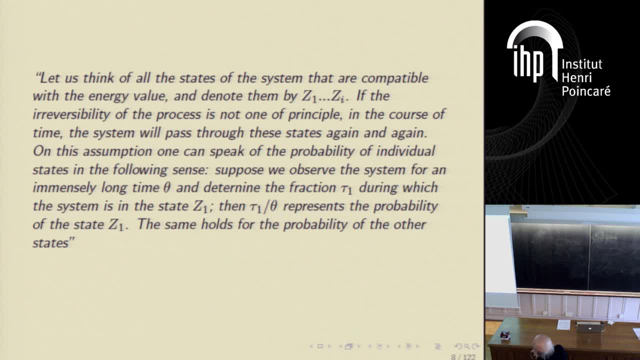 and the probability. I mean you observe the system over a large time and then the amount of time it spends in the state that you are interested in over the long time represent the probability of the state. So that was his way out to give phenomenological meaning. 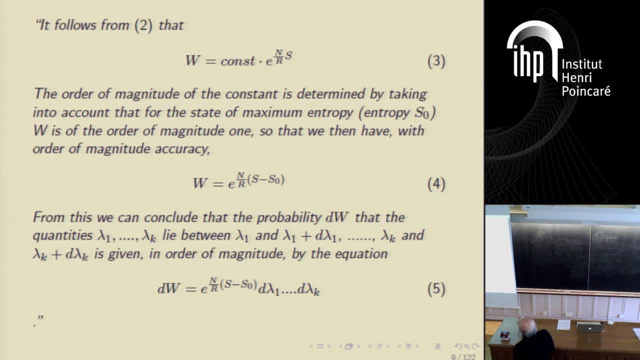 to this Boltzmann formula. Then at this point he inverts the. I don't know how many of you have gone through the history of the subject. so, and I think it's of some interest, because what in fact? the macroscopic fluctuation theory. 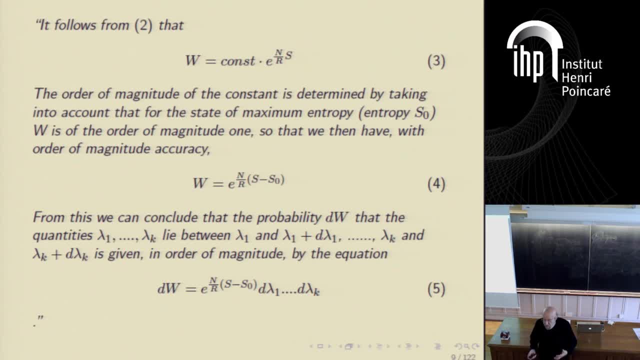 methodologically. that we have realized much later. but there's something very similar to what Einstein did, as we shall see. Okay, So inverting Boltzmann formula, we can extract this thermodynamic probability in terms of the entropy, Then that one. you start from the state of maximum entropy. 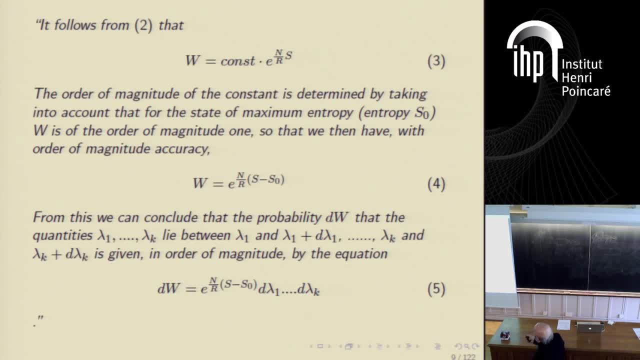 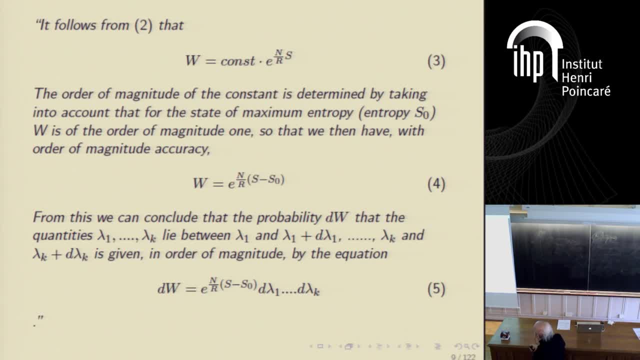 and so he writes this formula for the fluctuation, so for the seconds, of the macroscopic variables, for the distribution, I mean for the probability distribution of the macroscopic variables: lambda one lambda k, lambda one, lambda k. And of course this S minus a zero is negative. 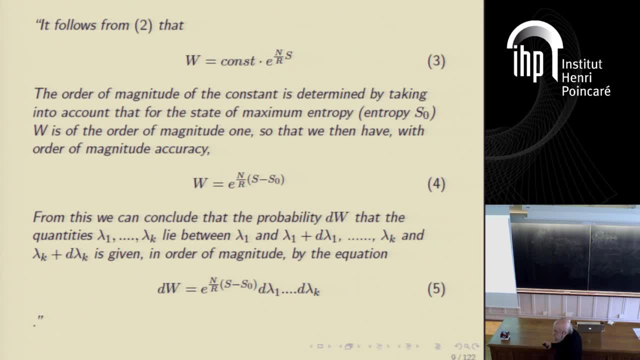 because S zero is maximum entropy. And you see, it's, it's a typical, you already see emerging the large deviation situation because you have in the exponent is Avogadro's number, which is a very large number. 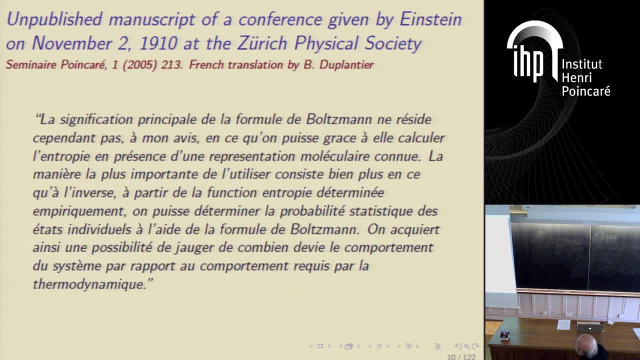 OK, His position is also clarified in an interesting paper which is not included in Einstein's works, but it was related here at the Institute, here at the Pointe Carré Institute in 2005,, when there was the Year of Relativity. 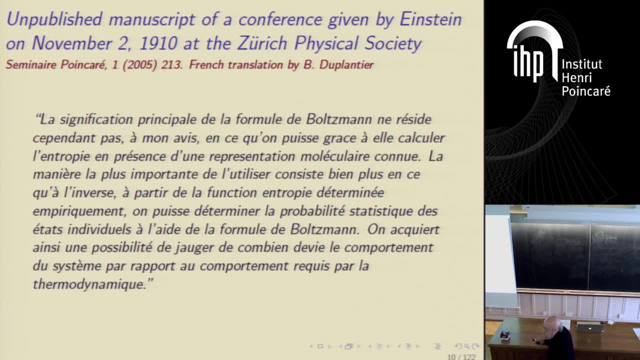 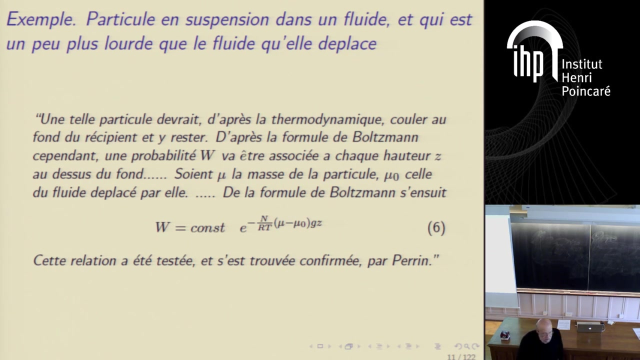 It was translated into French by Bertrand Duplantier. Here he emphasizes again that in a slightly different way, the fact that the Boltzmann formula is not a phenomenological formula And but, what is interesting, the way he used it, because he combined this formula. 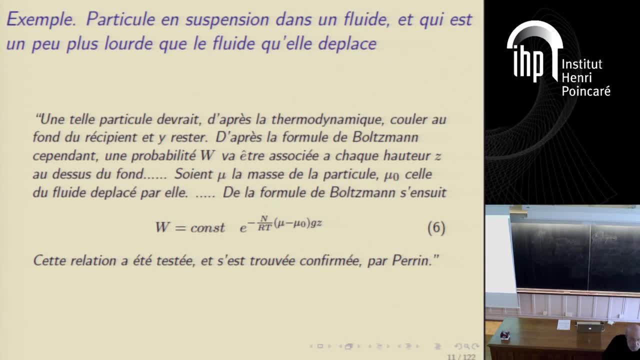 with what were macroscopic hydrodynamic expressions at that time, in particularly where Stokes' law for the resistance of a sphere going down in a fluid OK. So in that case you see, And here you see, you have the variation of entropy. 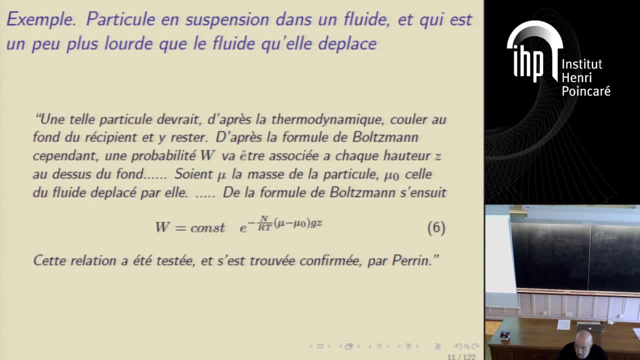 But think of the variation of the free energy, And then that is the work, the minimal work that you need to do. And so you see, here you have. mu is the mass, the sphere, Mu 0 is the mass of the displaced liquid. 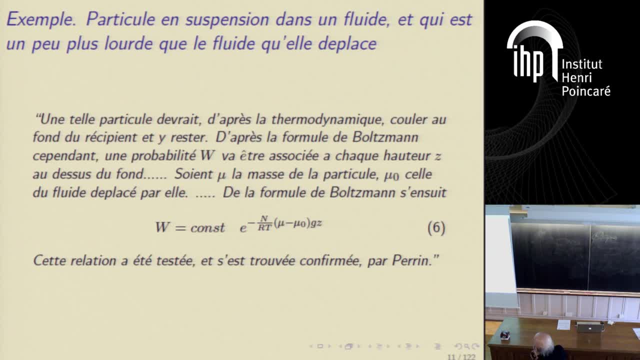 So is the Archimedes, And so that was the formula for the fluctuations. So you have a sphere which lies on the bottom of a container, And then it fluctuates and makes jumps due to thermal fluctuations. So this was the formula for this thermal. 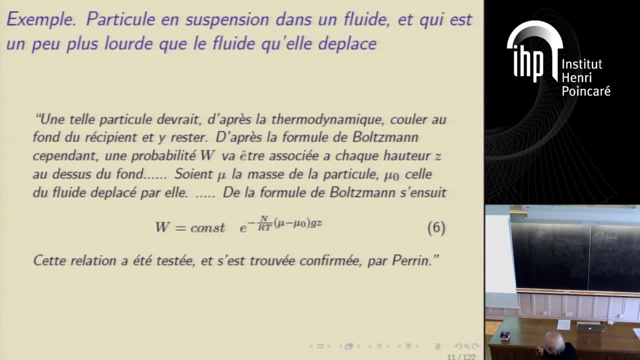 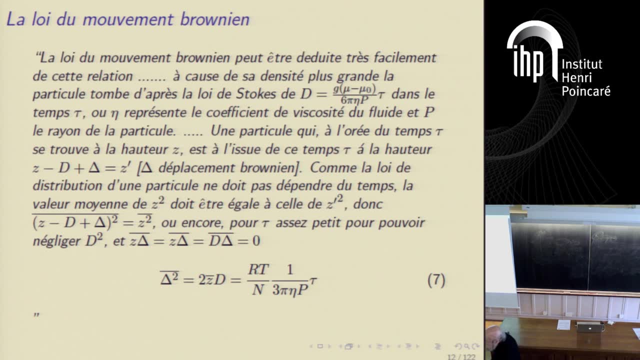 Fluctuation, And this was experimentally verified. But then he went on. He derived from this formula the law of Brownian motion in a thermodynamic way. You see the Stokes formula. So here you have that. It's a formula for the velocity of a. 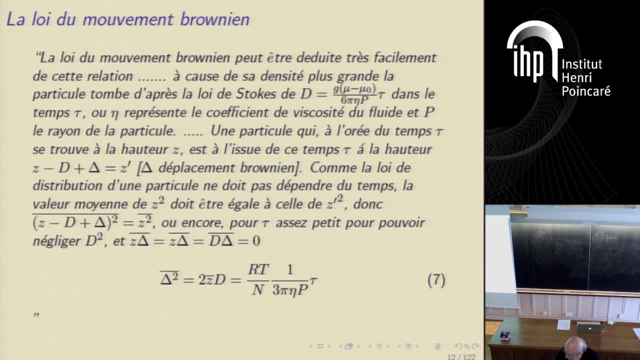 Mm, Mm, Mm, Mm, Of this body in a fluid. So this 1 over 6 pi, eta, and pi is the radius of the particle times, tau, which is a time. So this is the space which is being 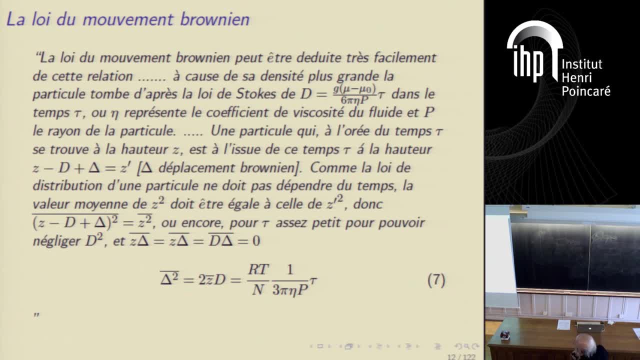 Mm, Mm, Mm, Mm, Mm, Mm, Mm. OK Yeah, According to this Stokes law, which is the interval of space which is covered by the particle, this is potential. So it goes. delta: the Brownian displacement. 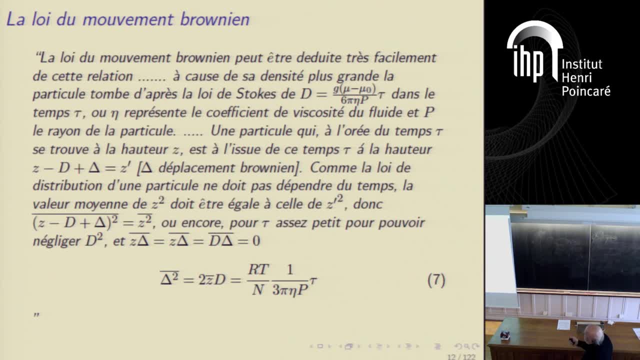 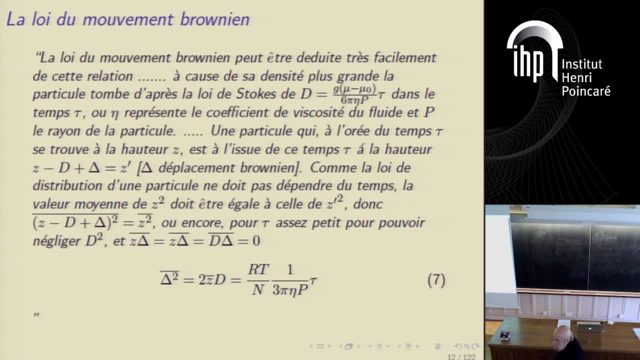 is proportional to the time instead of the time squared, And this follow- Well, we should see that as an exercise later- that from the general formula which I discussed the other day for fluctuation out of equilibrium we shall get the same result as Einstein in a different way. 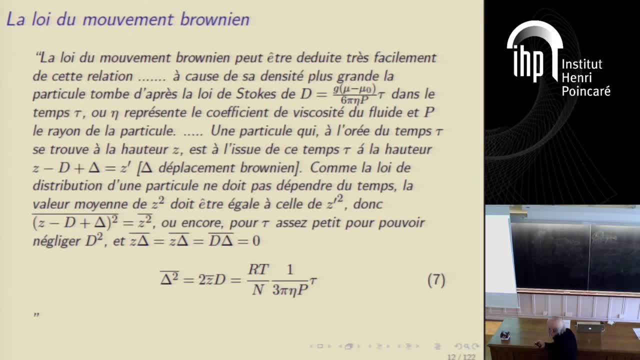 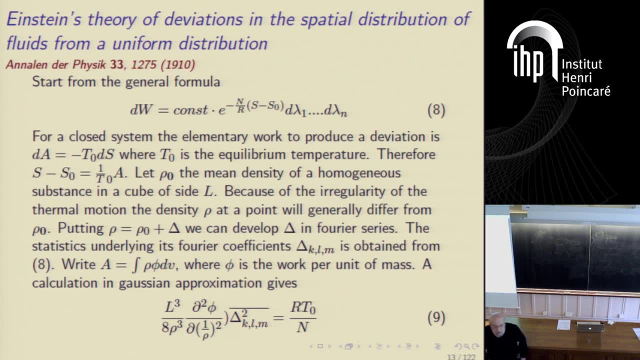 but which is, as an exercise, is quite amusing, OK. So then, what he did with this formula was the following: that he wanted to interpret what is called the opalescence When you throw some light on a fluid, due to the thermodynamic fluctuations. 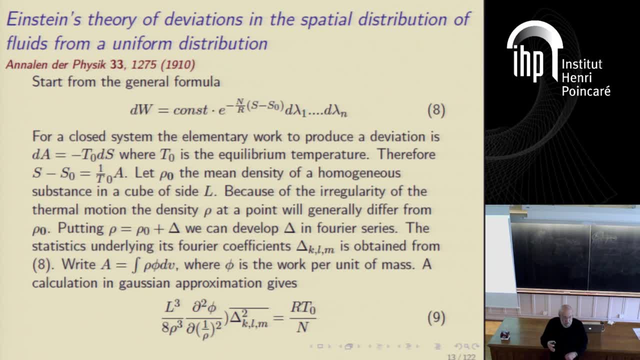 then you see some kind of the light is not clean, You get some opalescence, which he attributed to the fluctuations, And so he did this calculation. I mean, if you want to know more, you should go to and see this paper. 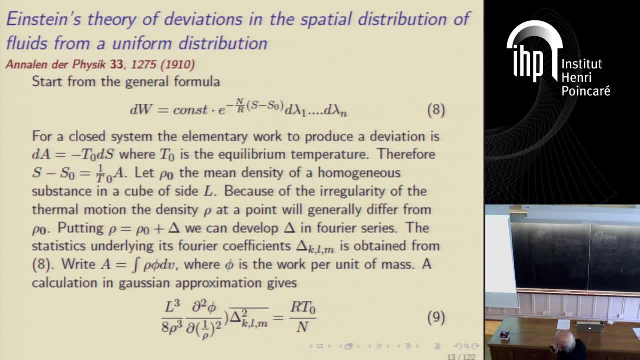 And he made the development of this fluctuation into Fourier series And then he calculated all the average within a Gaussian approximation of the averages of the Fourier components and found this formula: This second derivative of the work, with respect here to the inverse density, is essentially 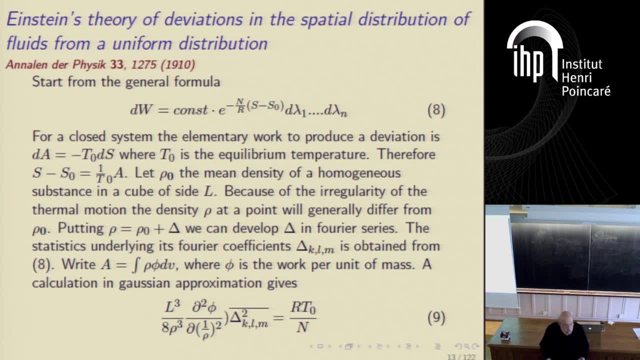 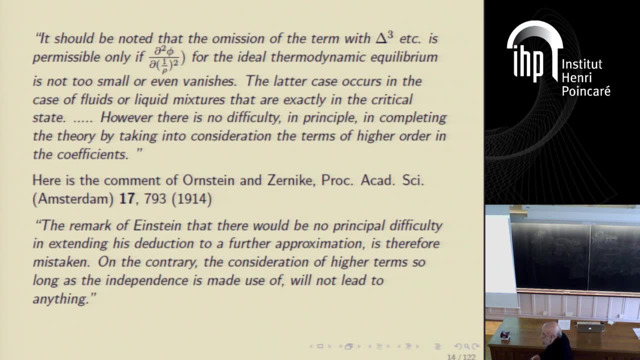 a kind of compression coefficient. OK, But then what happened? He wanted to apply this also at the critical point. At the critical point, we know that there are long range correlations, And he didn't realize that. So he said simply: we have to go to a further term. 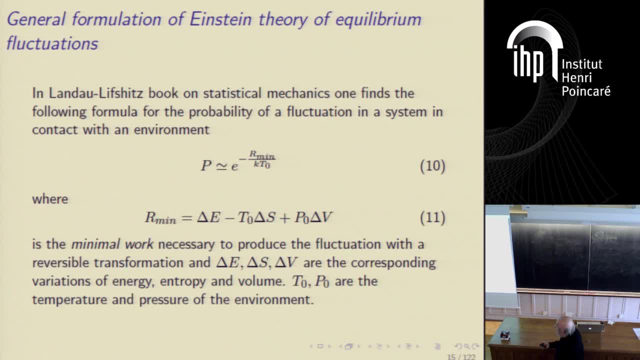 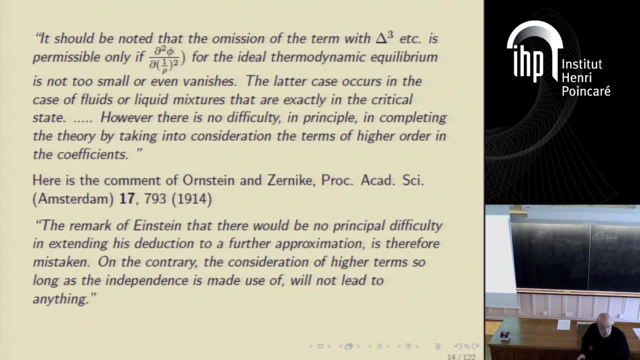 in the expansion And this provoked an angry reaction, The reaction from Holstein-Zernicke, who proposed the first correct theory. at the critical point he says that his deduction is mistaken. On the contrary, consideration of a term so long as the independence is made useful. 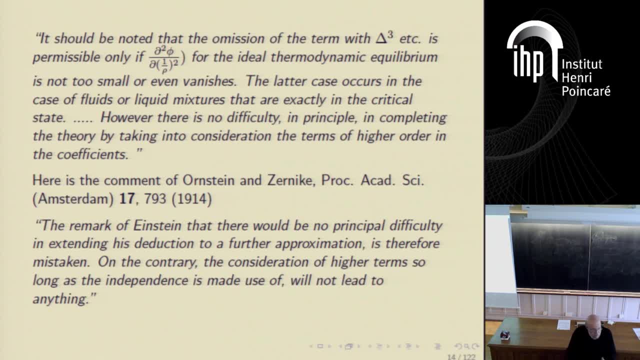 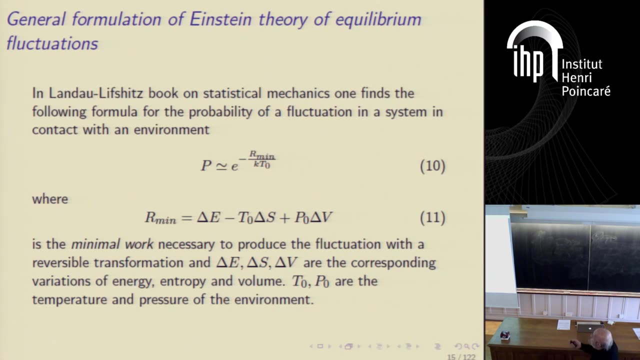 will not lead to anything. So I mean, at the time discussions were quite I don't know, I don't know, I don't know. People had very strong opinions at that time. OK, So if you go to the book of Landau-Liefritz, 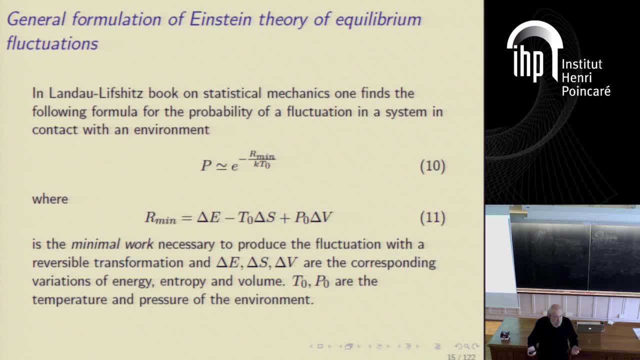 you find, because Einstein considered an isolated system. But for the general case in which the system is not isolated, there is this formula in Landau-Liefritz: And you see that here this r is the minimum, This r is the final work. 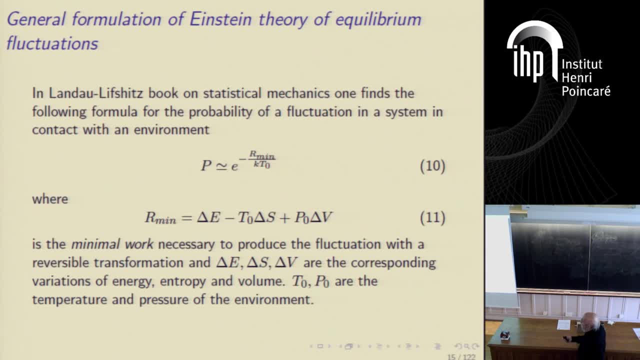 And here it's connected with the variation of energy, of the system of entropy and of volume, if you have, And t0 and p0 are the environment temperature and the position pressure, sorry, OK, So if you want, 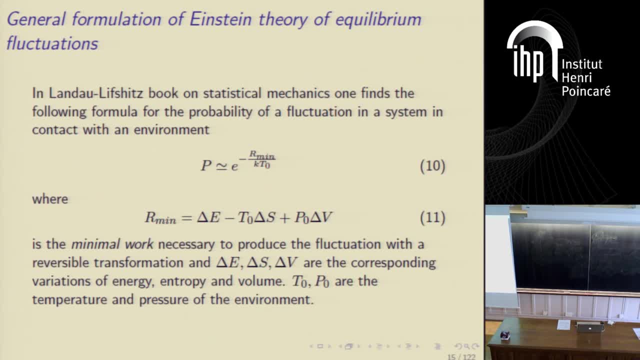 Yeah, Huh, Well, I mean Yeah, Yeah, Yeah. Well, I mean this gives potential this expression. So I mean heat is hidden here in the variation of entropy. So this must be calculated along a reversible transformation. 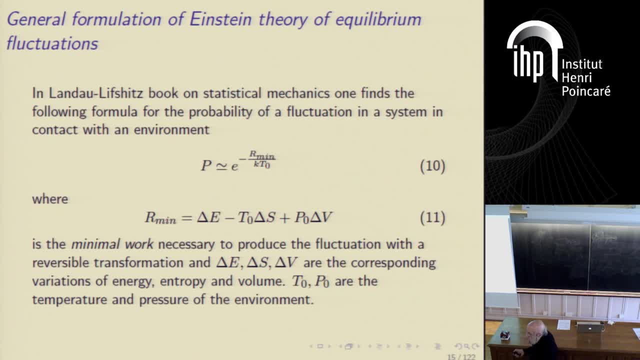 always. what is the difference between heat and work? Well, I think well, in analyzing delta E and delta S, you will differentiate between heat and work. I mean, the work part is this one, if you have the system. 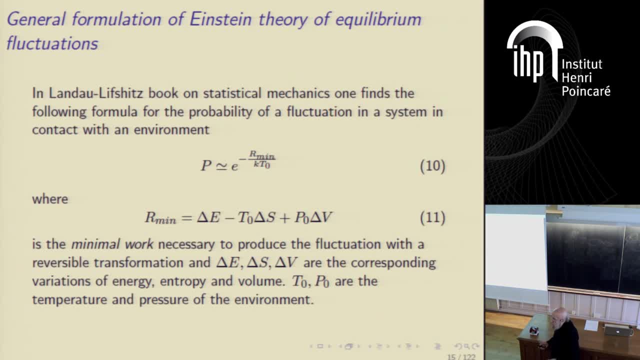 in a cocktail. No, this is the probability of a fluctuation, But the interesting thing is that this can be. this probability can be calculated in terms of thermodynamic functionals of the system at equilibrium. It's clear when you go seriously out of equilibrium. 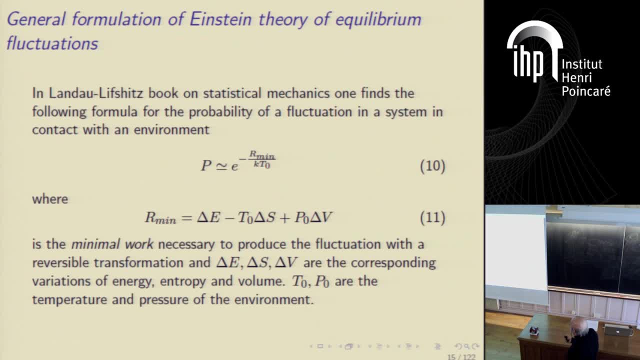 you see, the environment appears only through these two parameters, the external temperature and the pressure. But when you go far from equilibrium, you cannot expect such a simple expression, Because you don't know what are the thermodynamic potentials out of equilibrium. So that is. 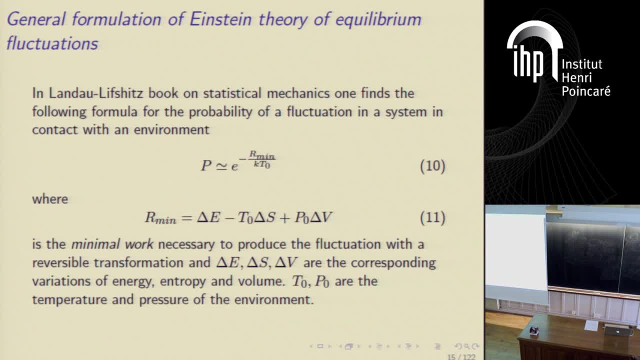 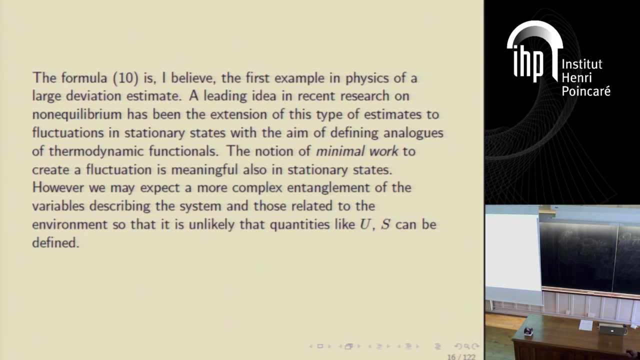 Anyway, you see, What I understood much later with respect to the beginning of our work, was that also Einstein used this combination of a large deviation formula with hydrodynamic expression, like the Stokes formula. So I believe that in fact this is the first example in physics. 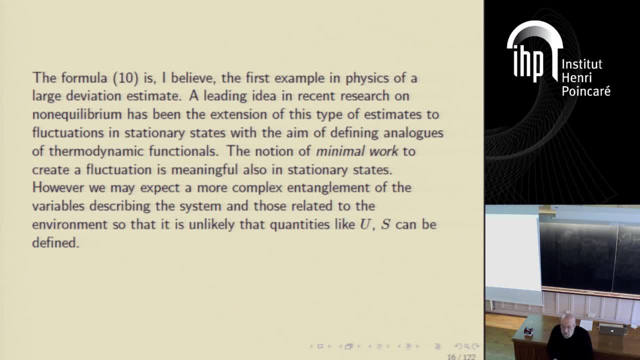 Of use of large deviations. So by large deviation we mean probabilities that are exponentially small, And there is some big parameter, large parameter in front of the exponent And in this case it's Avogadro's number, which is hidden in the Boltzmann constant usually. 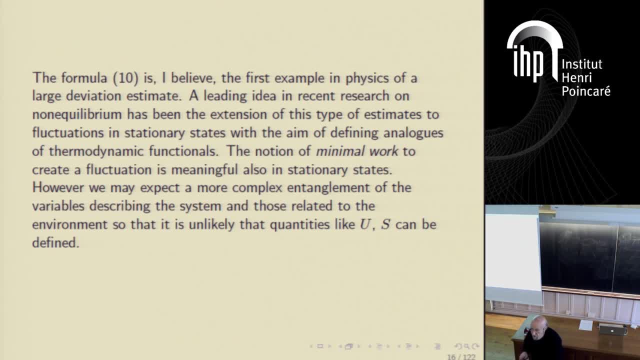 The Boltzmann constant is the ratio. It's the ratio of the gas constant over Avogadro's number. So well, I hope I gave you some idea And if you are interested, you just go to this series of books with Einstein works. 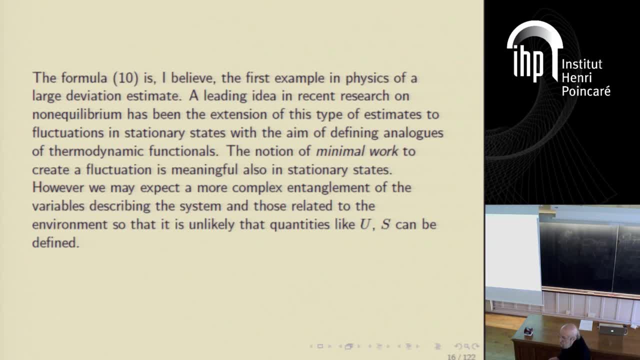 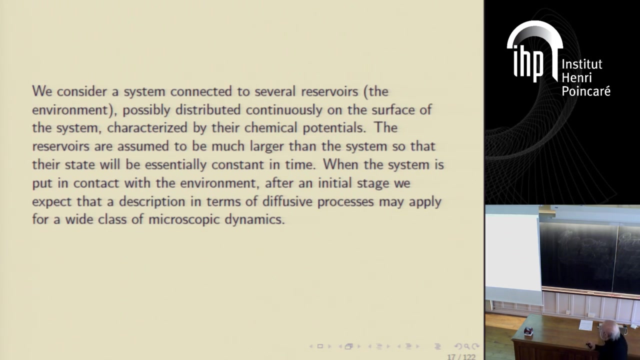 and you will find this paper, Not the conference at the Zurich Physical Society, which you've found either in the book that the Institute for browsing prepared years ago, Or then it has been published in some volume, or something like this. OK, now the situation we consider is: 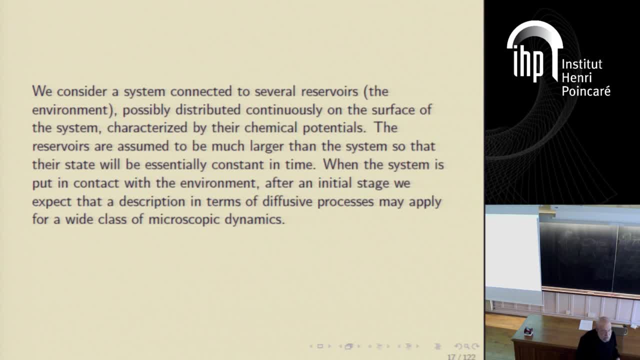 our system, which is connected to several reservoirs, so maybe thermostats, Thymonor, reservoirs with different chemical potentials, and you expect that once you have connected, there will be some initial stage in which the currents will be flowing through the system in some 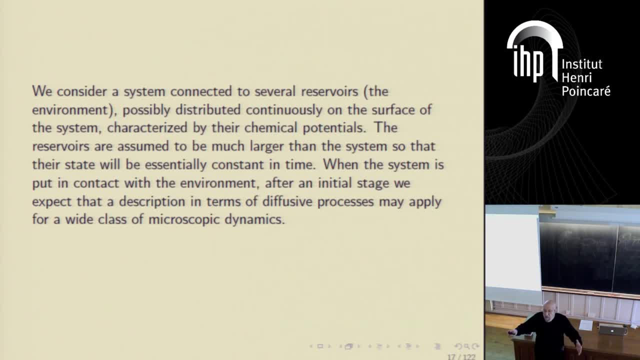 wild way. but at some point, since the reservoirs are supposed to be much larger than the system, the system will set into a stationary state, and that is the approximation even in Hamiltonian system. so there will be some diffusive regime at some point which will last for a rather long. 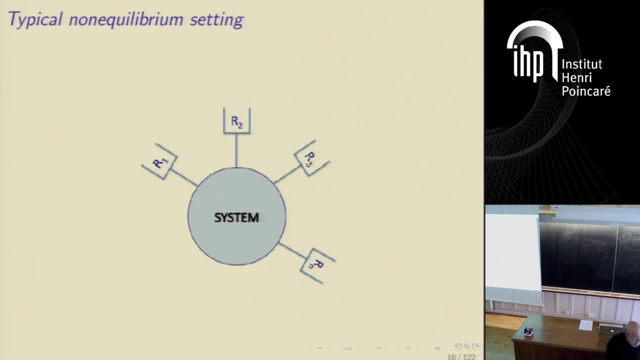 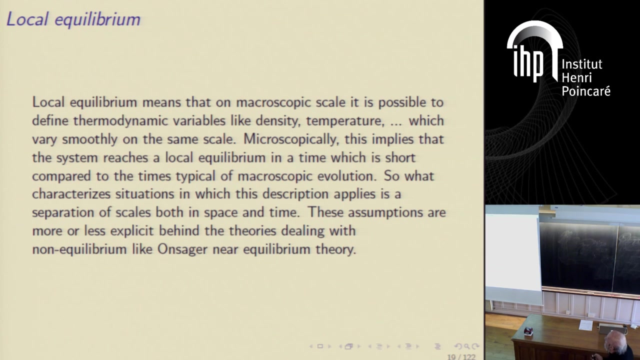 time. so this is the picture, so you have the system connected with. I'm laughing because Cristina Toninelli always teases me about showing this scheme. so now, in order to have the possibility of a hydrodynamic description, you need something like local equilibrium- that I also discussed the other day. 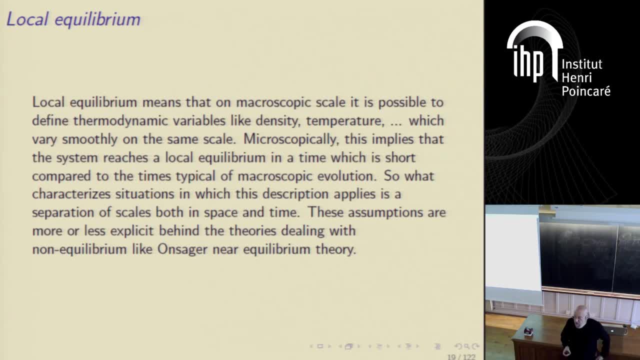 and so the idea is the following: that even, for example, if you have a system that is connected to reservoirs, which are very different parameters, you assume that locally, in a small region, on the macroscopic scale, the system doesn't differ too much from equilibrium by adding a large number. 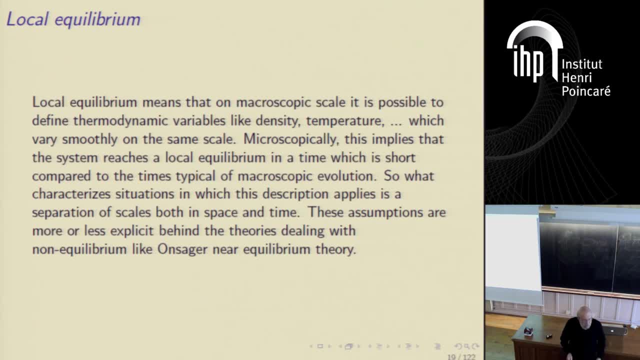 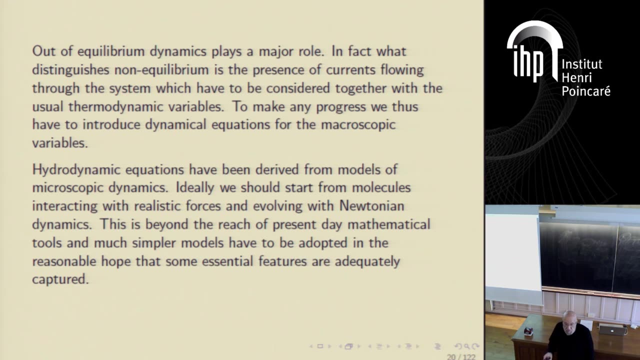 of small deviations from equilibrium, you reach a large situation far from equilibrium. so well, of course, once you are out of equilibrium, dynamics is important, and then we have to cope in some way with this. but we are interested in the macroscopic theory. so you see, in principle, what we would like to do is to calculate. 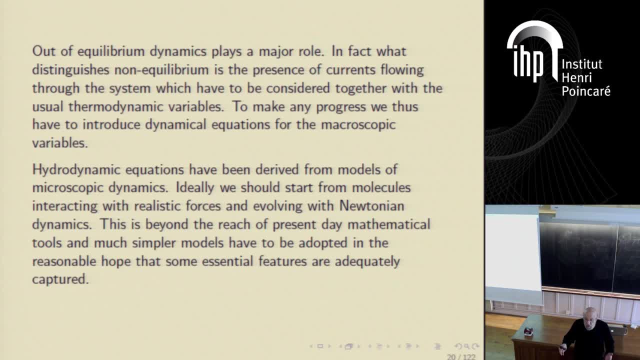 the macroscopic distribution in a stationary state and then use it to calculate large deviations. now, this is usually very difficult. there are only very few cases where you really are able to calculate the the macroscopic distribution. one case was the simple exclusion, the metric simple exclusion. 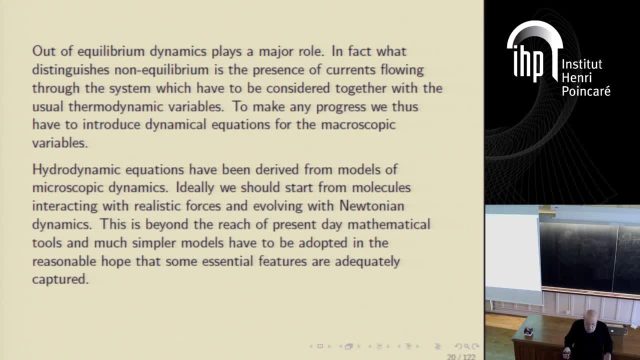 and it was calculated as a simple exclusion long ago by Derrida Leibovitz and Speer by solving the model by brute force if you want, but then we shall see. the another possibility is to try to arrive directly at the probability for the fluctuations of 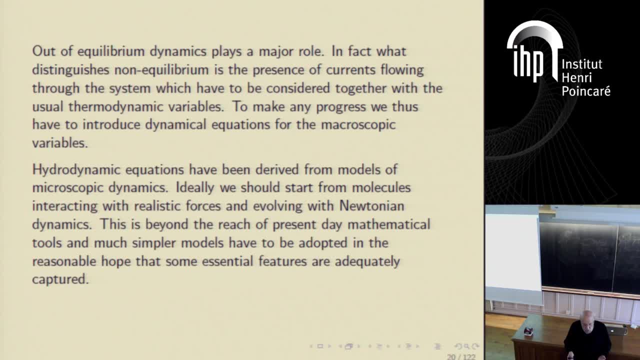 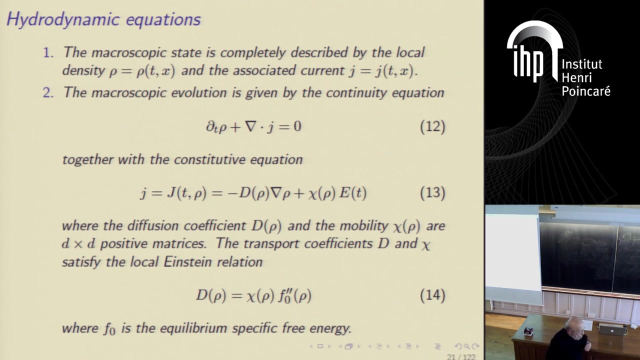 macroscopic observables without without having to calculate this macroscopic distribution, and that is the the way I will discuss this is the macroscopic fluctuation theory. ok, so well, this is clear. what is here? so we assume androdynamic equations. these are usually assumed in. 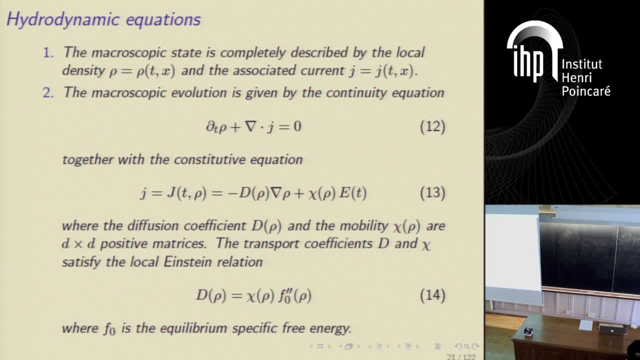 for example, there is an old thermodynamic book by Fitts in the beginning of the sixties where he discusses non-equilibrium thermodynamics and he discusses quite clearly the assumptions which are made and in particular, which are the assumed hydrodynamic equations. and then, of course, he discusses: 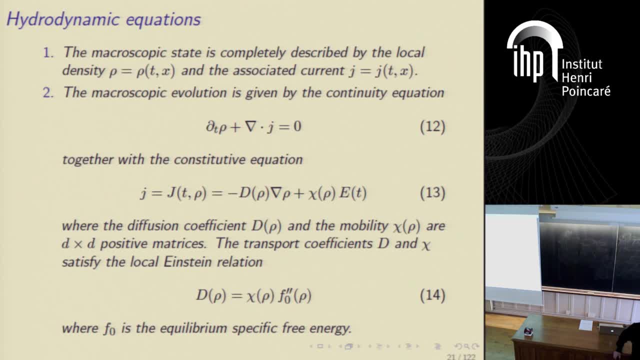 essentially on Sager theory, so near equilibrium. the discussion of the hydrodynamic equations is, you find it there. so here I will discuss, like the other day, the case of a single continuity equation. so rho may be a vector of thermodynamic variables, but I will discuss the case of only one. 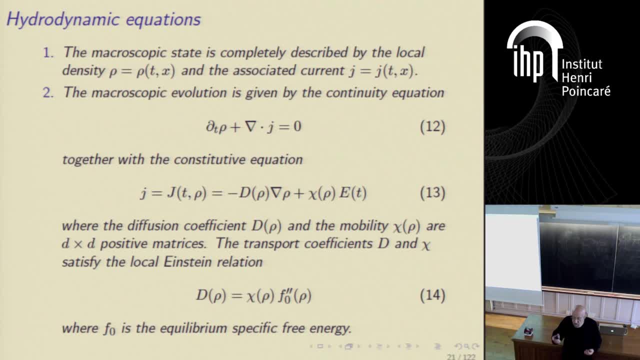 of them. of course, if you have more components, as Herbespona has illustrated at the end of the conference, you have a phenomenology which is much richer. so, but so I will try to present the essence of, of. so we you have a continuity equation, an expression relating 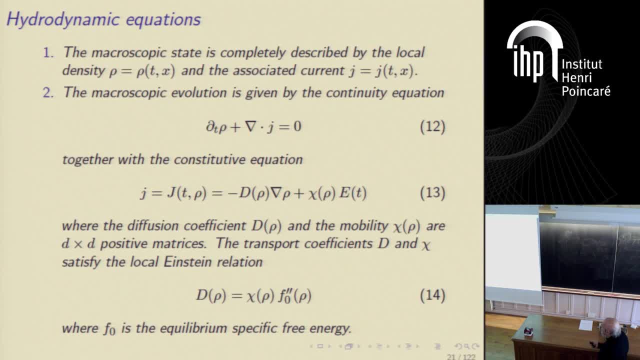 the, the current, locally to the gradient of the thermodynamic variables, and then there is an external field, and so you have these two transport coefficients and these are enough for specifying diffusive dynamics. and this has been stressed last week several times and this has are related by: 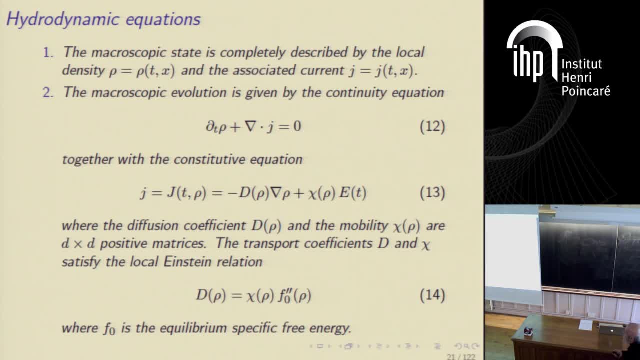 an equation which is called the local Einstein relation, again that in fact, with an appropriate definition, you can derive macroscopically. actually, at first you could consider a macroscopic translation of Einstein's theory of Brownian motion, but actually you can derive it macroscopically. I will tell you how. 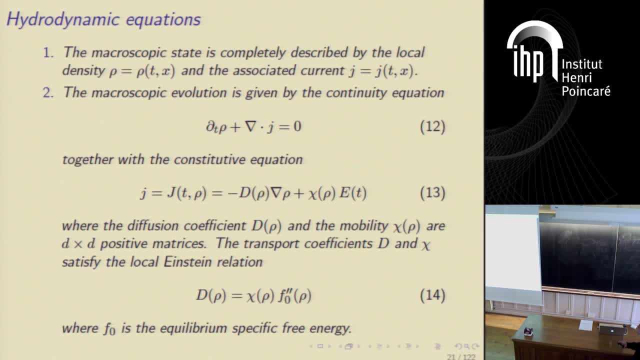 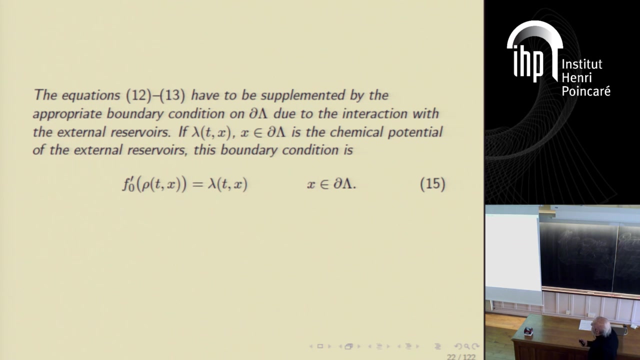 then. so these are the two transport coefficients and this is the second derivative of the equilibrium density of free energy. we shall derive an explicit expression later for this- and of course you must have appropriate boundary conditions and the relationship between the way you impose the boundary conditions, the way, if you want. 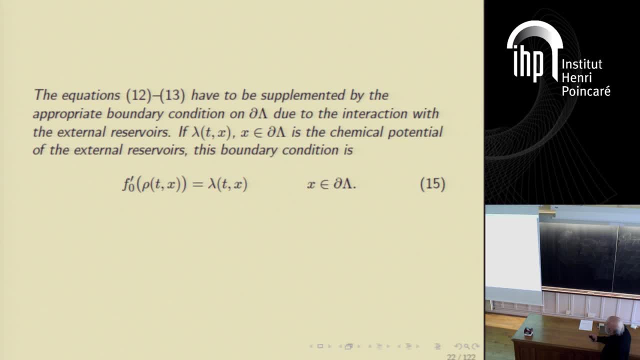 the boundary conditions are connected to the chemical potentials. lambda is the chemical potential of the reservoirs goes through the first derivative of the equilibrium: energy density. the fact that boundary conditions depend on time, then I have learned from a colleague mathematician that you can reduce it to the case. 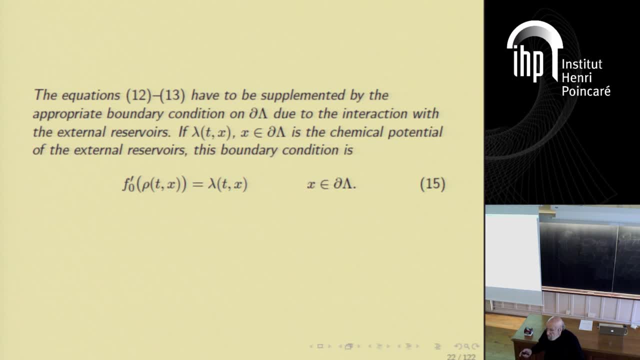 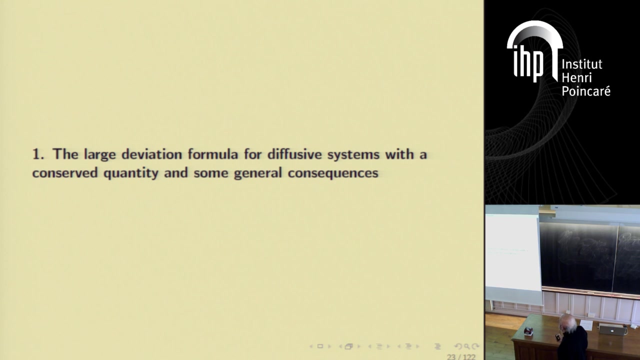 of the time independent boundary conditions by a simple transformation of variables and if you are interested, maybe another time I will show how you do that. but that is a purely mathematical question. there are no ambiguities in having time dependent boundary conditions. ok, so this is the formula. 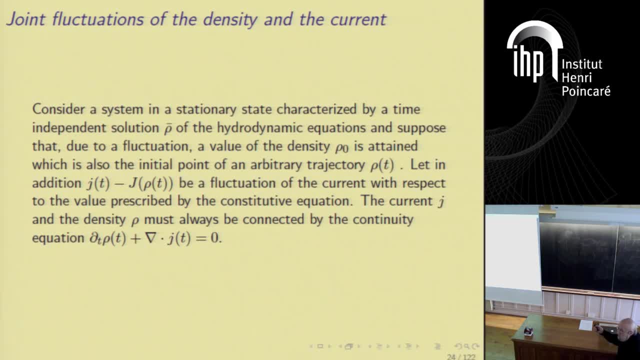 that I discussed the other day. for this formula the slides now are the same. so we are considering, we have a stationary situation, so typically you have a profile. so, for example, for a density, here are the reservoirs and then here the system is connected, and then typically, for example, 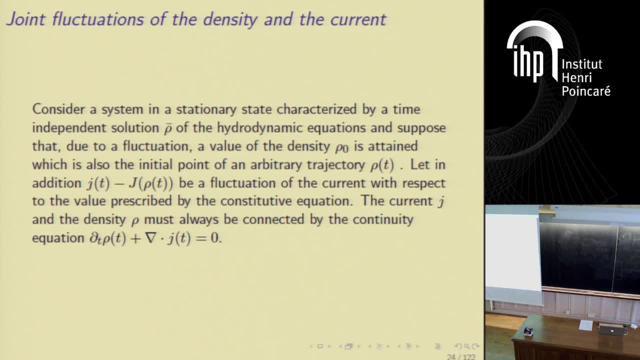 for the simple exclusion process. you have a density which goes through so linearly from some value rho minus to some value rho plus. for example, this is x, so that is what characterizes the stationary state, and and then you assume also that the current is fluctuating. 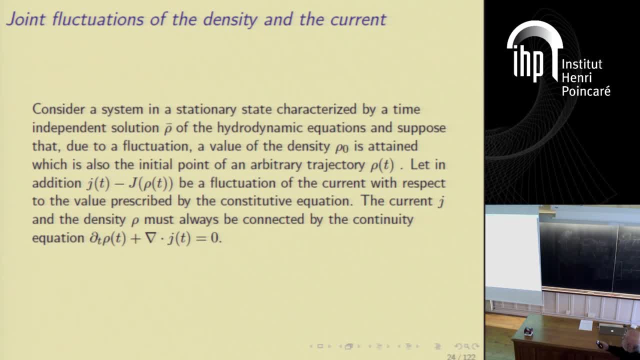 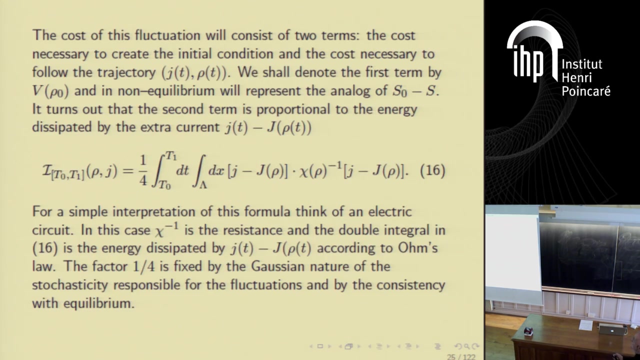 so there is a difference between the what is prescribed by hydrodynamics and the actual current that you see. so, and, of course, the fluctuation must respect the continuity equation, and ok, so, as I said, the cost of this fluctuation will contain, to term, the cost necessary to create. 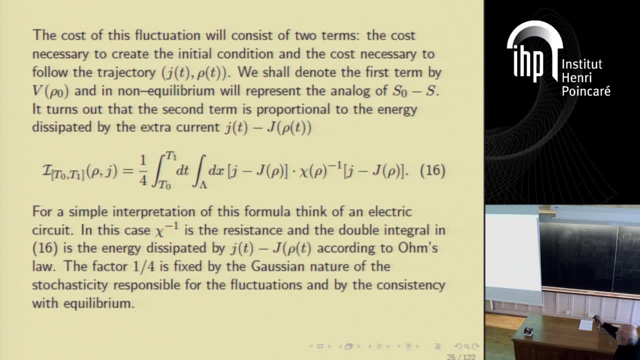 an initial condition, and then the cost to follow a certain trajectory which is not a hydrodynamic trajectory. that is something, and well, this, maybe I will sketch a proof of this relationship next time. and anyway, the final result is that you see the fluctuation squared with chi minus one. 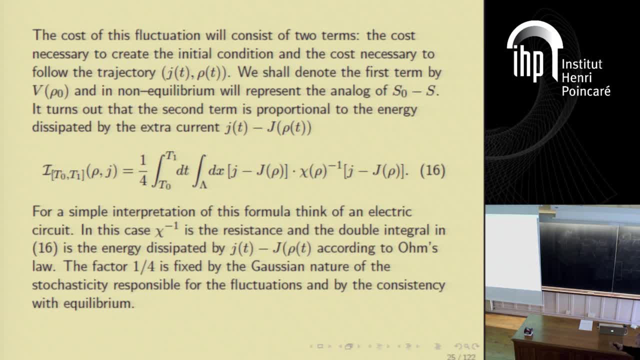 is the inverse of the mobility. so if you want is the resistance, and so this is the energy dissipated by the fluctuation during this trajectory. and then you have this factor one four, which is somehow mysterious because one half of it comes from the fact that, in the end, 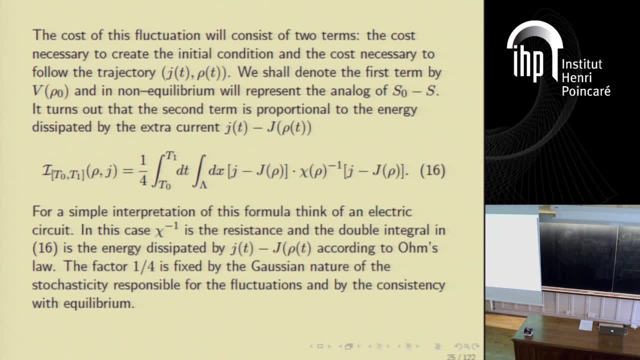 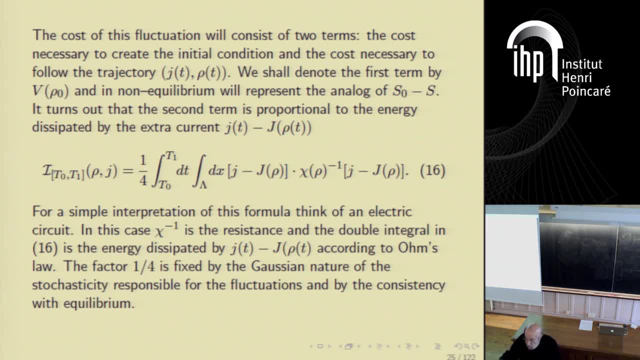 so, so, so, so, so. so, this is the so, so Well, let's go on then. Hm, The zero is just the deviation, the initial deviation, zero, just what you pay to have the initial zero from zero. Well, at the zero is when the fluctuation starts. 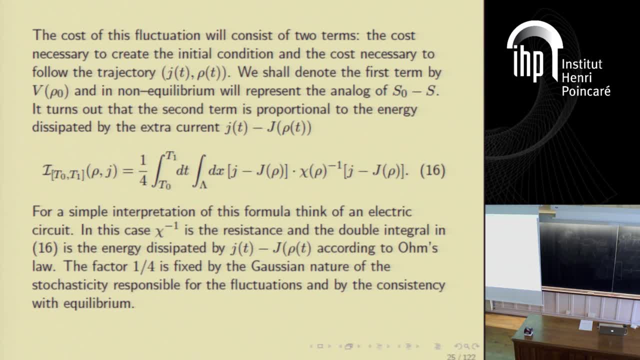 Then suppose you have a deviation of the density: Yes, And then the current just does what the density says, so Yes. Then this function No. Then this function yes. but then there is another term that I'm going to discuss immediately. 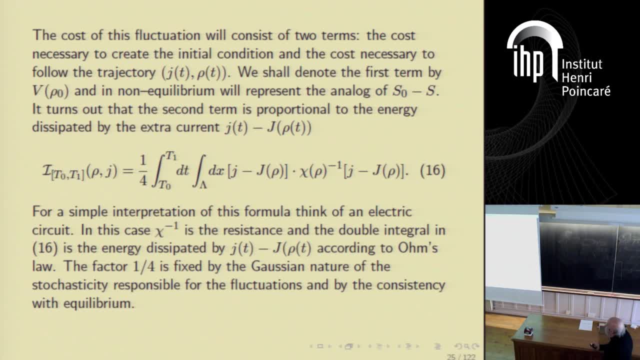 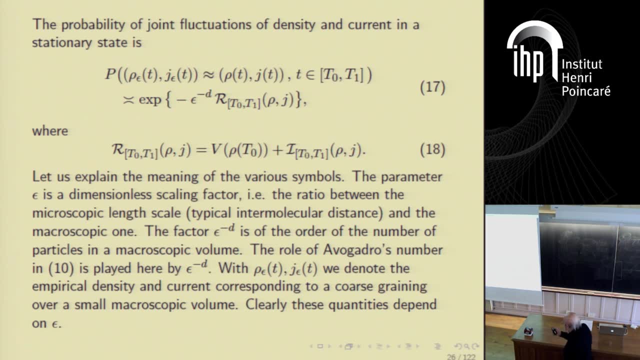 Okay, So now, what is the structure of the probability of the large deviation? There are, in fact, two terms. One is this dynamical term and the other one is just is the analog of the entropy of free energy in the. this is, if you want, is the term which was in the Einstein formula. 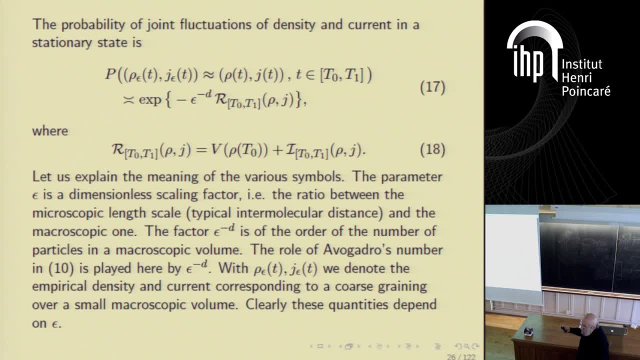 but here we are in general in a non-equilibrium situation. So this is the work: to create the initial, The initial condition. But then the two things may happen: You create this initial condition and then it relaxes with the hydrodynamic equation. 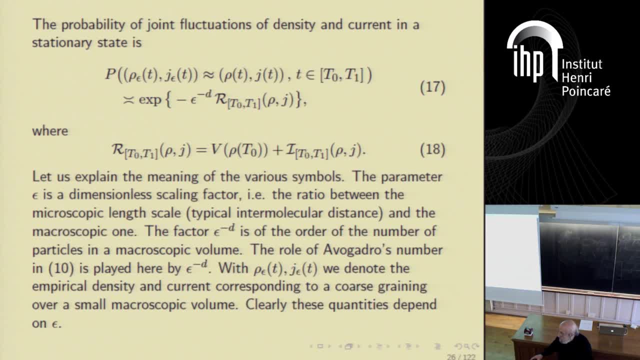 Then you don't spend any external work. If it relaxes, it just does that through hydrodynamic equation of motion, Okay, So in this case there is no current fluctuation. But if Yes, Okay, Then it doesn't relax through the natural hydrodynamic trajectory. and then there is. 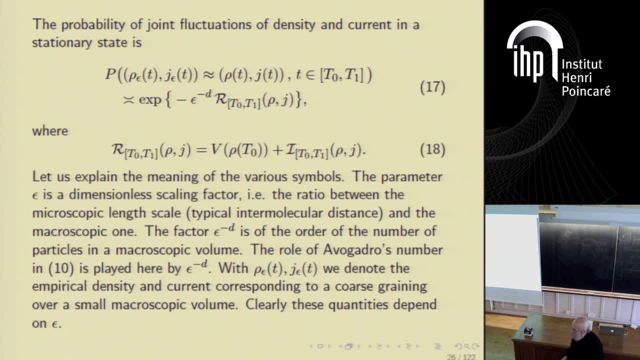 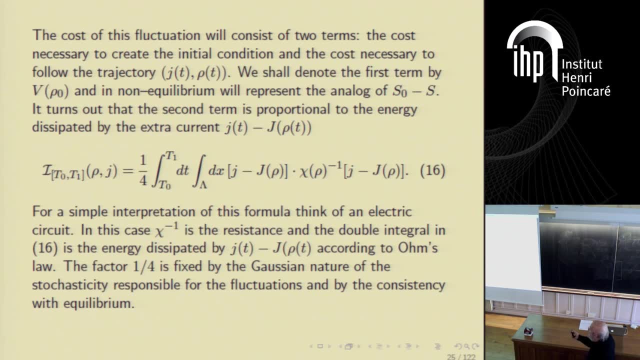 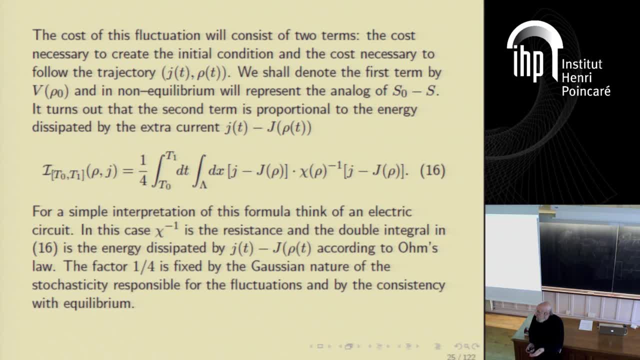 back to the stationary state following hydrodynamics: Yes. So now I make the deviation: Yeah, The density, Yes. And then I'm looking at the event where the this is doing a deviation, Yes, And the current is just equal J of rho, the rho of the deviation. 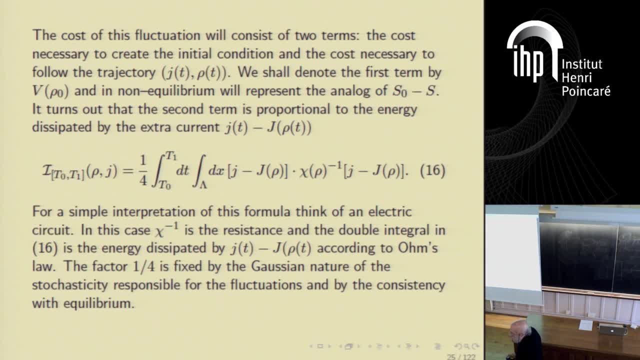 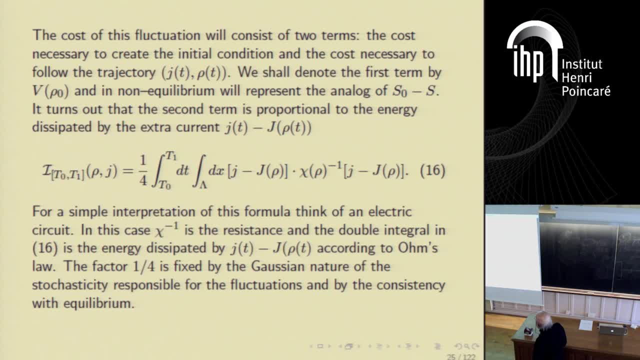 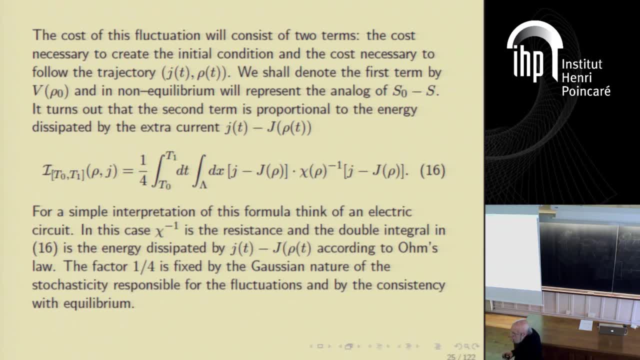 I would call it Well, the it is. whatever I chose to compute the function of the, then No, because I. So if you can, if you can give an error, it becomes one smaller one. Princed lounge. 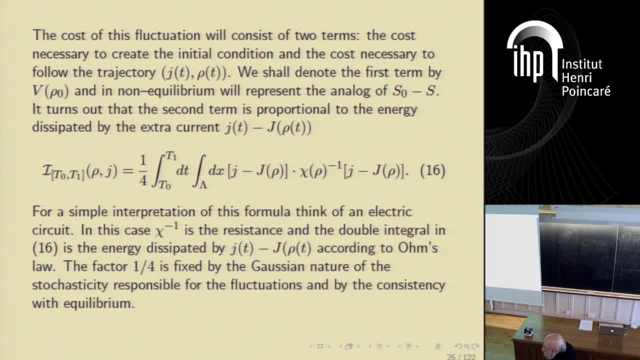 So you could create a function. I think It's like that. I assume that in the, I can choose rho and j. Yeah, provided they satisfy the continuity equation. Provided they satisfy the continuity equation, you can choose them arbitrarily. Wait then, why can't you just choose rho or just choose j? 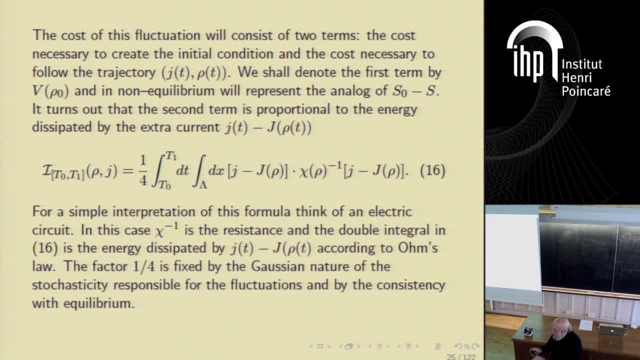 No, well, maybe this will be more clear going on. OK, I thought I could choose whatever rho and j on the left. No, j has always to be the divergence of rho. Yes, So it's not just a function of rho and j. 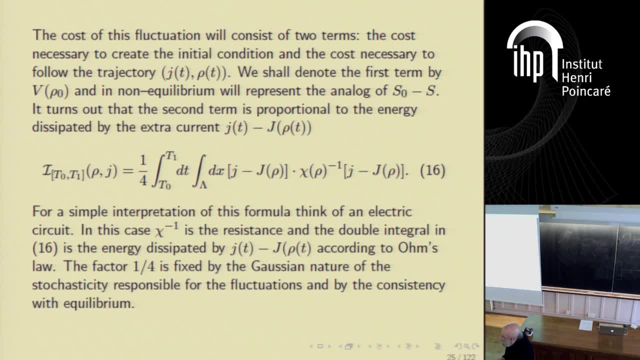 It's a function of rho. and then I compute the j in the divergence of rho. Yeah, So why do you write it as a function of the variable? just a function of rho? Yes, You don't know yet which one you want to put your focus on. 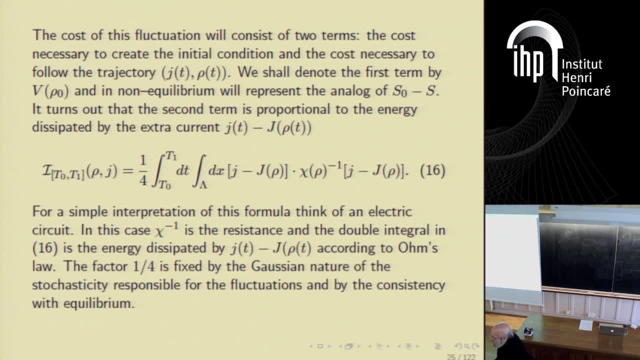 Maybe sometimes you want to look at j and sometimes you want to look at rho. That's right. But we should say this formula can be used even in cases. This formula here holds also in non-stationary situations. Well, this I will mention later. some results: 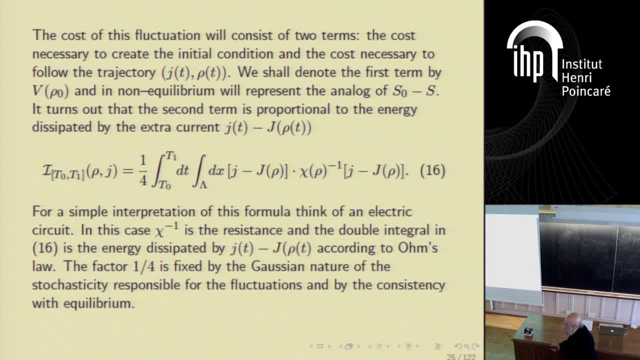 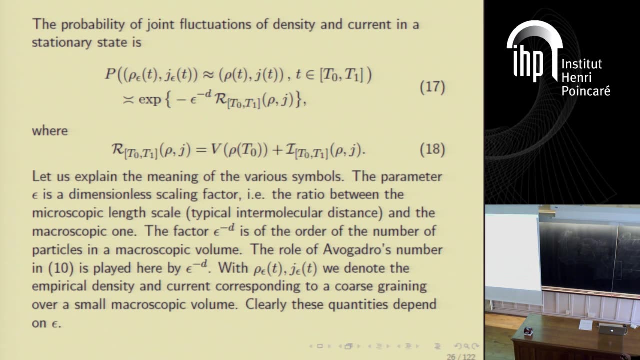 by Derrida and Gershenfeld, in which this formula is used in non-stationary states. OK, So this is the formula, the large deviation formula for a stationary state. So I emphasize that this is the analog of the entropy. 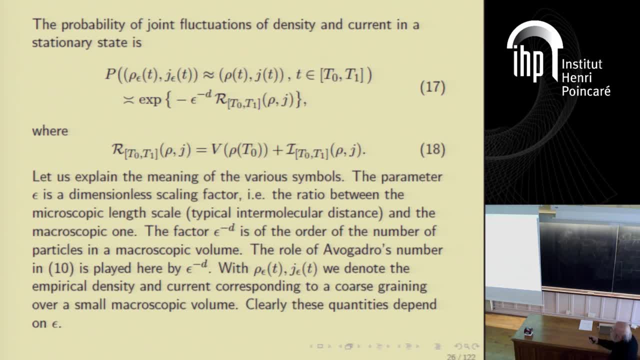 In Einstein's formula or more generally, of free energy, in this Landau-Lipschitz formula. Now, what you get usually is this: epsilon- This is the large parameter- is the inverse of this epsilon minus d. This is a typical iteration between a microscopic length. 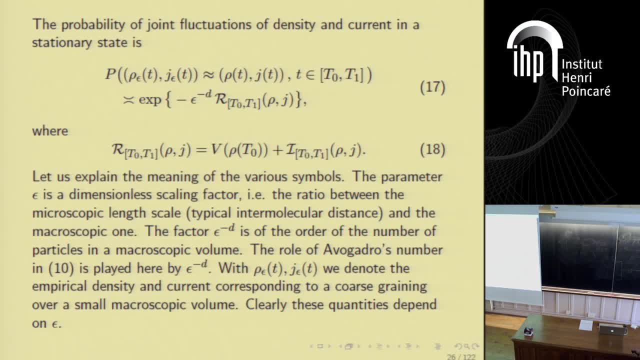 scale over the microscopic one. So this Factor here is of the order of the number of particles in a microscopic volume, So it takes the role of the Avogadro's number And of course this, what I call rho epsilon and j epsilon. 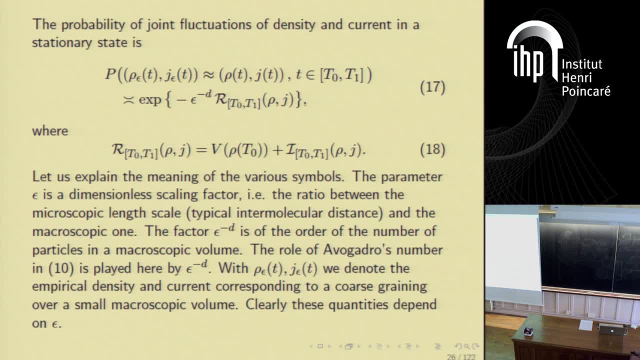 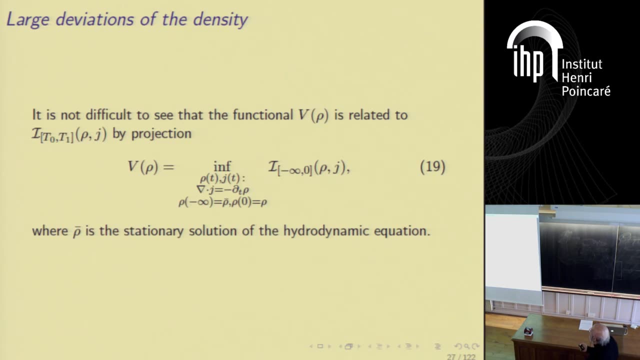 denote an average over a small volume on the microscopic scale. So they will depend generically on this ratio of scales. So this is the general formula which, and also the other day I mentioned that the two terms in this formula are related in the sense that by solving a variational principle, 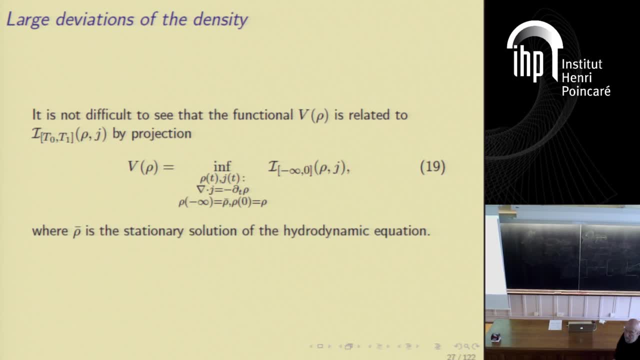 with our dynamical functional, you get this And I will show you later cases where you can calculate this, Please, yes, yes, it will be a sketchy description, But yeah, one has to be a little careful, But yeah, OK. 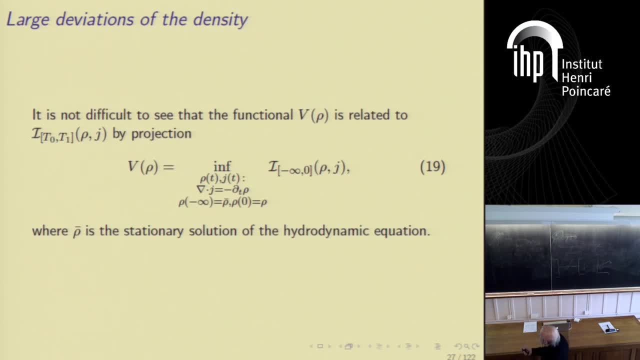 Now you see here, this quantity, which is actually, if you want, a basic Quantity for out of equilibrium, thermodynamics is related- is given by this variational principle. Now I want to discuss another way of characterizing this quantity. 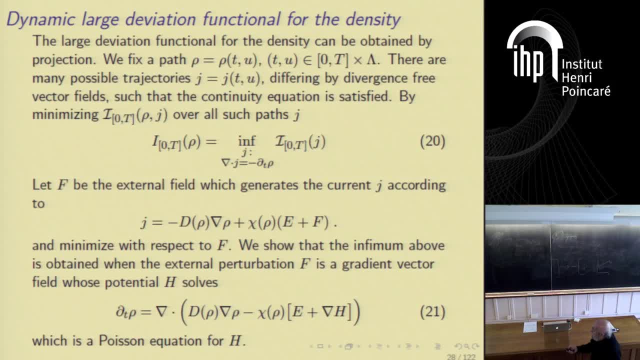 which is called the quasi-potential. So I will make, and I will follow, another way to characterize this quasi-potential, Which makes connection with a well-known theory for finite dimensional systems, which is theory of fluctuation for large. 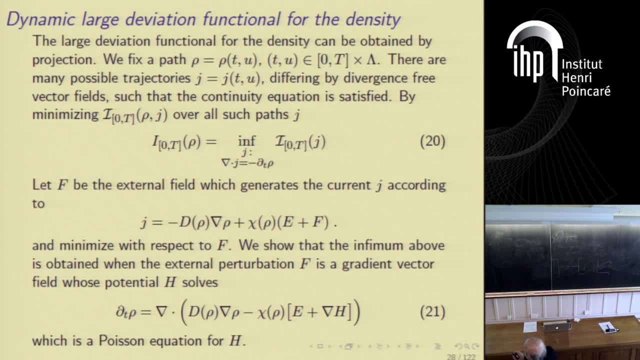 follows small noise. OK, You, well, you can read it. I think You see. So when you fix rho, this doesn't determine j, just for what we said before. I mean because rho and j are related. 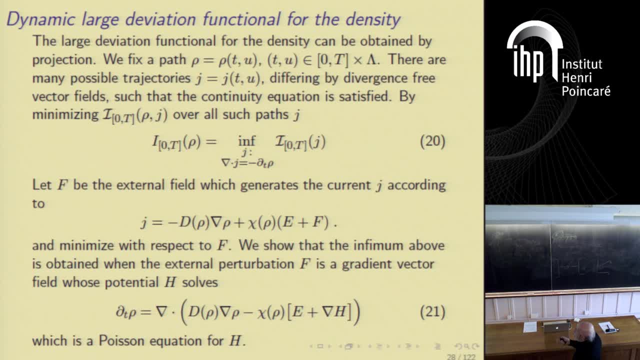 by the continuity equation, So you can add the divergence-free vector fields and the continuity equation is always satisfied. So you minimize all over all such path, over all j's, Such that the continuity equation is satisfied. 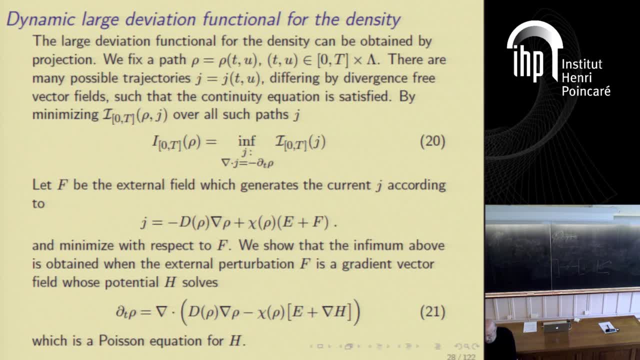 Now that is the way to calculate large deviations. It's an idea which goes back to, I think You add some external constraint or field in such a way that the fluctuation becomes the well you'll get, well the opposite here. 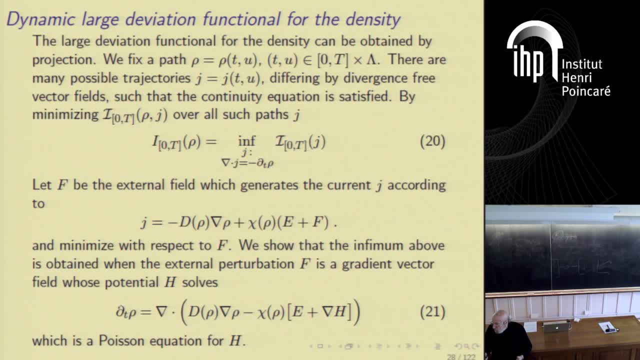 the law of large numbers so becomes the most probable value, and in this case the. maybe you were the first, with Baradun and Kipnis, to use this generalized the Cramer point of view. is that true? yeah, but he considered only the the case. 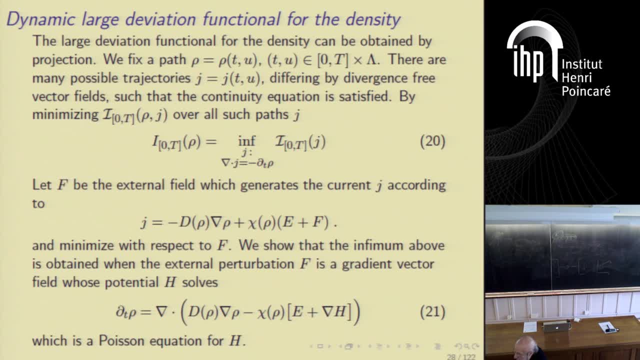 of variables which do not depend on space. it was a. it was much simpler, okay, so the way you do it is that you introduce another external field. he was the external field already present on the system, and F is another external field with which you, your fluctuation becomes. 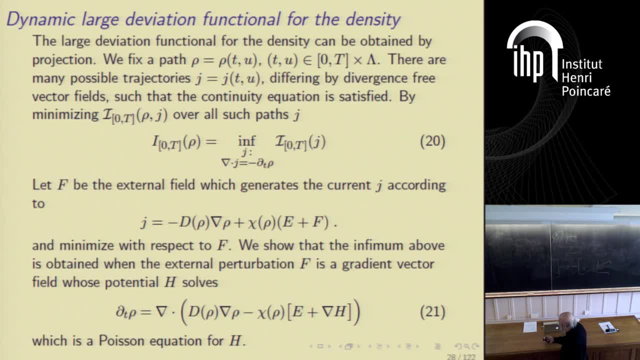 typical, as it's yours, and then you try to minimize with respect to F. now, the interesting thing, because that the you don't have to, in fact, to minimize over all possible fields, but for the density is enough. you don't have to, in fact, to minimize over all possible fields, but for the 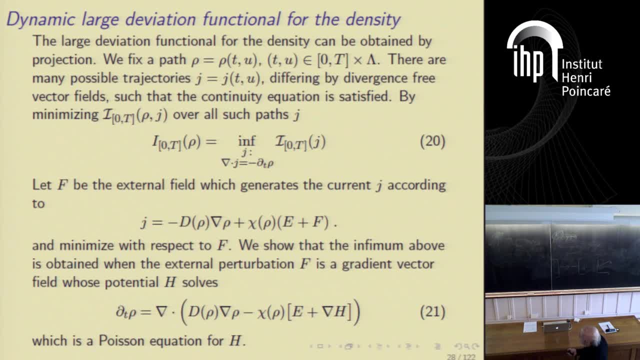 to minimize over external fields which are gradients of some potentials. so, actually, and how do you find the field necessary to create the fluctuation? well, you, we are speaking of a trajectory, consider a trajectory, and so which is time dependent? so you take the new hydrodynamic equation with the addition of this external potential and, of course, this: 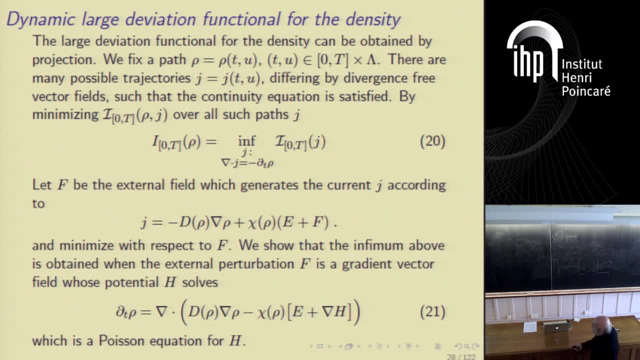 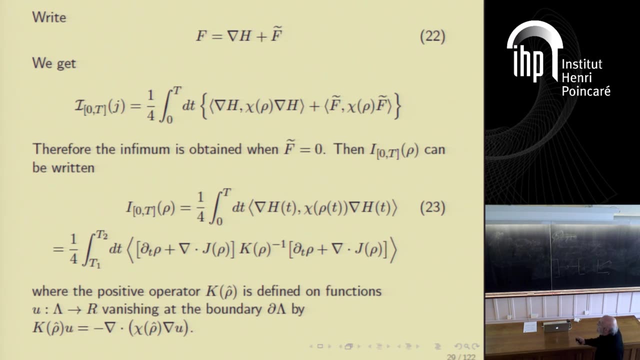 you may consider this as an elliptic: if you fix row, then this is an analytic equation for this external potential. so in principle you can solve it. and then you you split in general your field in a gradient path and they know gradient part. you rewrite your functional in terms of these fields and then you minimize and 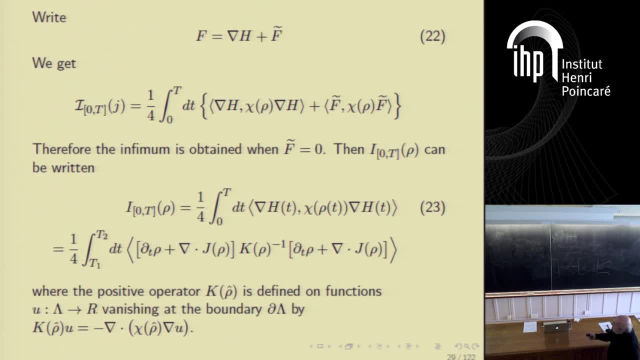 then you see immediately that this part here, in fact, can be thrown away- is a positive object. and then you are left with the following large deviation, functional for a trajectory of the density which, as you see, is nothing but the hydrodynamic equation in which you 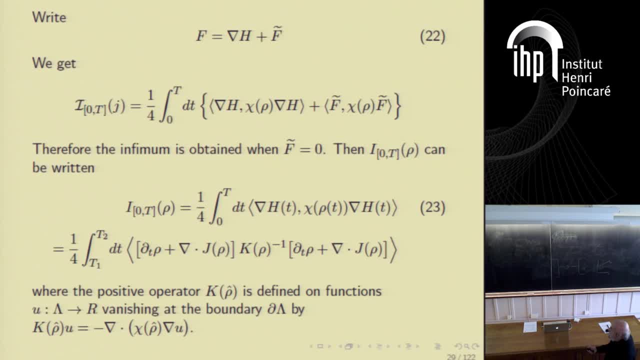 have brought everything on the same side. And k is the inverse of the mobility, but it's an operator in general, because you have space dependence. So this is a, you see, who knows, the people who know of Wenzel and Friedlin theory. they don't know that this is the. 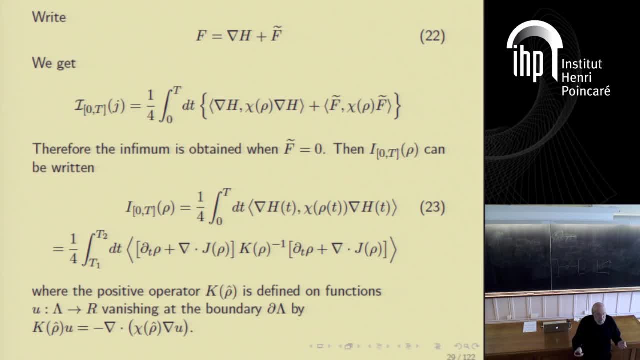 case For dynamical system, you add the noise and then the large deviation functional is given just by you bring. you have a Langevin equation: you bring everything on one side, and so you see that the fluctuation is measured by how much you violate the. in this case. 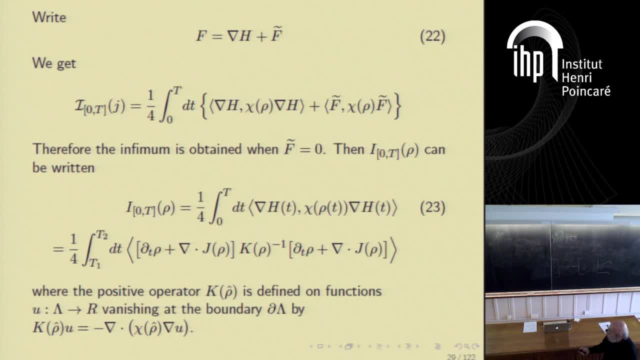 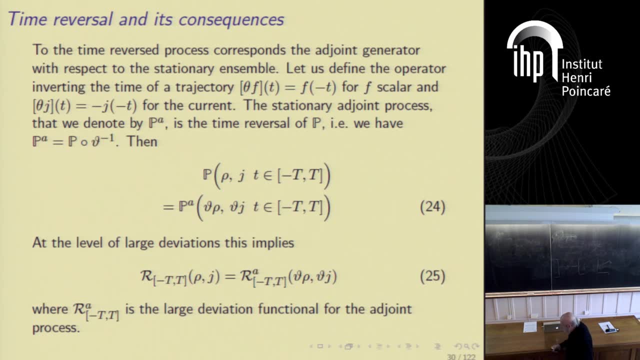 the hydrodynamic equation and, in the other case, the equation of motion. Okay now, so we just remember that for having the, for calculating the trajectories, the probability of the trajectories of thermodynamic variables, we have a dynamical functional which contains the hydrodynamics. 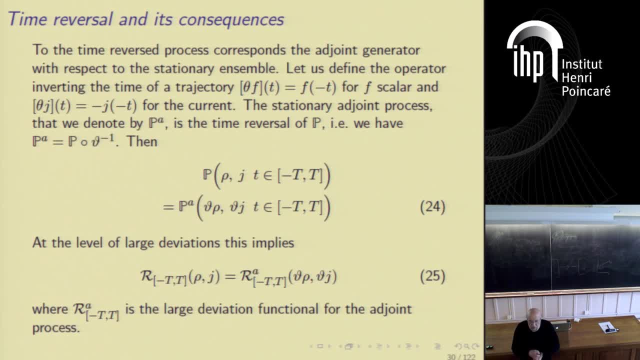 Now it's already about one hour that I'm speaking. What do you want to go Me? I could go on for another half an hour, or we can make a break and then continue. What? no, that's what the audience decides. 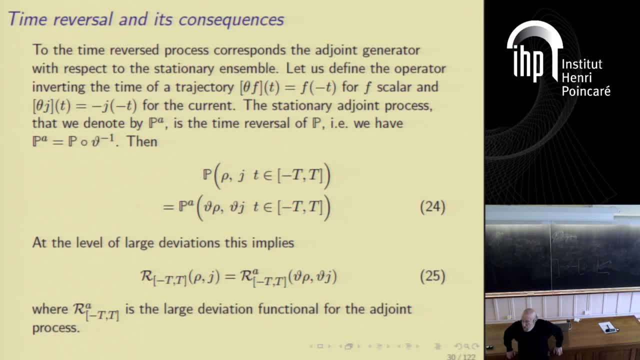 Gone Good for everybody. Okay, I'm trying to go slowly, so, But if you don't understand that, please interrupt me. Okay, so this is the same slide I've shown the other day. You define the time-reversed quantities and you define the what is called the adjoined process in this way. 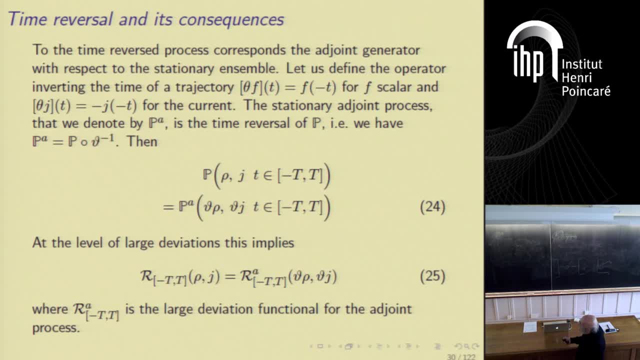 So you take the probability of a certain trajectory. I take the interval of time minus tt in order: Time reversal: you are in the same, in the same interval, And the level of large deviation. this implies that you have an exponent for the direct process and that's. we know already what it is. 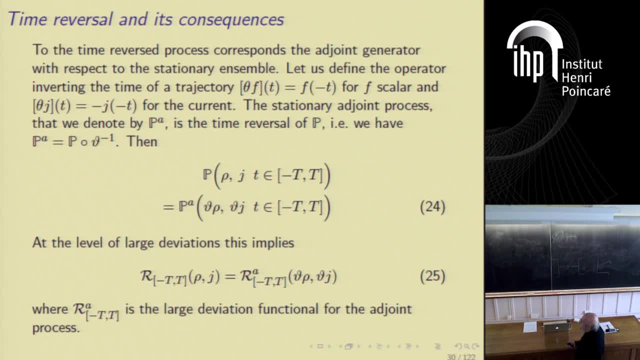 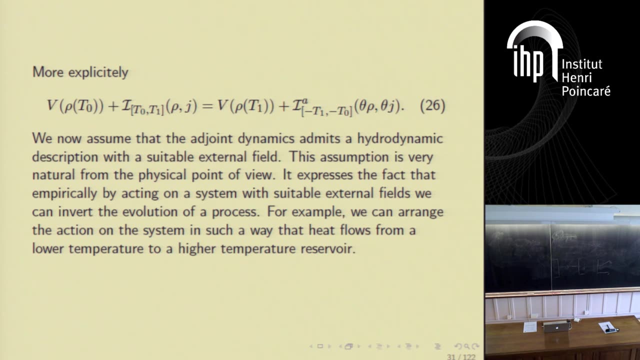 And then there will be an exponent for the time-reversed process which has to be evaluated at the time-reversed trajectories, Okay, Okay. And then there will be an exponent for the time-reversed process which you don't really know, right? I mean, it's a. I mean, the time-reversed process is a complicated object. I mean, in general, you're not so easily computable, right? 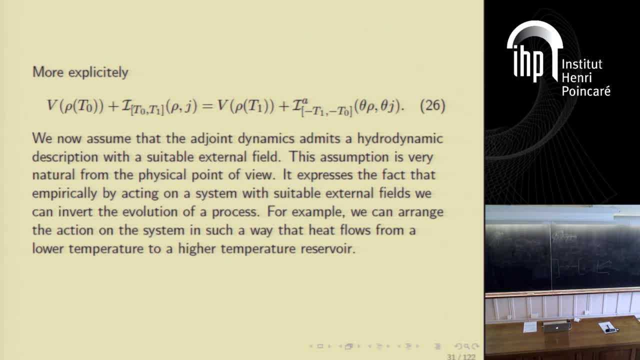 No, Yeah, that's what I just wanted to emphasize. I mean that- Yes, I mean forward dynamics- is sort of given to you by defining the model, but I mean the reverse process. But I will give an explicit expression for the current. 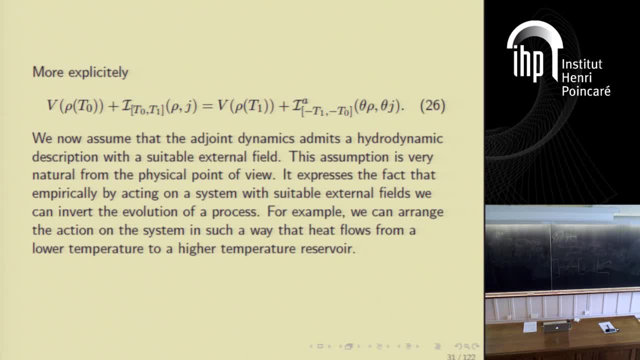 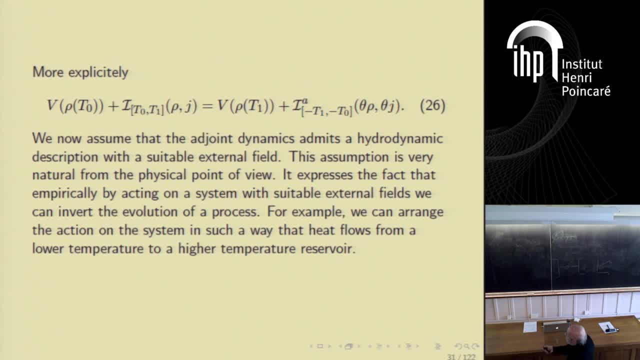 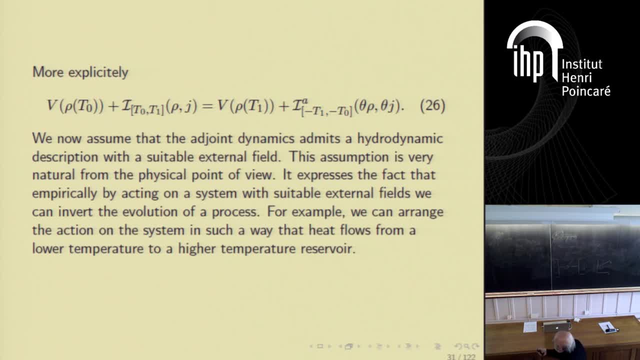 So this is what it is. It's just this quasi-potential, But then you see, therefore, the adjoined process, or time-reversed process, which is called the IA, and then you evaluate it on this time-reversed interval. 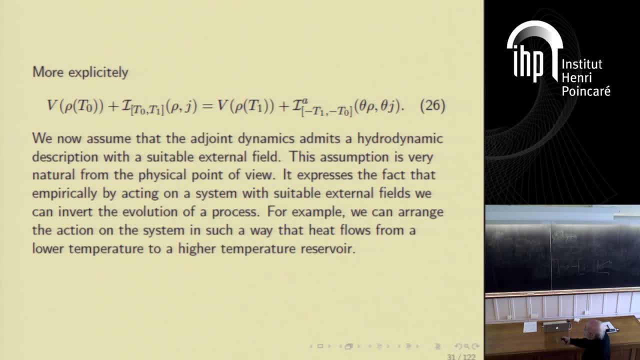 At the moment, we don't know what is the form of dysfunctional, However. and then the next one is an assumption At the level of existence of a time-reversed process. I think this is an everyday experience Because I mean, as I said in my talk, I mean you can always by acting from the outside. 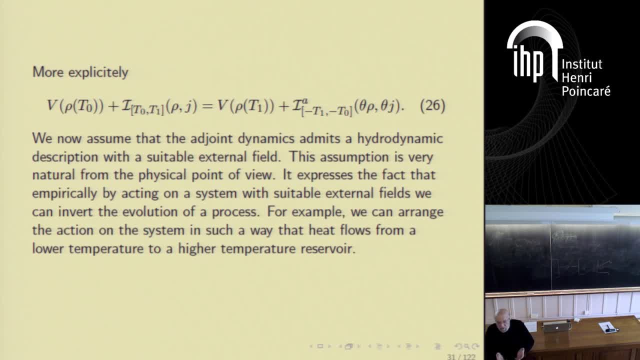 have heat flowing to a higher temperature reservoir. So in principle, this can be done. Now the question is: can you do it with the external fields? Yes, As we shall see these external fields, even in simple model And do not have a very simple structure. 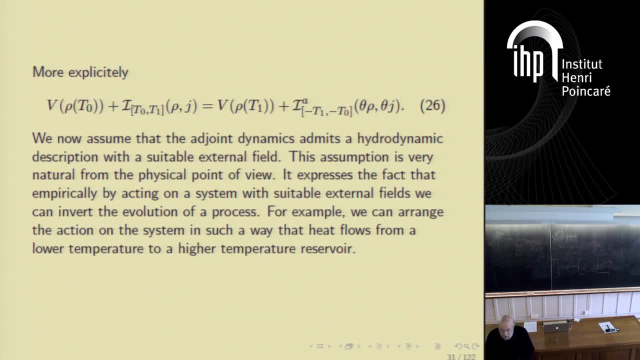 That is connected with the remark of Herb Spoon, But the question here: you assume that the path probability for the forward process is equivalent to the path probability for the joint process. Which property is equivalent? The path probability for the forward trajectory is equivalent to the. 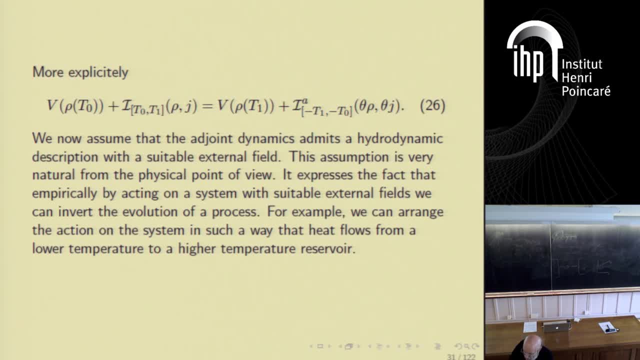 The, The, The probability of the reverse process, of the time-reversed process. Yeah, But the system is in state and it is irreversible, right? No, no, no, But you have to distinguish between time-reversal invariance, which is something. 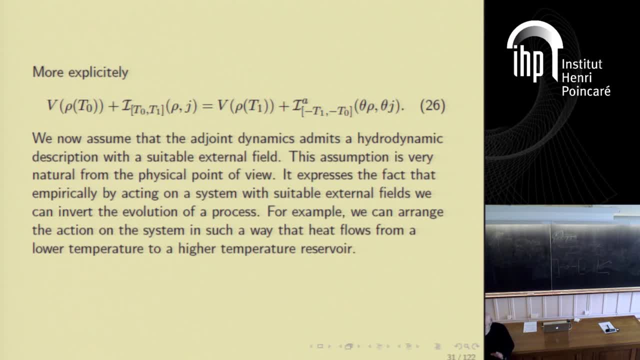 which out of equilibrium is violated, and existence of reverse dynamics, which are two different things. So it's clearly lost the time-reversal invariance. when you go out of equilibrium, You see, for example, you put boundary conditions, so you violate parity and the CPT theorem. 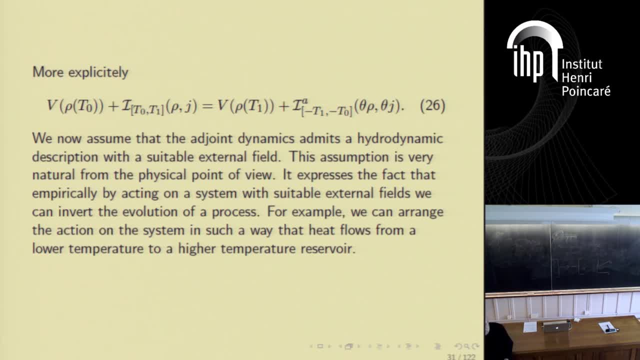 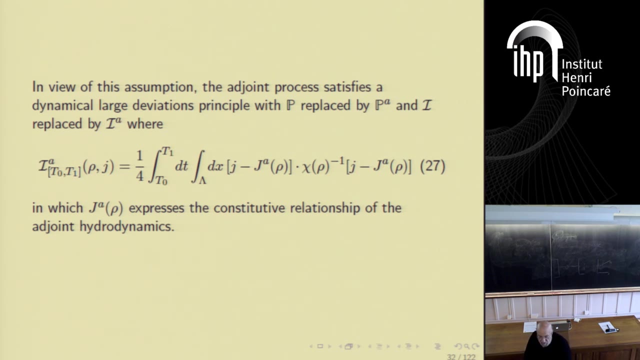 tells you that also time-reversal is violated, OK. But now we assume non-reversal. OK, OK, OK, OK, OK, OK. So we assume that not only the existence of the time-reversal process, but we assume also 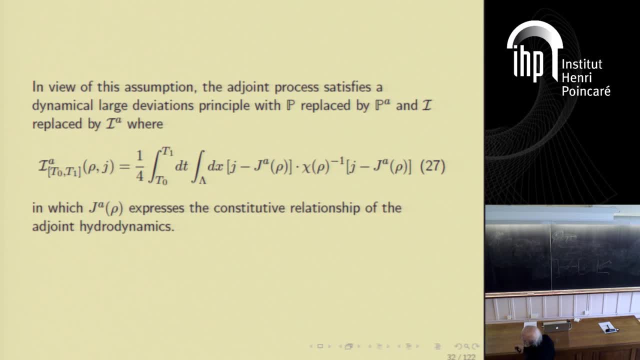 the fact that there is a hydrodynamics associated with the time-reversal process and that there is so a new constitutive equation associated with the time-reversal process. This is a stronger assumption, But which is verified in models. we shall say: 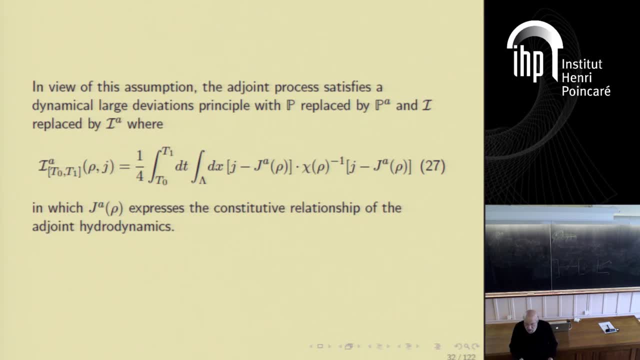 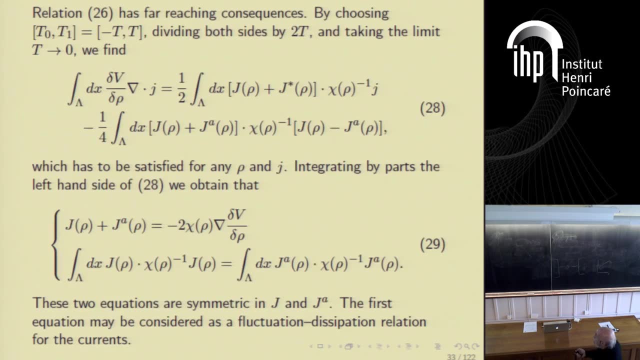 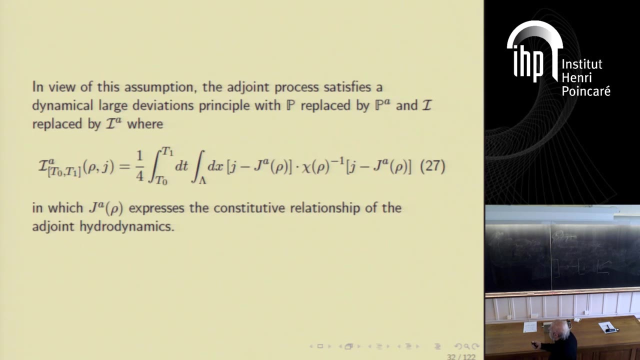 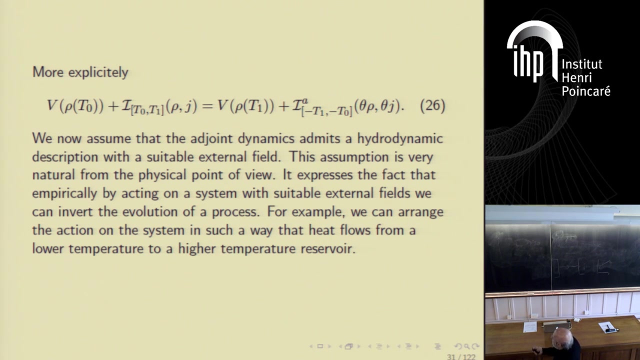 I mean for Markov processes. all this is very natural, OK, OK, natural. And since our best example are. So now you play with this time reversal invariance relationship, So you divide by time and you take the limit of time. 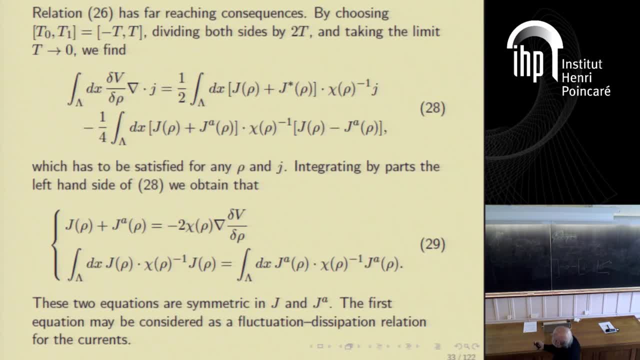 going to zero. so you get some derivatives and then, I mean, you get a relationship which has to be satisfied by for every row in J, and that provides you with two relationships. So you see, this allows you to express the current of the reversal process in terms of the original current and something connected. 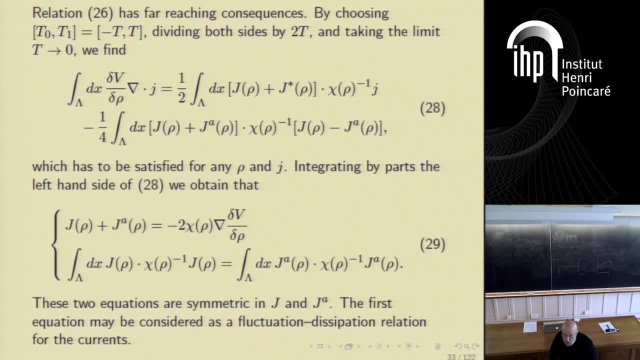 with the quasi potential. So you see, this is a current because this is a gradient of the quasi potential and this is the mobility. So this is- you may read this as a current fluctuation relation. Usually they are not given in terms of current but and this is that the dissipation of the first process and 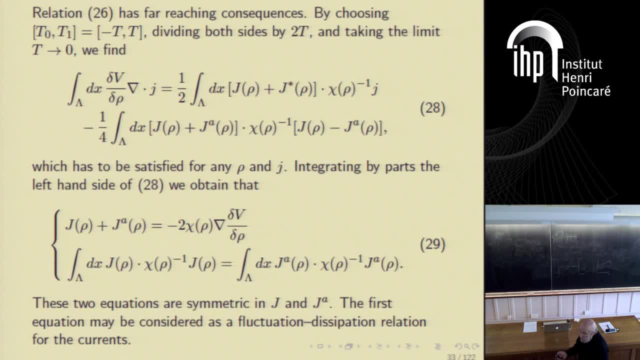 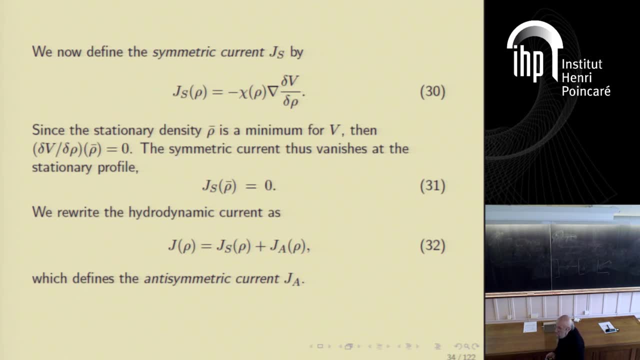 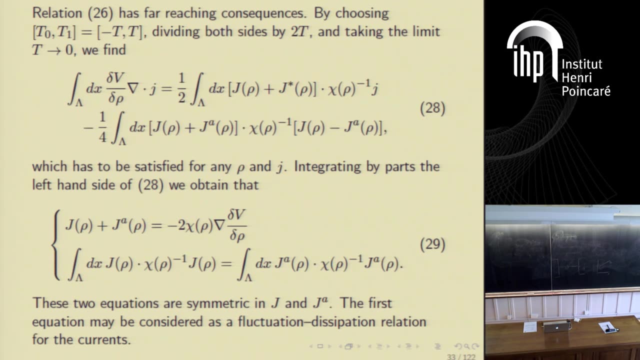 this time reversal- are the same. So you have these two equations which follow from the equation above, and now I still have a question on your notation. I mean, in the example, I mean the ordinary current is really just a function of the density. Yes, 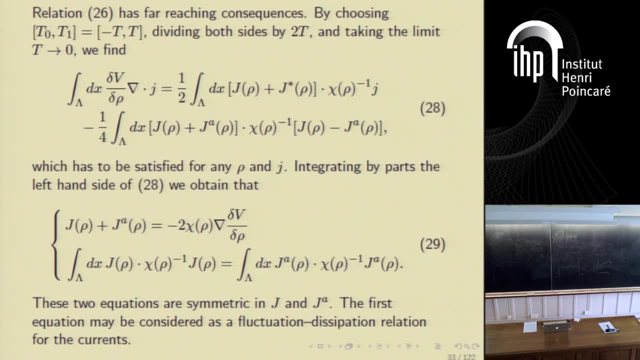 But now when you look at the reverse current, is it functional of the density or is it a function of the density In general? it will be a functional of the density because this object here is no local. So this the quasi potential in general. but we shall calculate examples of the quasi. 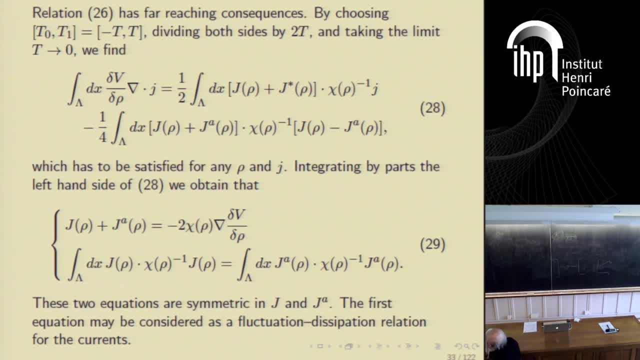 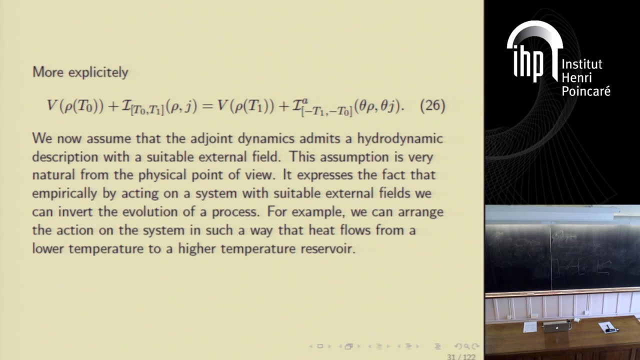 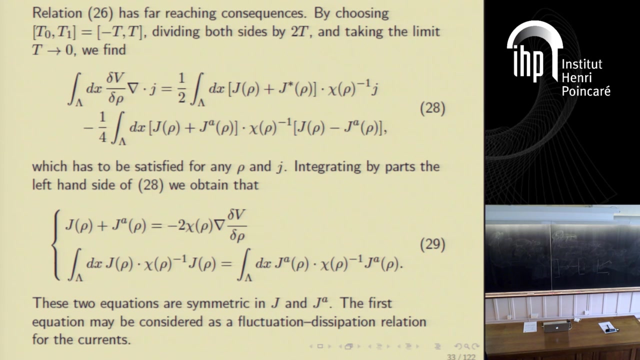 potential. So, and the quasi potential is not local in space, So the time reversal current will be a non-local function of the density. Well, it's a direct consequence of this relation. here You divide, you see, Okay, You divide by twice, by the length of the interval. then you send the length of the interval to zero. 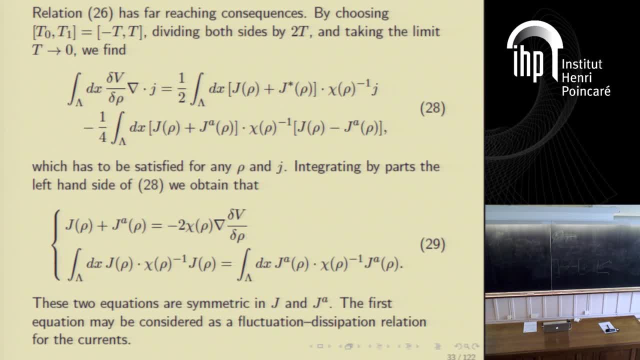 and then you derive this relation. Now, this relation has to be satisfied for every row and for every G star. and J a is the same. Yeah, I'm sorry, The answer is J a. It's a mistake, It's the same. 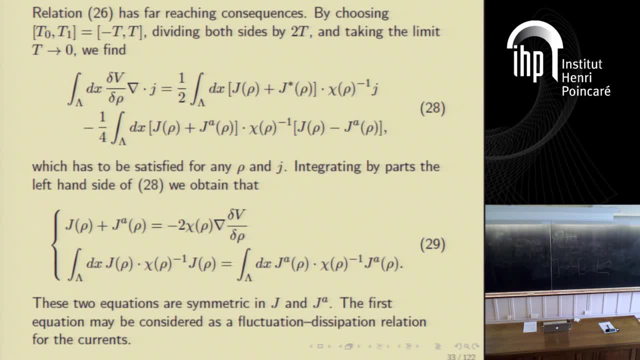 No, no, no, I mean it's an error. It should be J a, J a Okay, Everywhere. No, I never introduced J star Okay, So I made a mistake. Now it's a relationship which has to be satisfied for every J. the fluctuation of the current 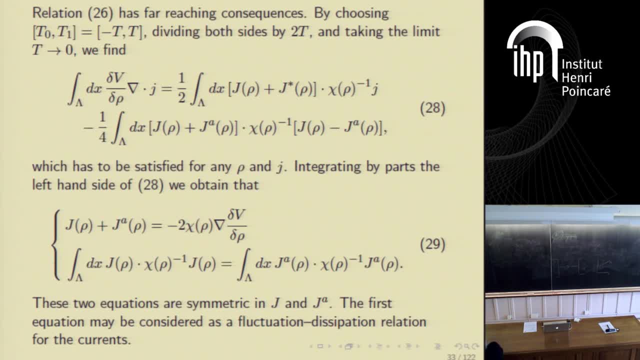 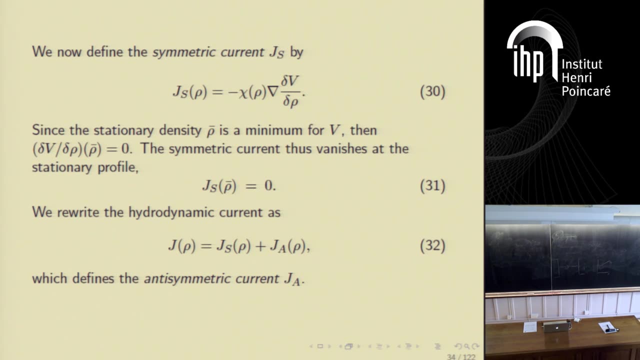 which appears here and here and every row. So, And then you find these two relationship. You are saying that if you find a way to reverse your dynamic, I will discuss the measure of the quasi potential. The quasi potential can be either you calculate, 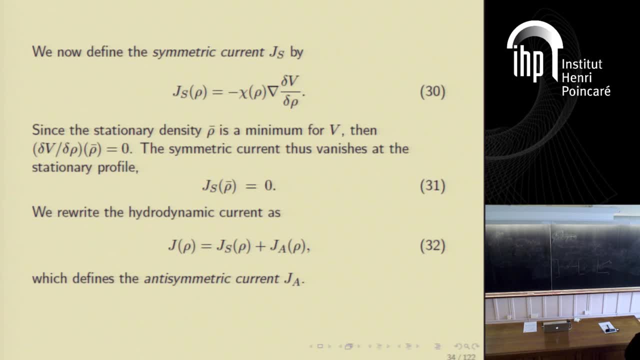 it and I will see how to calculate. Or you can measure, because essentially it's a generating functional of correlation functions in the stationary state. So by measuring some correlation functions you can get some good approximation to it. But in your former equation you were able to 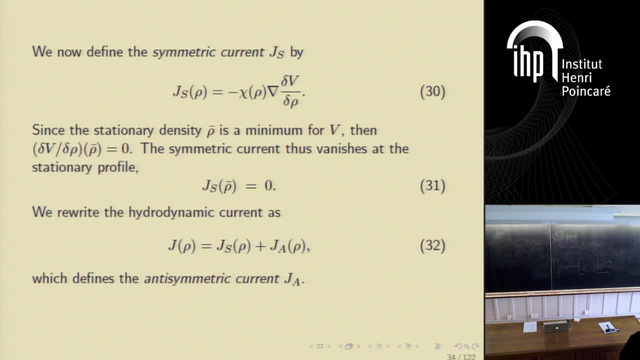 No, but so far I mean this J was defined by the variational principle Which, when I introduced at the beginning the formula for fluctuation, I say that V is related to the. Yeah, So I mean, in principle you can calculate it. Now to measure is another question and that will come up heavily in a while. 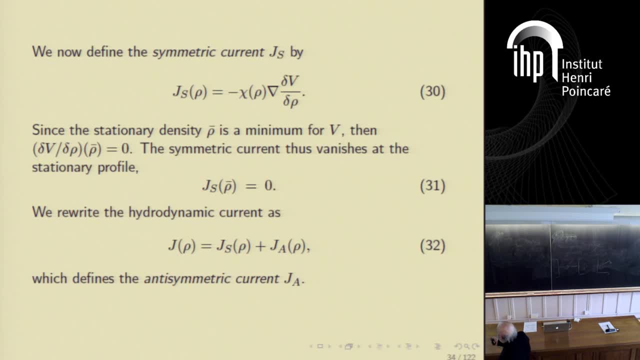 Okay, So, as I said, I define this I call symmetric current because we shall see that under time, reversal doesn't change sign, The dissipative part doesn't change sign, And so the symmetric current since V as a minimum on the stationary state. 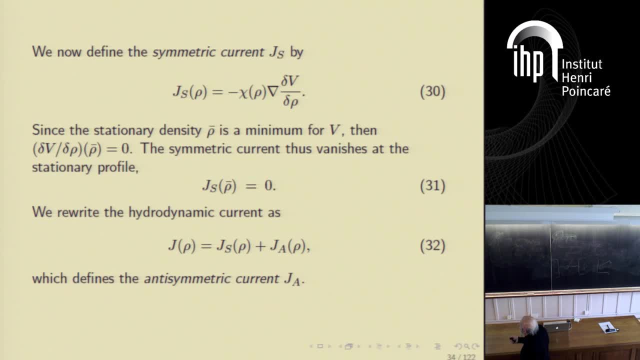 So is zero on the stationary state. So in the stationary state The whole dissipation is given by the other part of the current, The anti-symmetric part. Something that confused me always here- Terminology maybe that is used because somehow current is something always anti-symmetric. 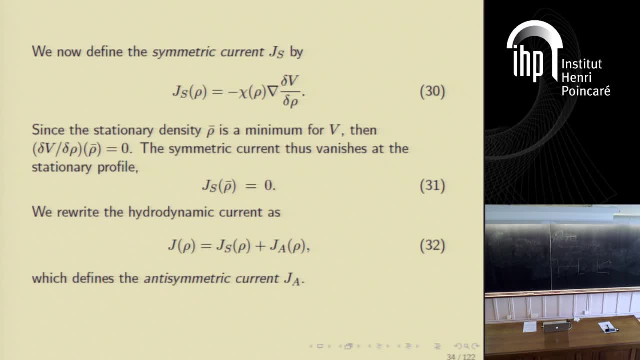 You still call this current symmetric. What does it represent? I call this symmetric. I mean the. What is the problem? Because I mean I didn't say No, no, No, no, No, no, no. The point is: 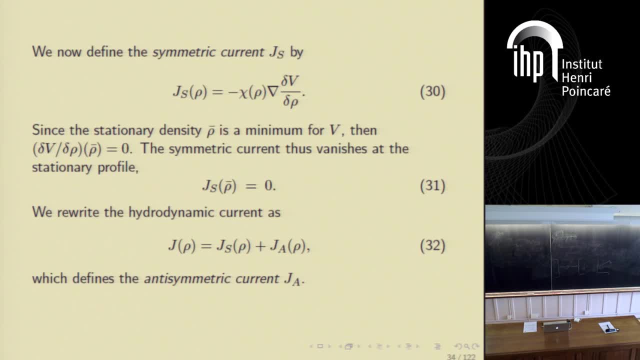 Something associated to something that you said before. that changed sign No. no, But I did not define how this J of rho behaves under time reversal, So we shall now find out how it behaves under time reversal. I think that has been one of the good things of the macroscopic fluctuation theory to clarify. 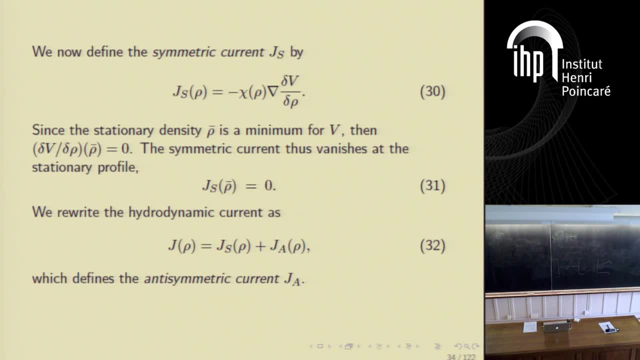 these aspects. This is the splitting of the current I have never seen in the literature. So if it is something you are not used to, it's right. No, but I, You said it, You said macroscopic and you said current. 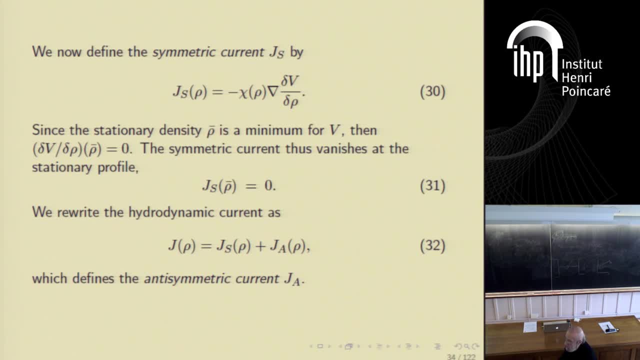 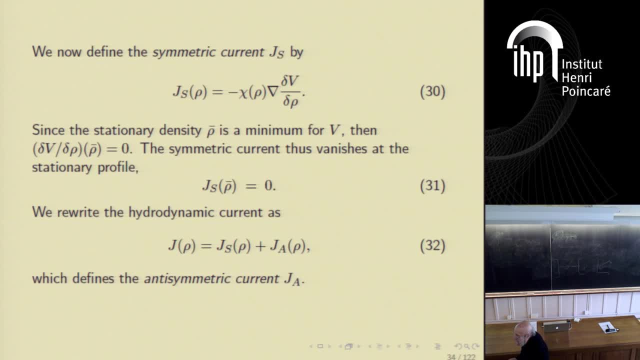 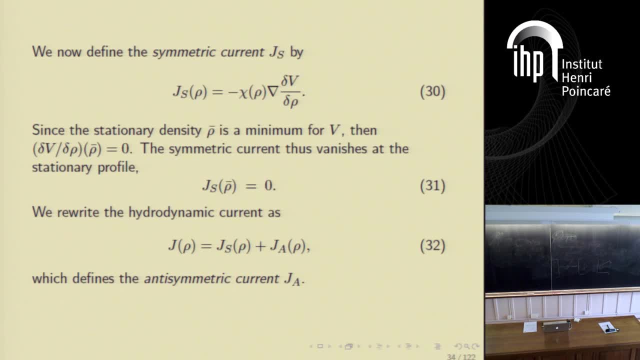 No, no, No, no. The current on the time. reversal: The current, The current change. If you go to the reverse process, the current changes sign. But here we are speaking of the constitutive equation. So what behaves in a more complicated way is the J of rho. 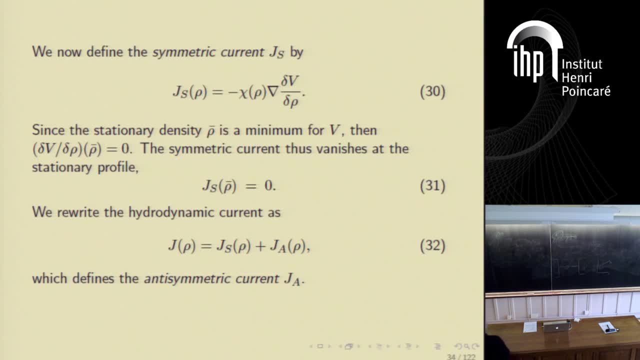 OK, We OK, OK, OK, So I split, I introduce this and split the current into two terms. The second term is defined by the difference of the total current, which you know Because it's given by hydrodynamics. 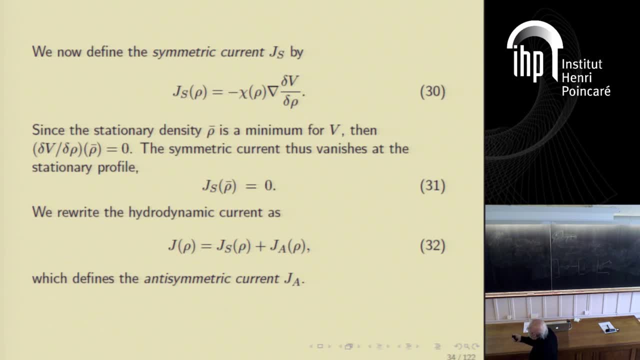 And this part here is known once you know the quasi potential. OK, So you see that since the quasi potential is in general non-local, So also this part here will be non-local. But the splitting is interesting because it's It allows to define clearly what the properties under inversion of time. 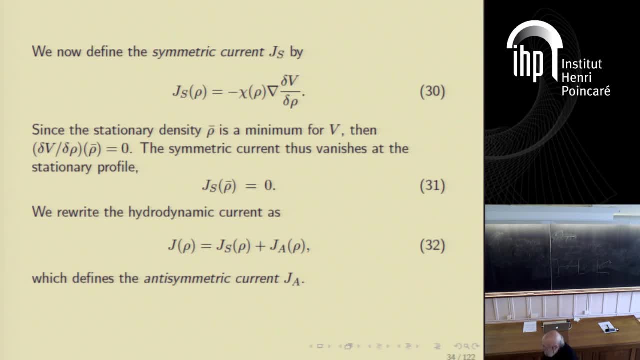 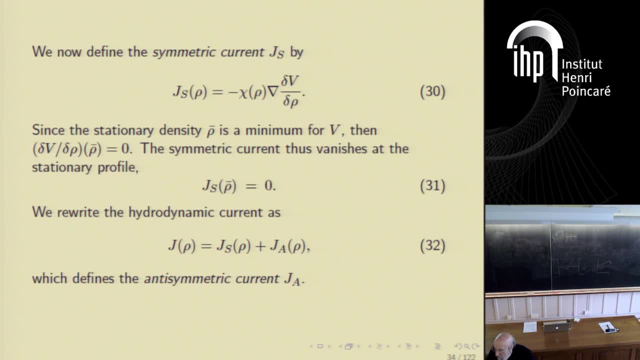 No, No. In a stationary state, I mean, we takes theầu the place of entropy, of equilibrium. So in this case it is a current. But a current dissipates energy through Ohm's formula J, squared times, resistance gives you the heat produced. 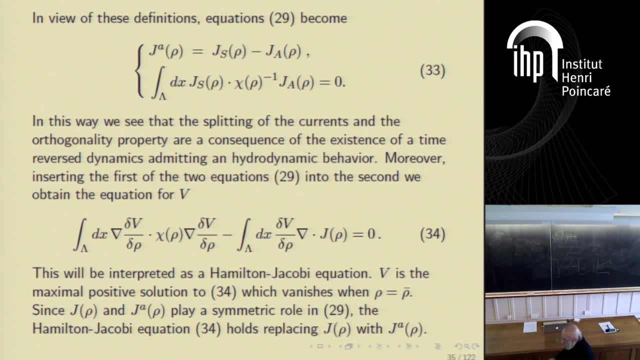 OK, Well, I hope I will convince you at the end of that. OK, So if you make this definition, then you see that the J associated to the time-reversed process, to the hydrodynamics of the time-reversed process. 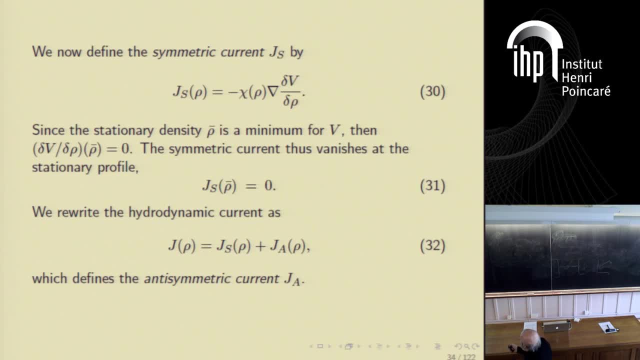 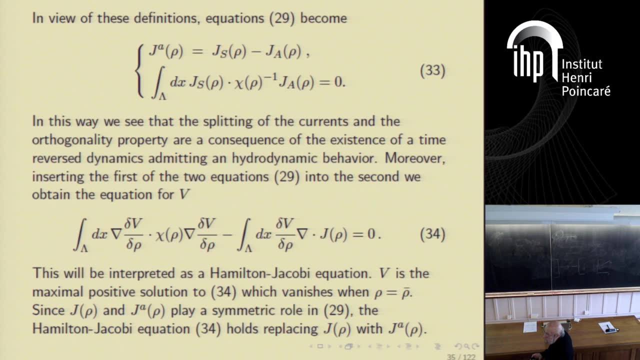 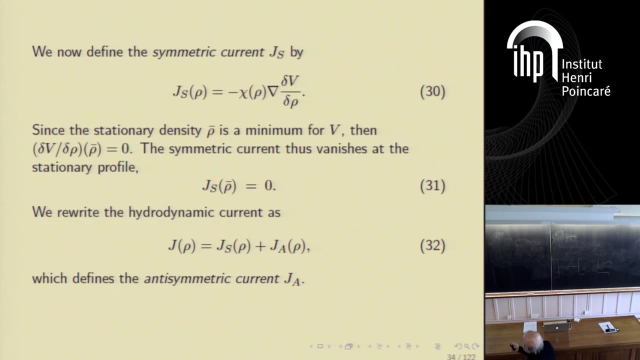 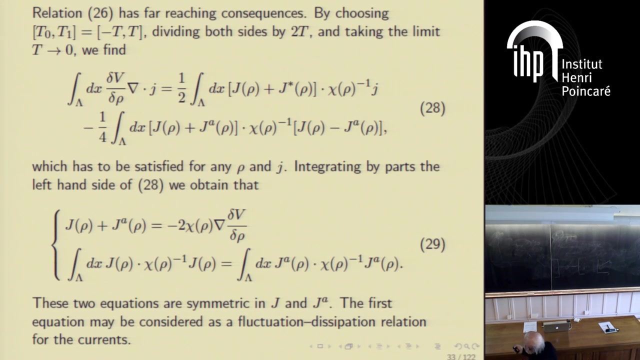 is 1.. While the direct one is just the sum of these two currents, the other one is the difference. And then you'll discover that the other equation, this equation here, if you put inside the definition of symmetric and antisymmetric current, tells you that these two 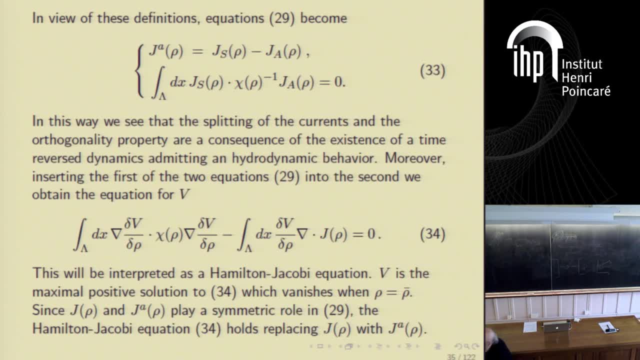 currents are the same. These two currents are orthogonal. You integrate our space and these are orthogonal, I mean. so, you see, usually I believe that when formulas are simple and have some aesthetics, that's the right way. OK, Now, if you go back, 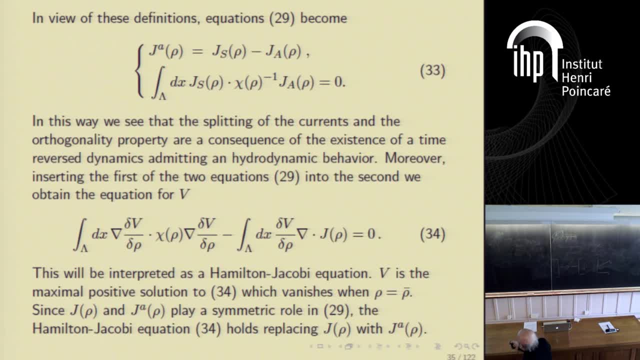 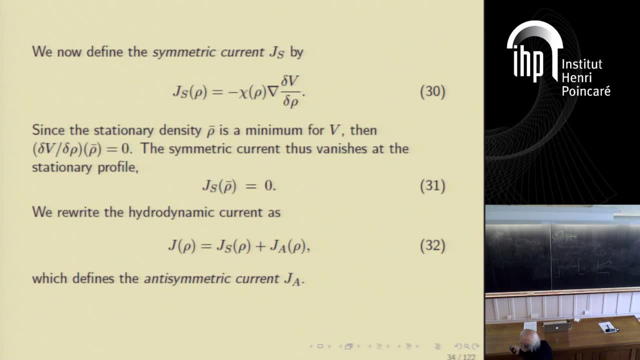 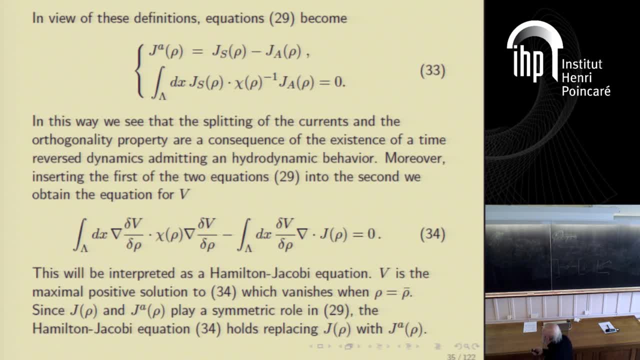 Then I will tell you what is the Hamiltonian corresponding to it And v. you can define this quasipotential as the maximal positive solution which vanishes for the quasi potential, the stationary profile. So then, I don't know whether I will discuss. 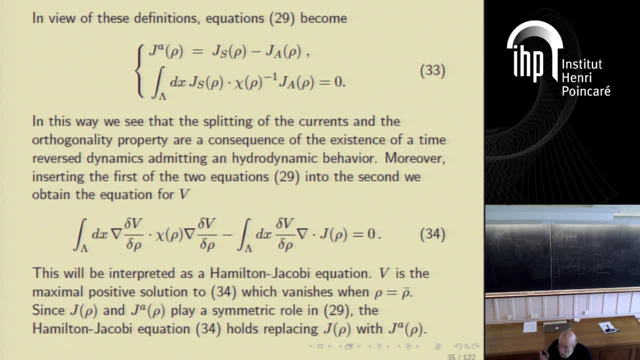 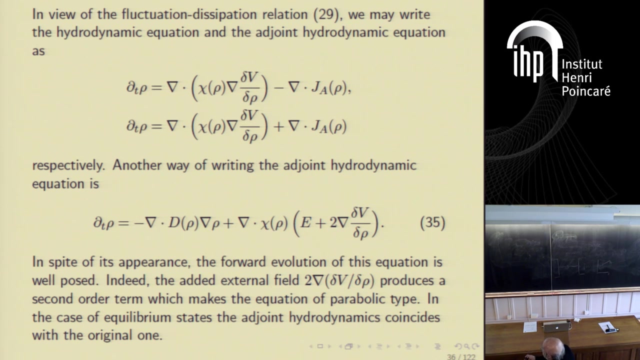 Maybe I will discuss it later. This is also a Lyapunov function for the hydrodynamics. This V is also a Lyapunov function for the hydrodynamics. Just by using this Hamilton-Yacobi equation. OK, in this way you see the hydrodynamic equations. 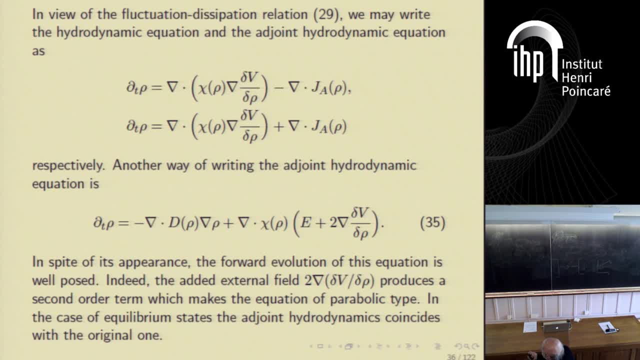 of the original process and of the time-reversed process are different. You can write them in a very simple way, because the dissipative- what I call dissipative- part is the same, And then there is this anti-symmetric part which changes sign. 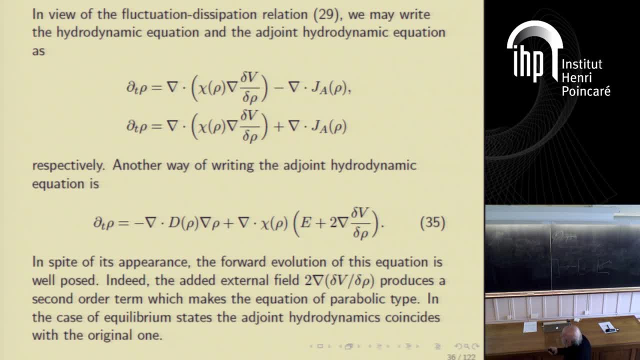 And here this term, here is this F field that I introduced a few slides before, which produces your fluctuation. So this is the hydrodynamics associated to the time-reversed process, And then you see that, in general, this is non-local. 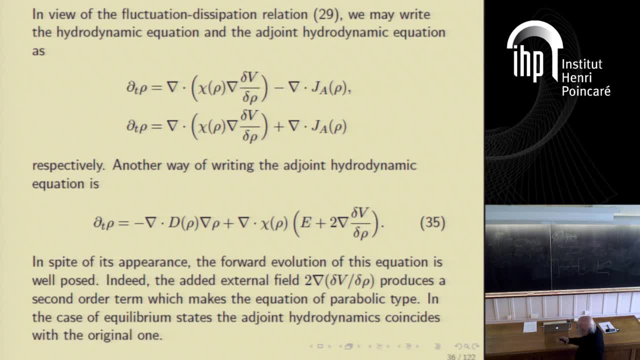 because this functional here is non-local, So it's considerably more complicated than So. you see, to reverse the process in general is not enough to add a field which is just a function of the point, But it's a field which is non-local, so it depends. 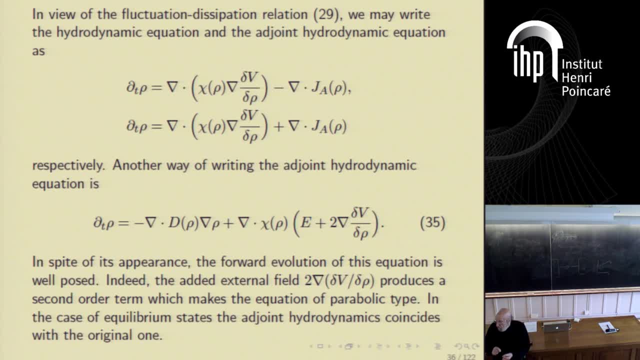 on the values of the density, The density everywhere on the system. So you have to act in a correlated way in the different points of the system. So I mean experimental is for the moment beyond, But in principle you can drive the system backwards. 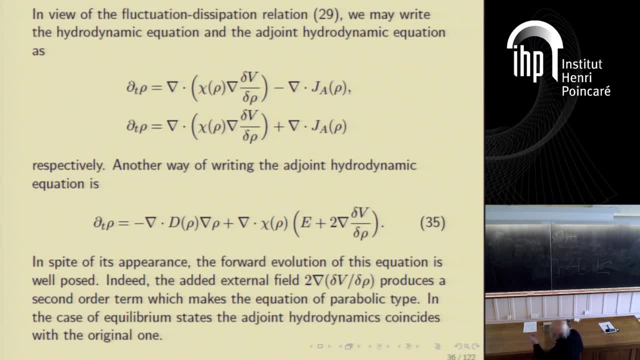 by using this field here. So you see that much information is contained in this V, which is called quasi-potential and which plays the role of the entropy out of equilibrium. In other contexts there may be different definitions of entropy, But in this context of large deviation this is OK. 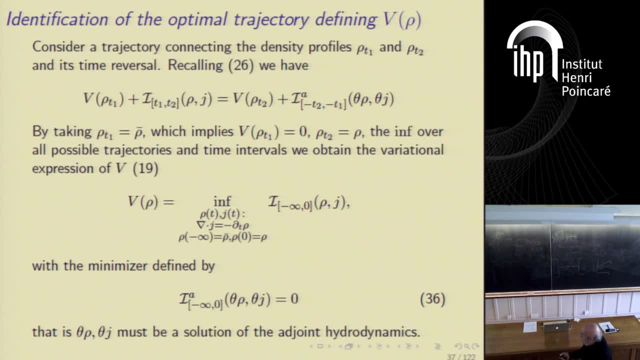 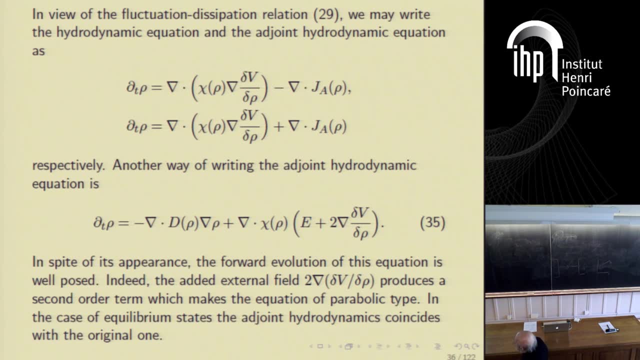 I have a question on your. I mean now, the dissipation has a wrong sign. Yes, Is this balanced somehow? or is that just the way? how it is? No, I mean, It's the long-time behavior of the solution. 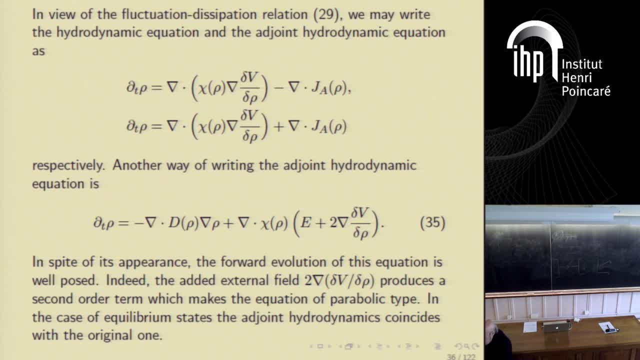 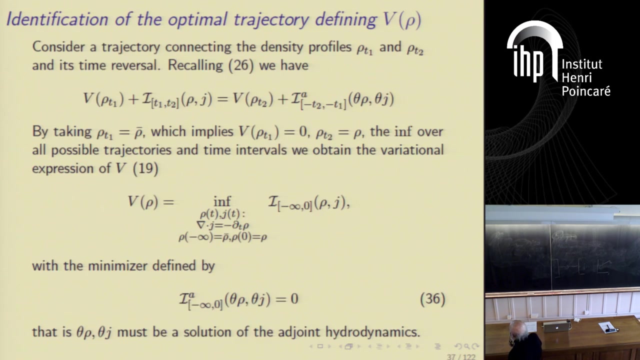 I mean, you see, it's like a particle in a magnetic field. You see, the term which changes sign is like a magnetic term under time reversal. So it gives you some rotation term. But I will show, maybe I have it. 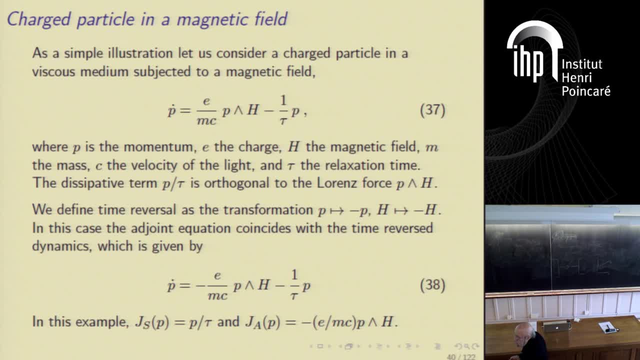 Remember, the other day I showed that this charged particle in a magnetic field. So But here the friction is the right sign. No, no, It's OK. You see that here the dissipative parts remains the same, And it is the Lorentz force term which changes sign. 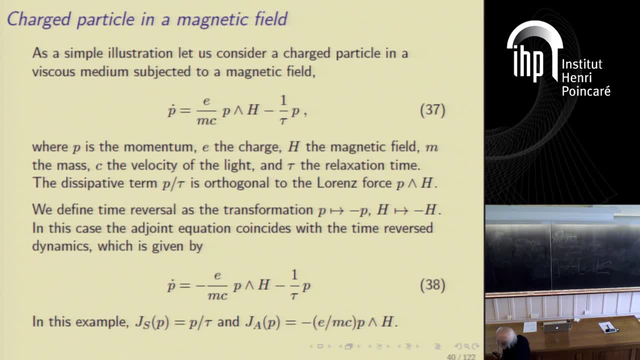 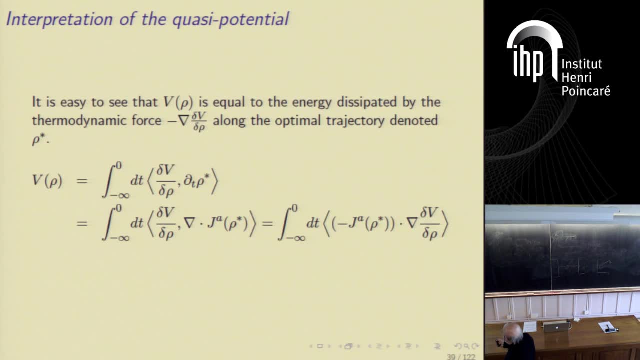 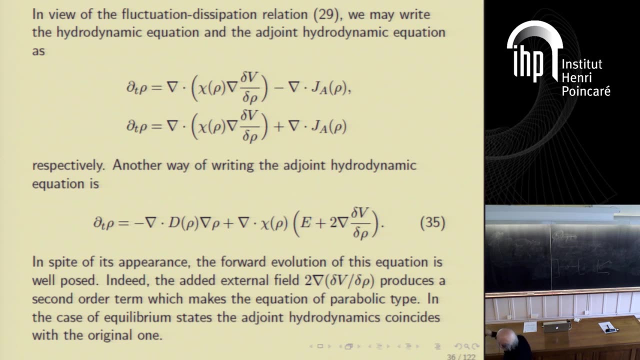 OK, So look at the other And you have the previous equation. The previous equation: No, no, no One for the Oh. You have the minus sign in front of the Oh. this one, Yeah, that's why I added this. 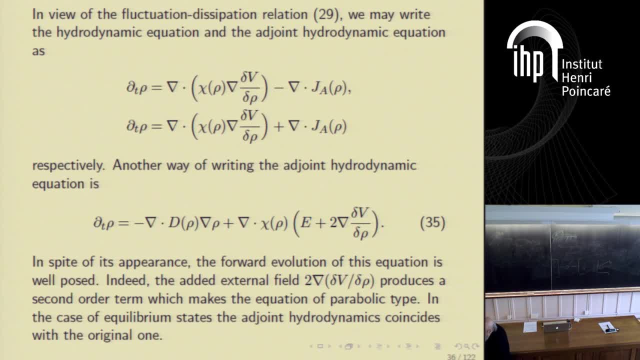 You said another. That was my question. But is there sort of another term which somehow? Yes, Then it re-establishes the correct sign. So it's well-posed. So the total diffusivity, the zero plus minus, zero plus zero is positive. 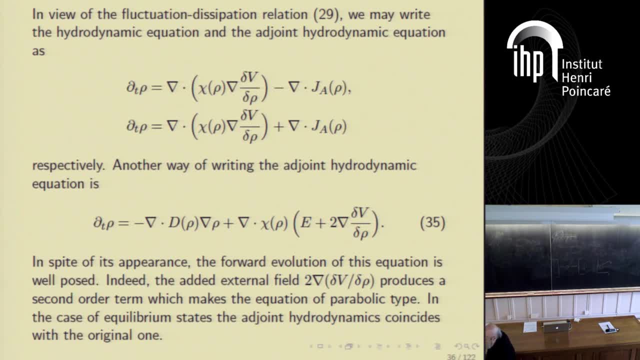 Again, In the end, the first term will have a positive sign. When you made explicit the derivatives which appear here, then you will get the term which is the same kind and which will re-establish the effect. This factor of 2 is helpful. 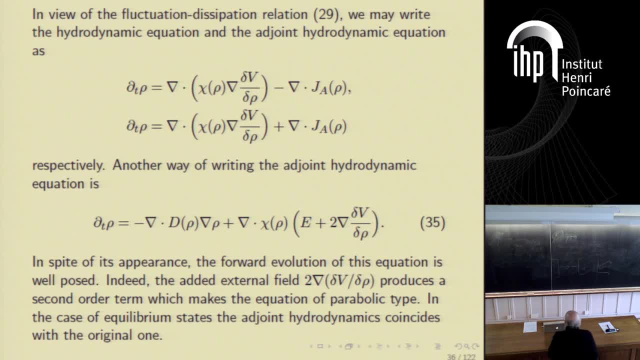 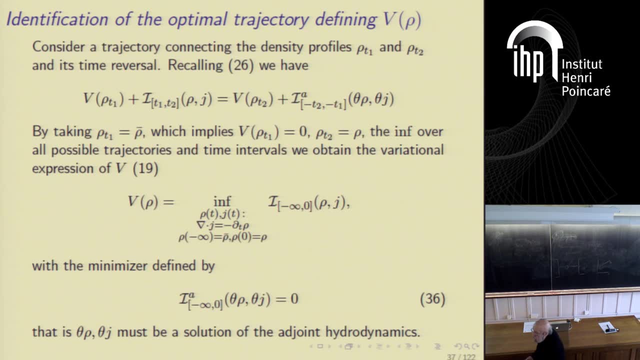 Helpful. OK, Now you can identify what is the optimal trajectory to create and to calculate. So you know what is the solution of the variational principle. And from this relationship here you start, Because you see you have to take the inf over all trajectories which start from the. 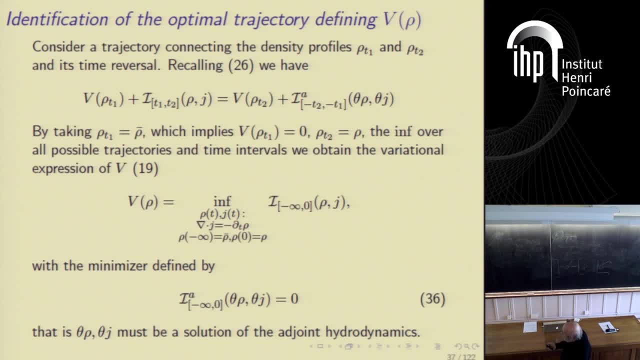 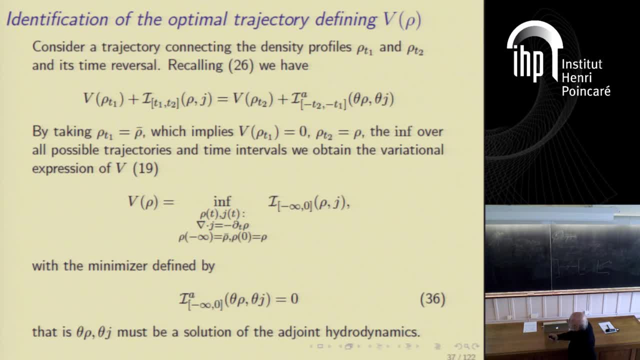 So this is on the stationary state. one of this term is zero. Then you see that if you minimize this object, this, you can do nothing, because So the best you can do is to make this quantity equal to zero equation. So what you have to do, you take the time-reversed. 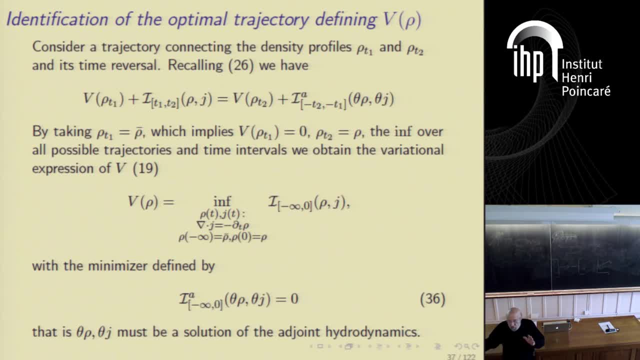 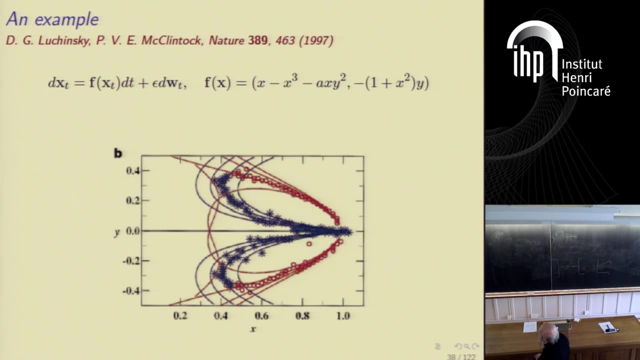 hydrodynamics. You can see the relaxation trajectory And then you go backward And this is the trajectory which creates the. I mean this is that I have shown. also the other day This very nice example was published in Nature by, and my clip doc. 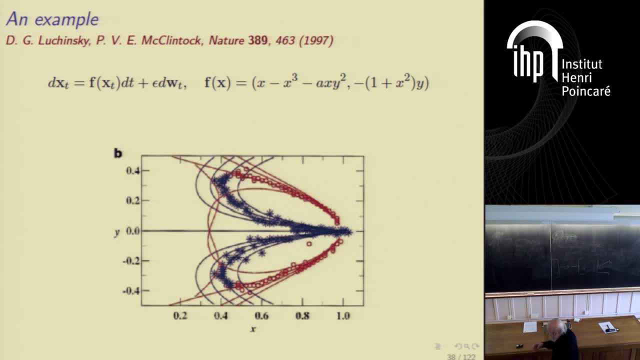 And it was made with the stochastic electron And it was an experiment made with stochastic electronic components. So they put the noise, which was small, but not too small, so they could wait for fluctuations, And the Langevin equation is non-gradient. 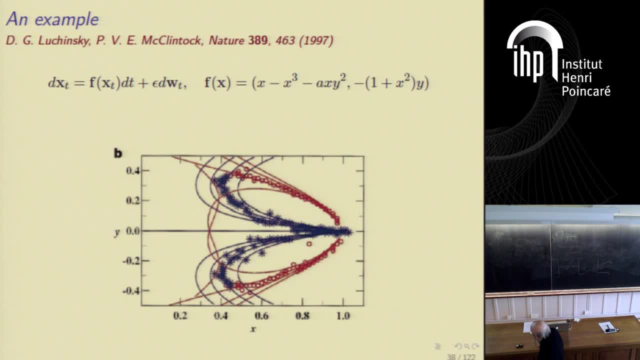 So it mimics a non-equilibrium situation. And then you see that you're, You have two types of trajectories. Now I don't remember which one is- the relaxation one and the fluctuation one, But you see, they were rather puzzled by the fact. 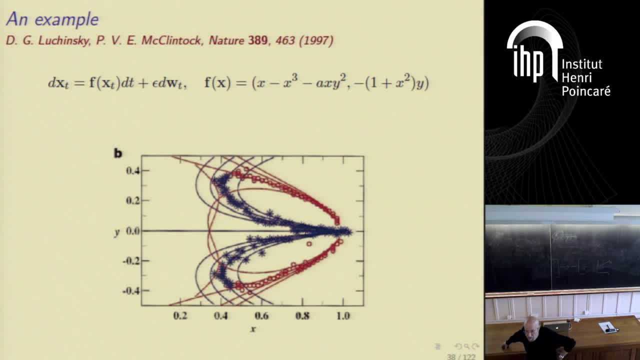 that they are different, Because in equilibrium, the trajectory which creates a fluctuation is just the time-reversed of the relaxation one. But as And then? somehow they did not, Then they did not, They did not have a general scheme. 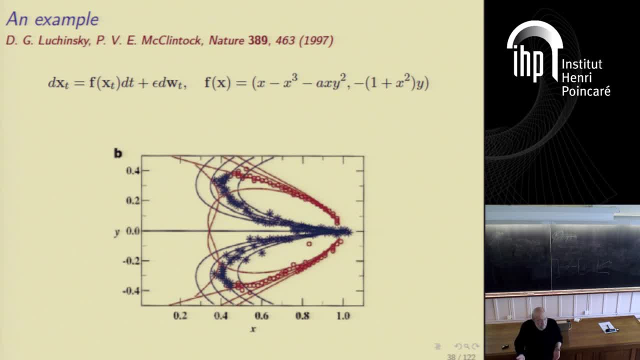 They did not have the notion of time-reversed diffusion, which exists in the mathematical literature. But if you do as we have done, defining the time-reversed process in the standard way and so on, then it's clear Because one trajectory is related. 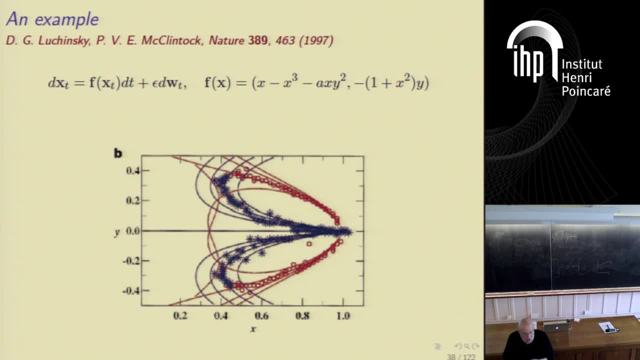 to the original hydrodynamics And the other trajectory is related to the time-reversed hydrodynamics. So there, They are different. Oh, these are No. no, I mean because this is symmetric in space. How does time flow in this picture? 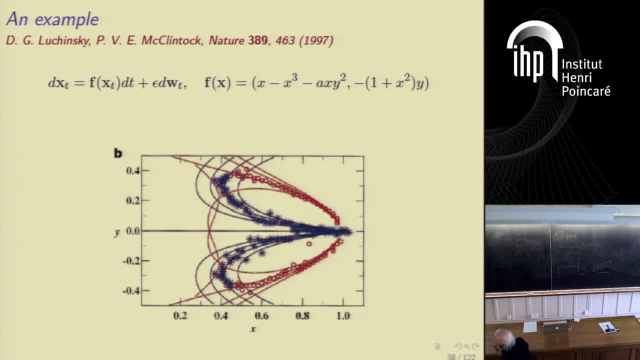 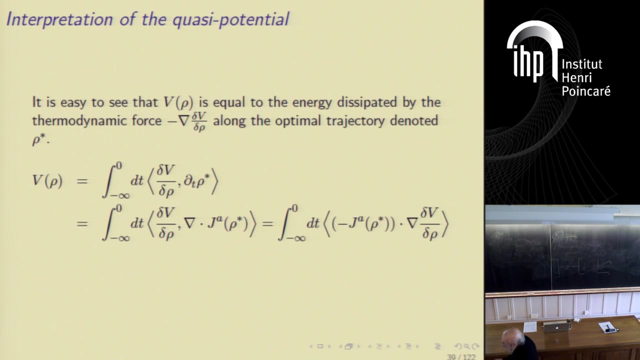 No, no, You don't see time. Time is eliminated. This is the equation in the xy plane. This is the equation in the xy plane of the orbit. OK, Now we shall discuss several interpretations of the quasi-potential. 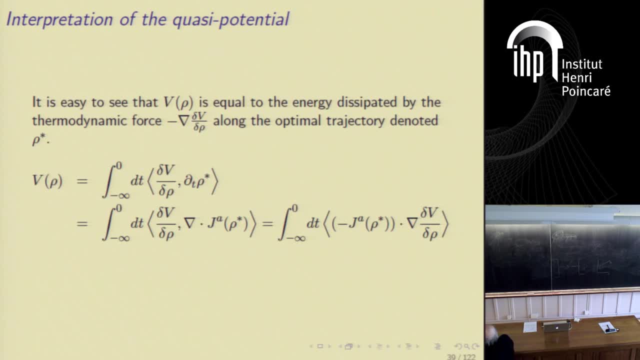 Well, also this one must be an A, Are we No Here? Yeah, Yeah, Yeah, Use the star for this optimal trajectory, But never mind. Anyway, if you calculate v on the, you calculate, I mean. 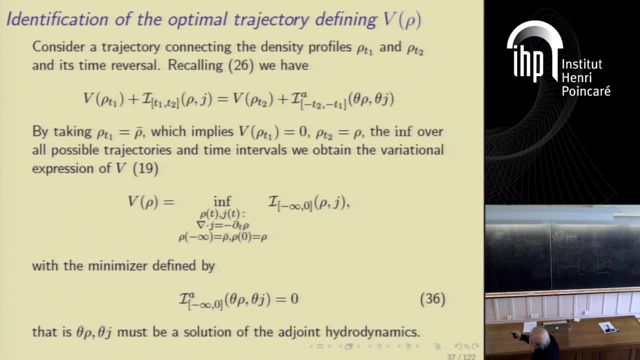 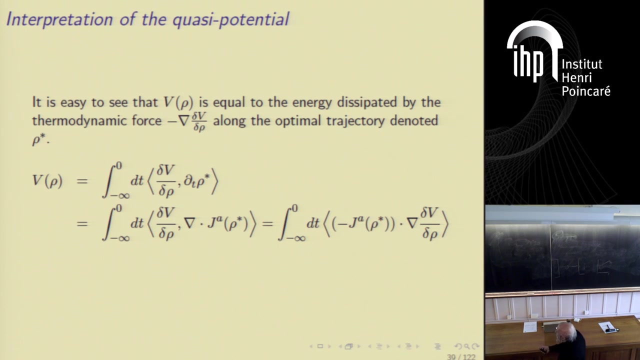 let's go back here. You calculate the, so here you have a variational principle. So you find an optimal, You find an optimal trajectory, And then you calculate all this on this optimal trajectory. Then you find the following: that in fact, this is just. 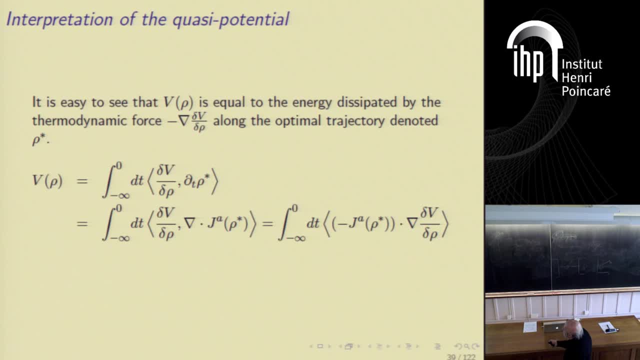 you make some integration by part. This is just the work done by the along that trajectory, by the, what they call the thermodynamic force, the gradient of the quasi-potential. So this is exactly this. Then I mean you can show that this is the meaning of the work. 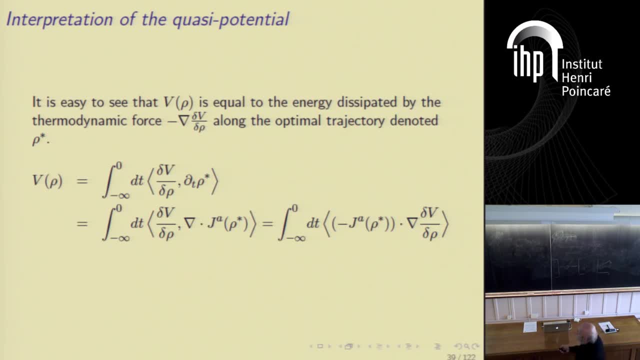 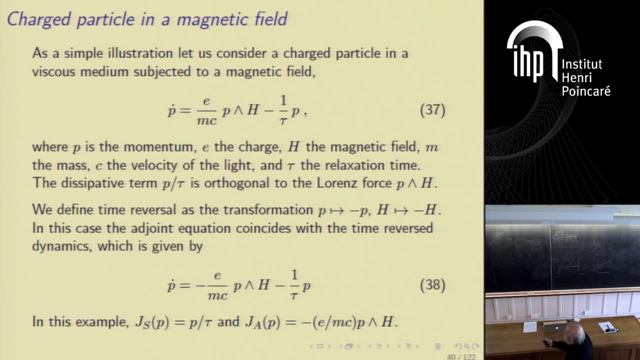 But this is quite clear from its definition. Now, these are the examples I gave also the other day. One is the particle in magnetic field, in which, that is quite strange, There is nothing magnetic in going out of equilibrium. But the new term. 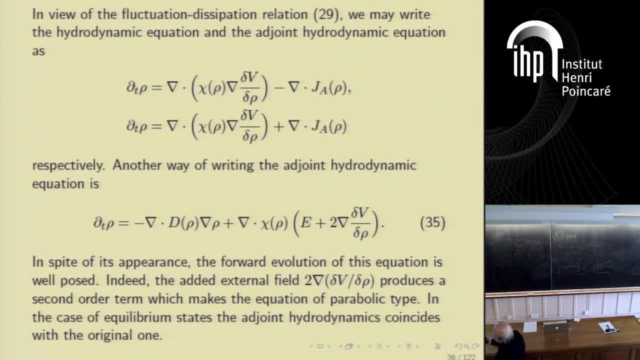 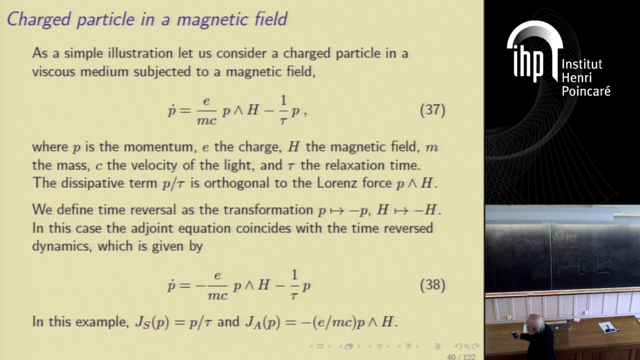 That you see this term and this J-I current is zero in equilibrium, So this doesn't exist. So you get only this term. But this is the term which behaves like a Lorentz force in the magnetic example. So it's like handing a term which behaves even if there is no but there. 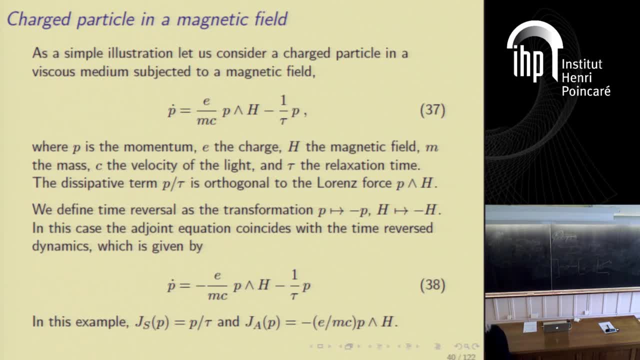 is a kind of duality, you see, I mean that's the way of putting it. It takes the whole effect. In the whole effect you put a magnetic field and then you get a potential difference. So you get the difference in the boundary conditions. 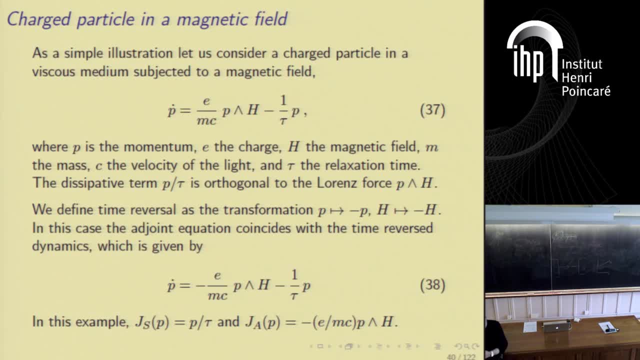 Here it's just the opposite. You put the boundary conditions and you get a field, an effective field which is under time reversal, behaves like a magnetic field. But the two things I mean physically are two very different situations. 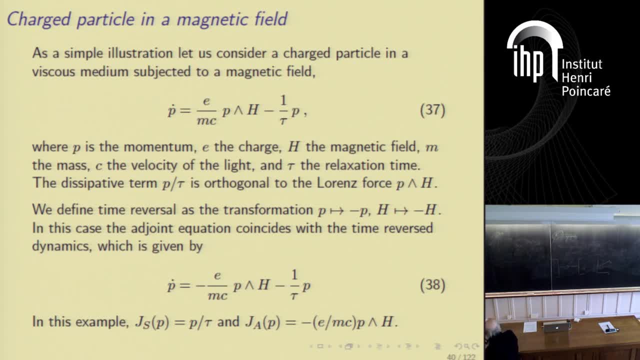 But the J-S is a part of the current that is dissipated inside the system and the J-A is what is actually. Yes, That's what it is. No, I mean, this one doesn't contribute to the dissipation. I would say. 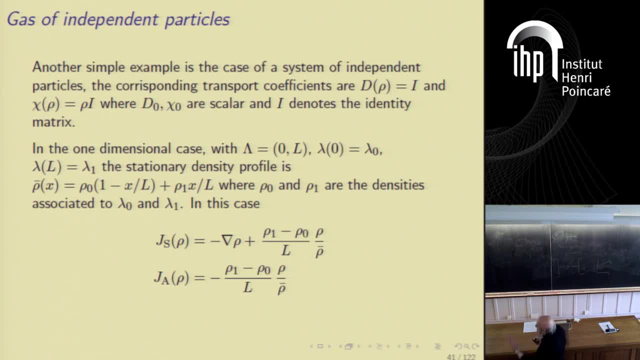 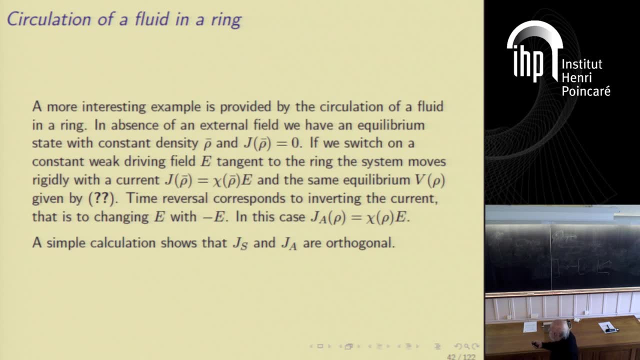 OK, then this is the other example of where everything is easy, because calculating the effective potential It doesn't present. And the third one is this circulation of a fluid in a ring, And it's very easy to calculate. the two currents are orthogonal. 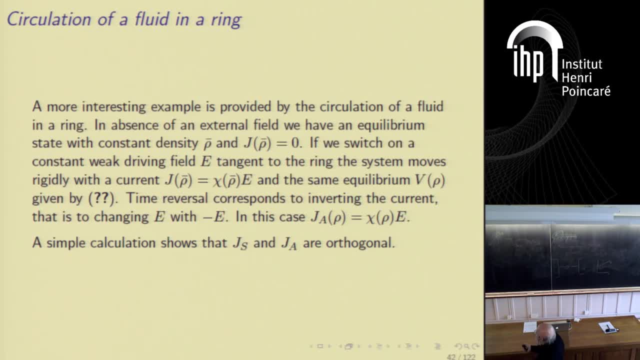 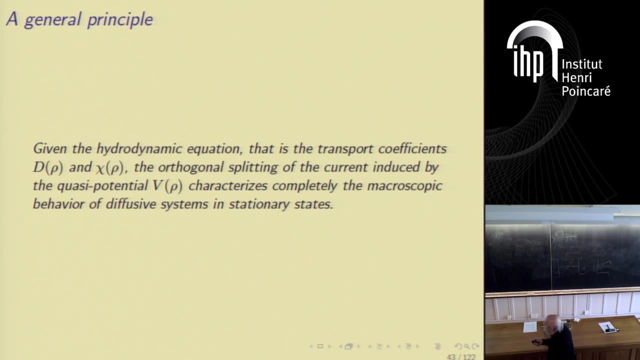 I mean it's: Oh, I should have eliminated this, which was there also the other day, but I forgot. OK, OK, OK, OK, OK, OK. So I mean this seems to be a general phenomenon, this splitting of the currents into two parts, which 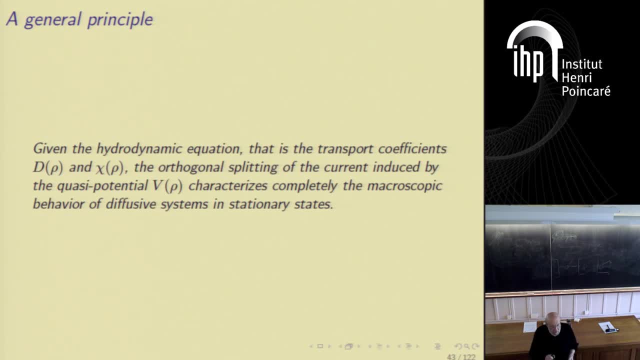 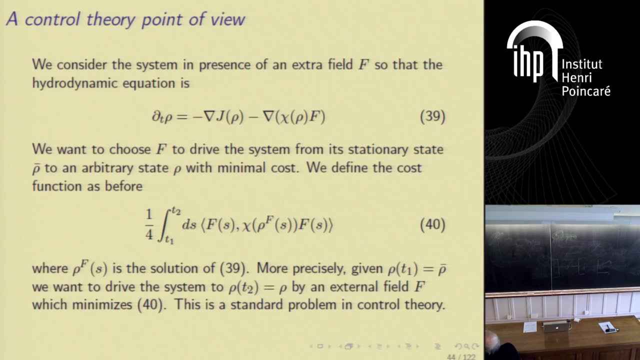 are orthogonal to each other and are characterized by having opposite transformation properties. on the time reversal, Maybe I can give you another point of view on all we have said. OK, OK, OK, But then maybe we stop After one hour and a half. I think it's enough. 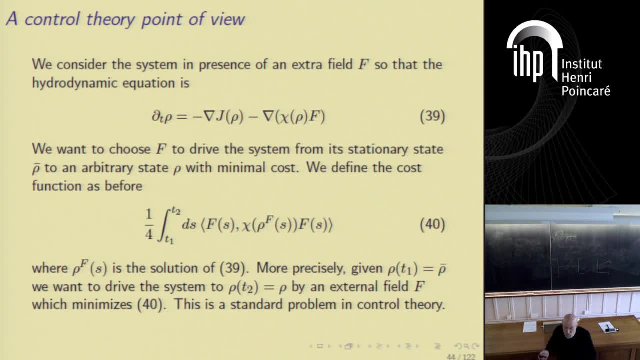 Or maybe I can keep it for tomorrow. If you are tired, we stop here. We have seen a long program to do in the next two And I will not be able to exhaust everything, OK. So anyway, if you want to ask a question, 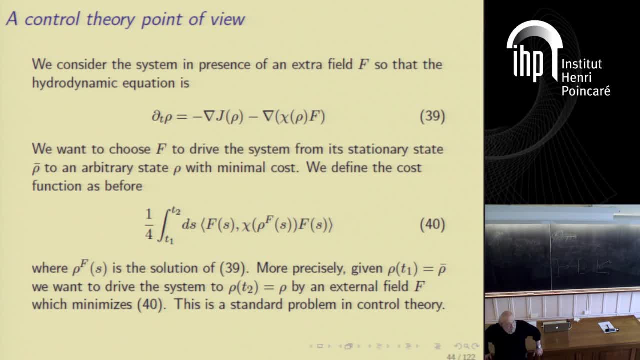 I'm happy to answer if I know the answer. I'm not very clear about the joint process and reversal process. Well, it's a standard definition in the theory of Markov processes, Absolutely standard. That's the way you'd Suppose you want to realize. 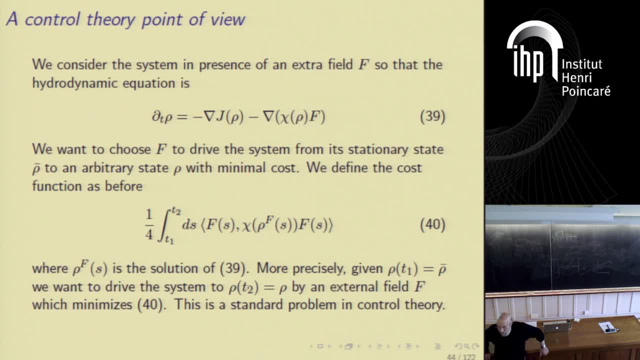 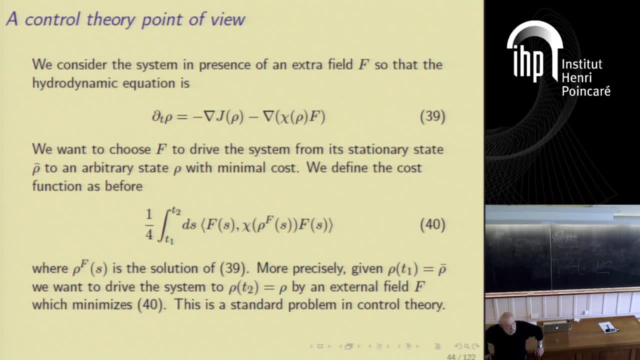 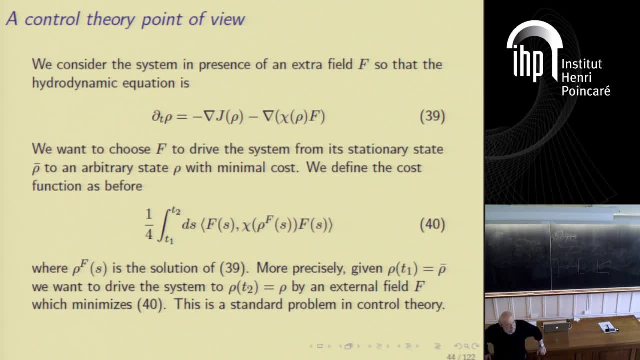 the trajectory of the time reversal process. But we certainly modified Mm-hmm. But the past probability for the reverse trajectory is equivalent to the forward trajectory. No, I mean the scheme is consistent. The optimal trajectory is different from the trajectory of the original process. 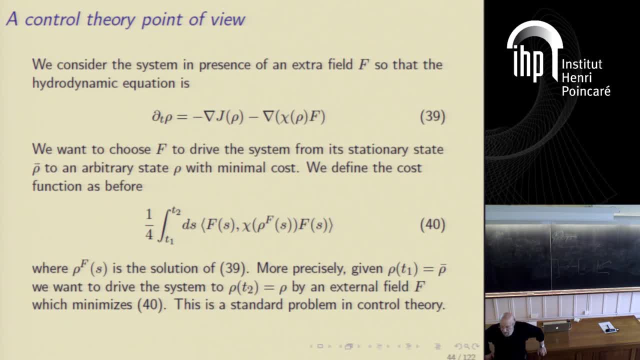 It's associated with the time-reversed process And, if you want, they have a way to simulate it. Well, so far, what I've discussed so far it's with the boundary conditions and fields which do not depend on time. But when I will discuss thermodynamic transformations, I'd have to introduce time, because otherwise, 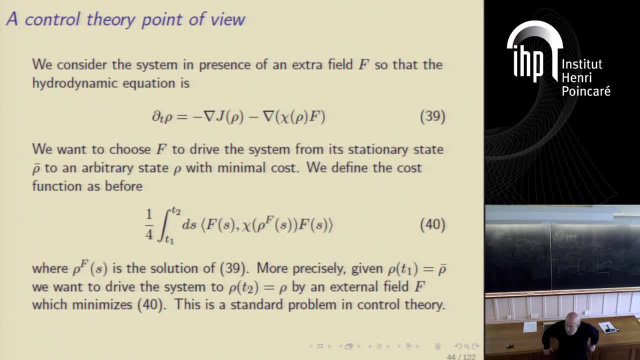 nothing changes. Yes, Sir, if I take the step with boundary conditions, forward dynamics, I know that you know the particles are jumping. I put something in the background, I look at it, The time-reversed process. I mean, I'm not sure how well you actually know how particles 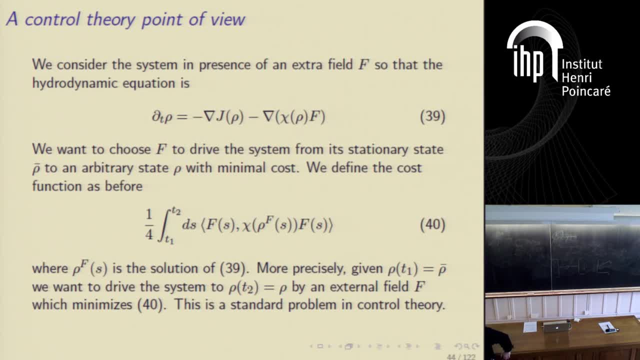 are jumping on the time-reversed process. Well, you, I mean you have to first give a rule, You, just if you have a time dependence for the boundary conditions. No, no, Let's just fix boundary conditions, Yeah. 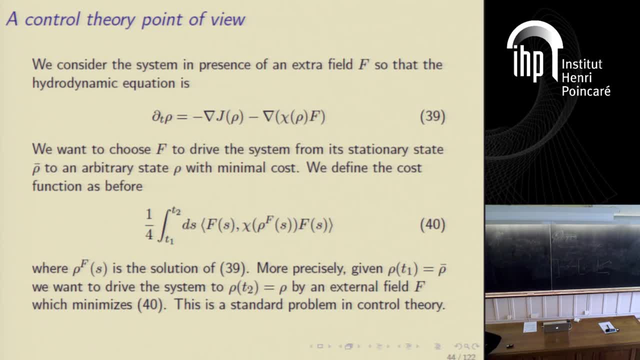 No external fields, Just fix boundary conditions. Yeah, I have inside the 7. From outside I fill in the particles and get them out. And now I look at the time-reversed process. I mean, can you say what the individual particles, how they are jumping? 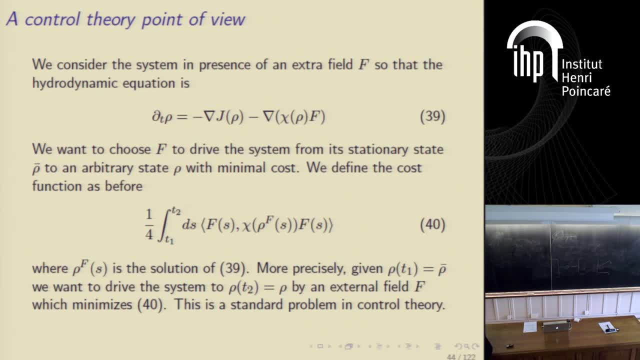 Well, they will jump. I mean, the boundary conditions are the same. Yeah, So the microscopic time-reversed process is well-defined. It's defined by How do particles jump? How do particles jump? It's well-defined, I mean. 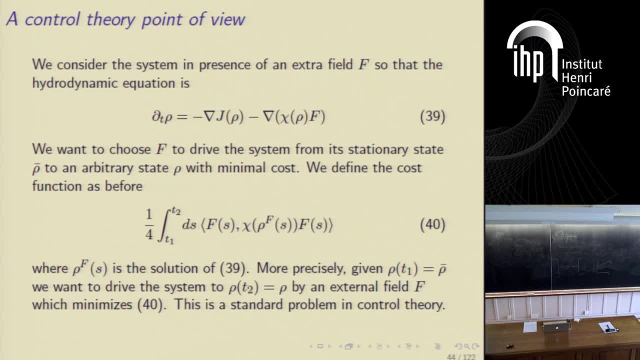 Not even Markov process. No, it is Markov process. No, no, It is Markov, It is Markov. But how do they jump? You see, you know the generator? Yeah, But you know the generator, which is the adjoint with respect to the invariant measure. 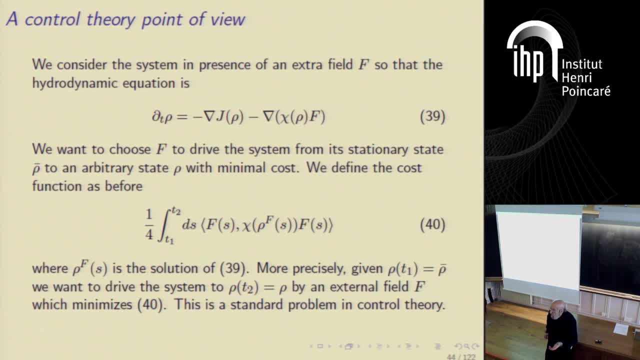 Yeah. Do you even know the invariant measure explicitly? No, You don't know it explicitly. Okay, But I mean, in principle you know everything, Because if you know the invariant measure, you know, And the generator of the time-reversed microscopic process is just the adjoint. 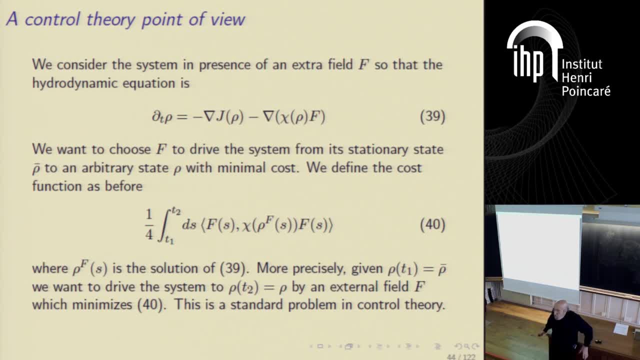 Yeah, With respect to the invariant measure. So I mean Yeah, But I mean, for instance, if I do this, If you, Then practically it's another question. So you are doing the diversion. That's why you know it's Markov. 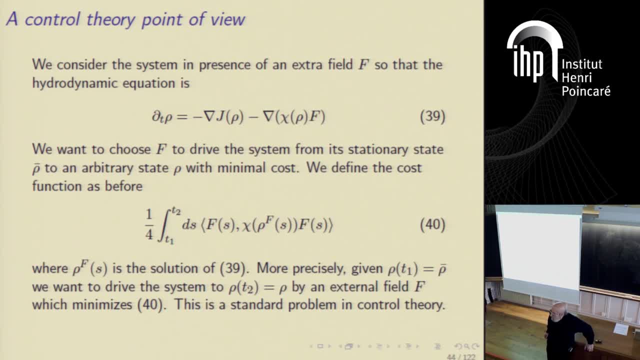 But that's it, That's it, That's fine. I mean so in the forward. I know that you know the particle jumps. It just has to know whether the side which is next to it, whether it's actually empty. 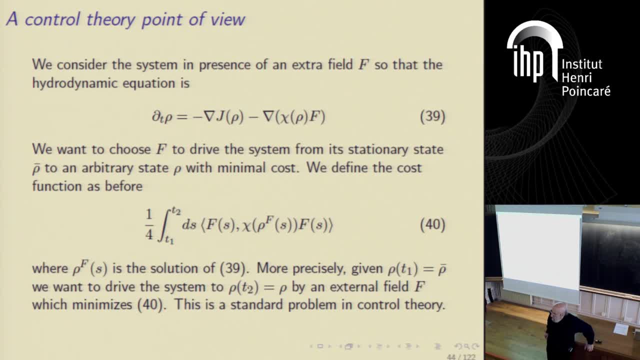 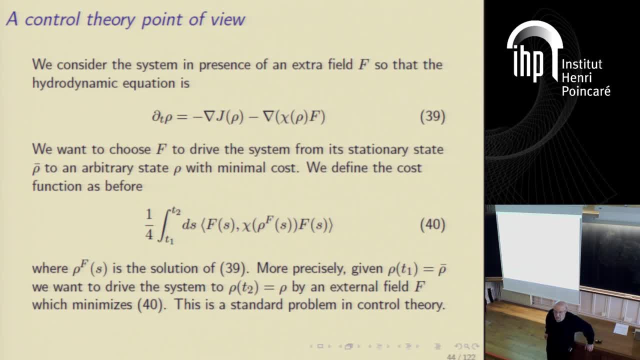 Yeah, Yeah. So when you're talking about cross-examination, is it probably complicated in which you don't know? Not, It's a non-local. It's a non-local, This non-local for the hydrodynamics, but at the microscopic. 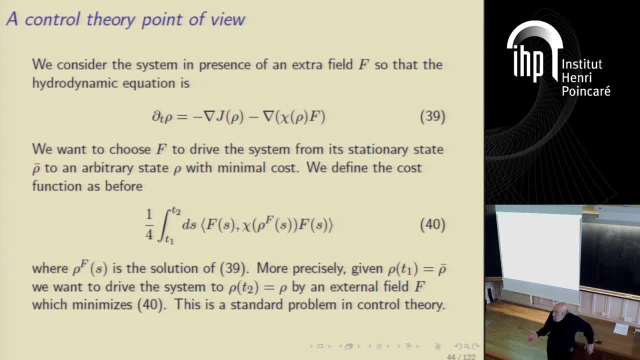 What is the general At the microscopic level, once you have the generator? Well, it will depend on the whole configuration, Presumably Yes. Presumably yes because it's a joint with respect to the It's from the invariant measure, where you get sort of all the. 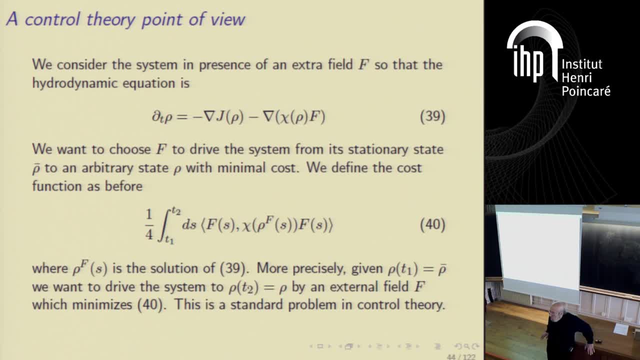 OK, Yeah, I don't claim that it is simple, but the conceptual is well defined. Conceptual is well defined. I mean, I think every theory has its limits in what you can practically do with it. And I mean the lucky thing is that with this approach, 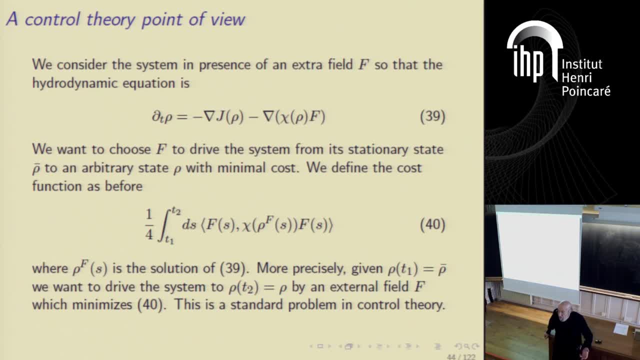 there are many concrete problems which have been solved, but I don't claim that you can solve all the problems with this. I mean, that's clear. No, no, what you say is absolutely correct. I mean, after all, we all have learned on your book how to deal with this problem. 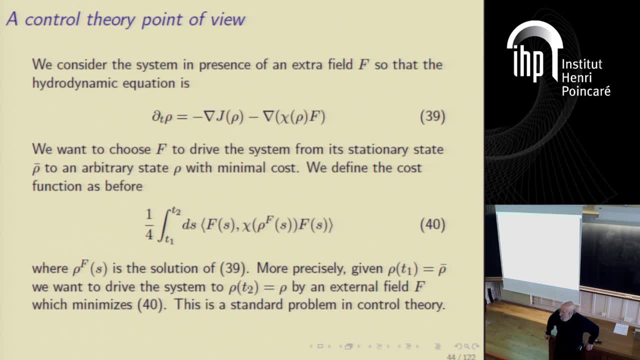 In a context of what you call current. this is what we call current, with some kind of energy or flux of energy, what you call energy work. No, why? why? I mean in this system, if you take it in terms of particles. 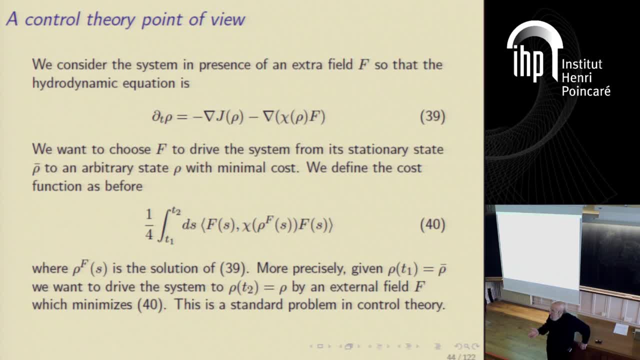 I mean, the only conservation is the number of particles. Yes, yes, I mean the yeah So there is in the stationary state, there is a clearing. what is the current of the Yeah so? But this is not the J. 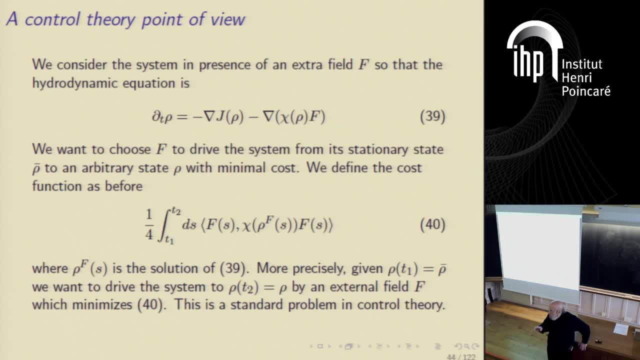 Well, you have the J of rho, which is something which is the macroscopic constitutive equation, But when you No, I take the stationary state. Yeah, The stationary state. there is a curve. Yes, Now I. 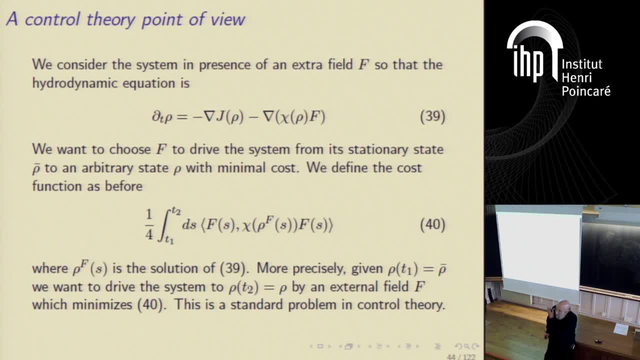 The current has a complicated expression because, as I emphasized, it is non-local. in space It's a function of the density, but non-local. So it depends on the values of the density of all over the system. Yes, What is the interpretation of the symmetric 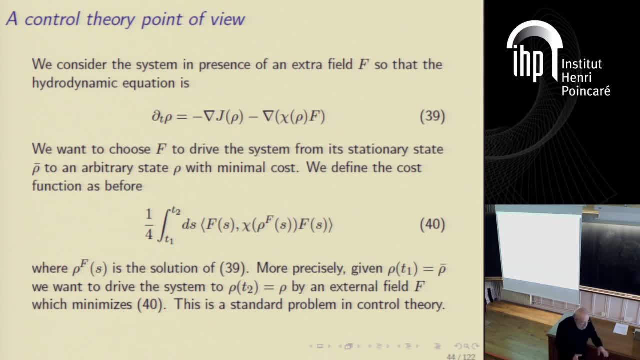 Well, I mean the. They are clearly. The interpretation is quite clear in the in the extreme cases. So, if we are in a stationary state, there is only the J current, which, And so with this J current, you may calculate how much energy you have to dissipate. 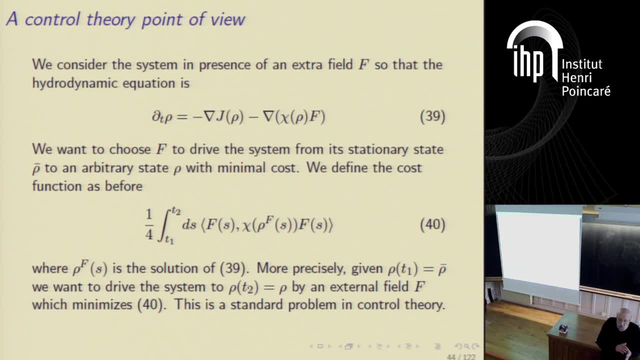 to maintain it. In the opposite case, in which you have, For example, the system is in equilibrium and you have a fluctuation of density and the system relaxes To equilibrium, Then you have only the J current, But then in the general case, 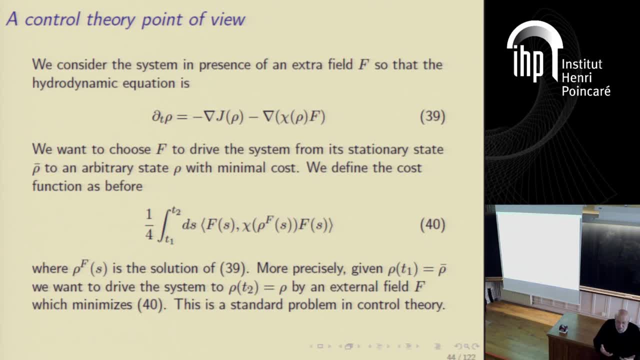 somehow the, The interpretation is mixed, because You cannot separate so clearly The fact that they are always orthogonal. Well, that is. Well, that is a theory in this scheme. I mean, We have to come back to this type of questions. 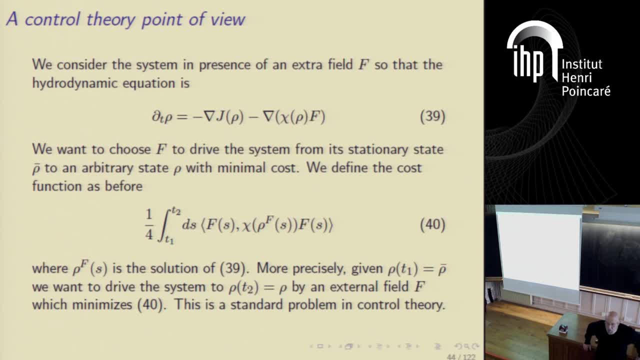 because I mean the. I mean the operational interpretation of this scheme is not simple, but I think that I mean as long as the thing develops, one has to go on. We look backward and see whether what we have done is sensible or not. 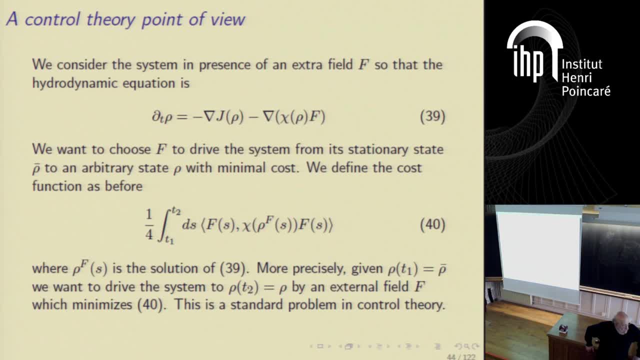 So tomorrow at 2 o'clock And then I think it's on Thursday. Yes, Uh, So we still have time. 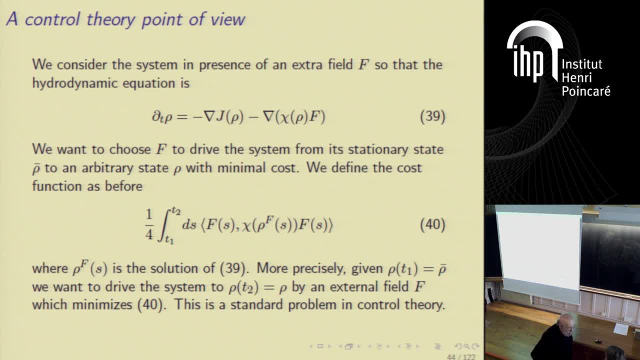